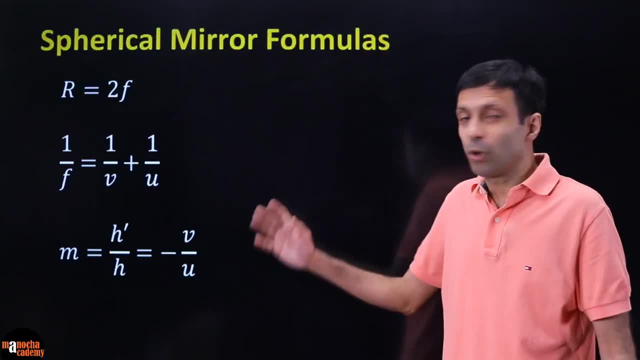 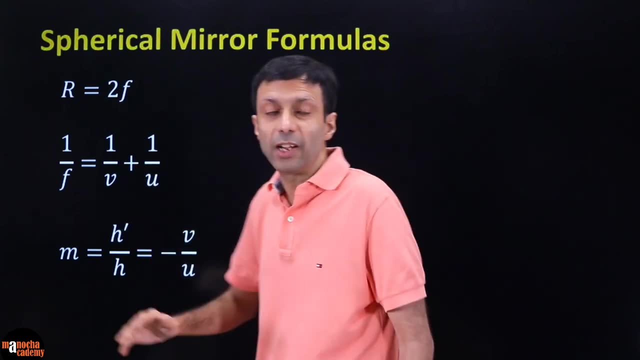 So guys stay connected, keep learning. So please watch the video for the details. but I'm going to do a recap on the spherical mirror formulas. What do we mean by spherical mirrors? Spherical mirrors means curved mirrors. There are two types of spherical mirrors: concave and convex mirrors. 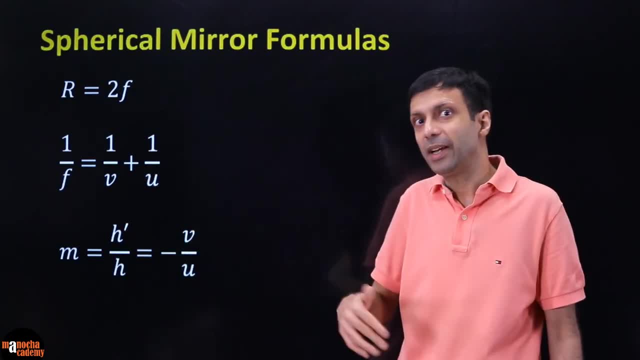 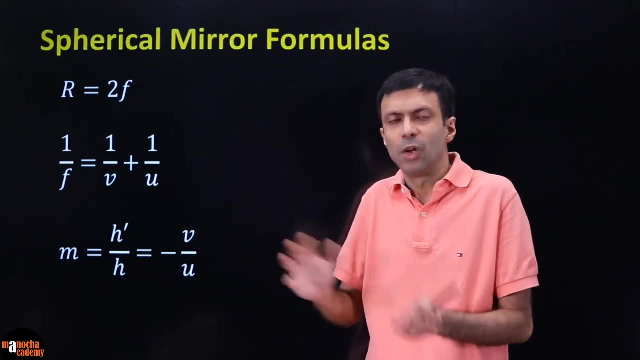 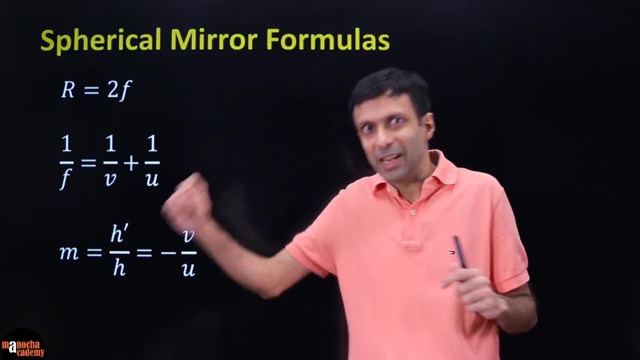 And these formulas can be used to predict if you place an object you know, at a certain distance, in front of a spherical mirror, concave or convex, with a certain focal length. Using these formulas, we can predict where the image will be formed without drawing the raised diagram. 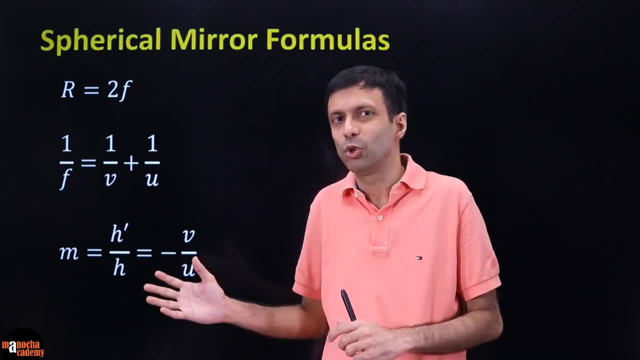 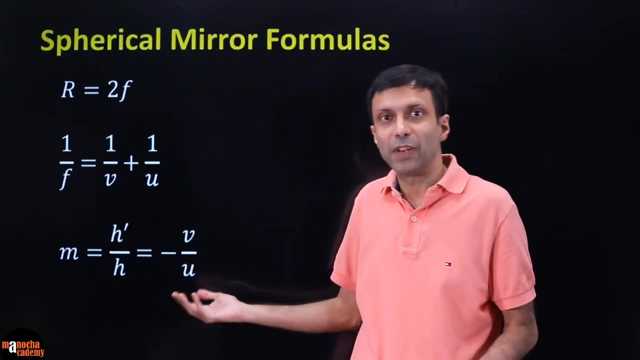 It's important to draw a rough diagram to visualize it, Okay, Which I'll show you. But you don't have to draw all the rays, You can just predict it using this formula, or what will be the magnification? we can find that out. 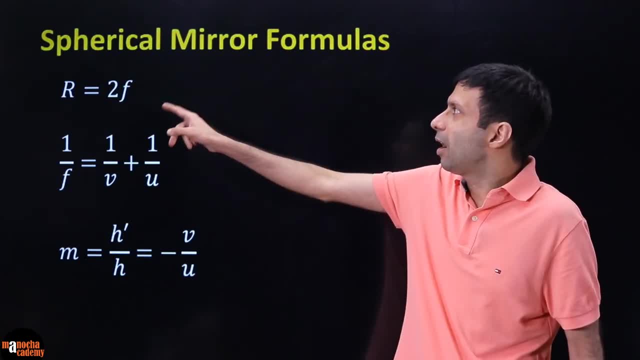 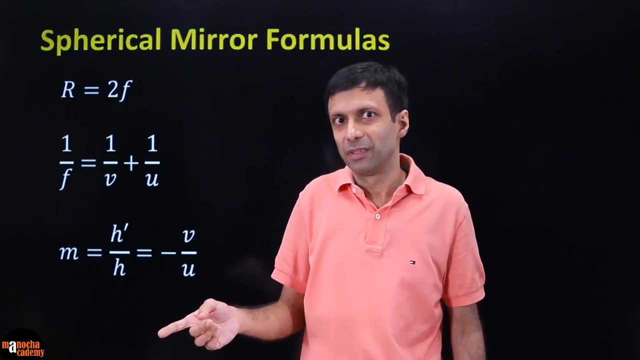 Okay, So what do these formulas mean? The first formula: R equal to 2F. What does this capital R stand for? Capital R is the radius of curvature. Right Radius of curvature means spherical mirror, is a curved mirror. So what is that radius of curvature? 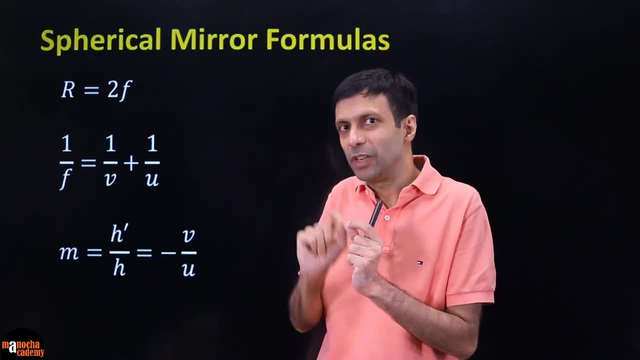 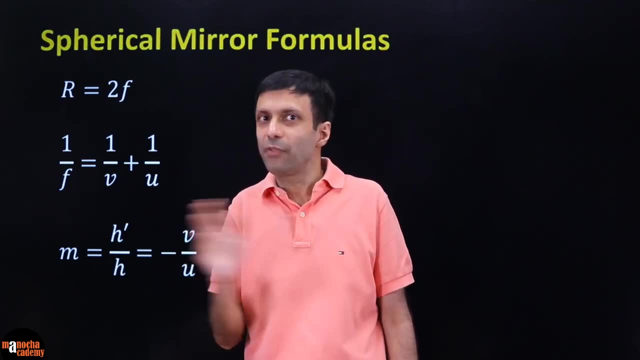 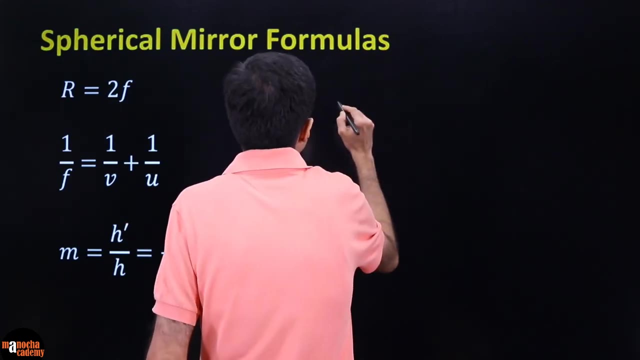 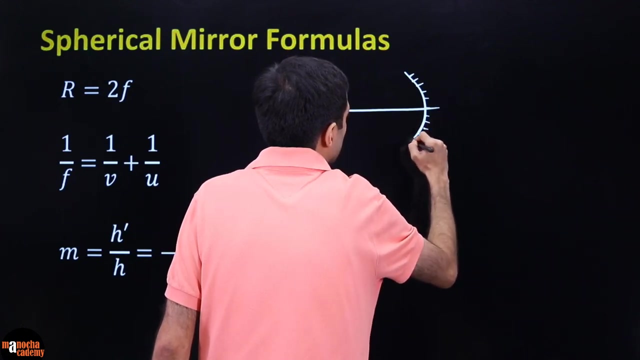 That means the distance from the center of curvature To the pole. That is basically twice the focal length, Because we know that focus is halfway Right. It is exactly at the midpoint of the pole and the center of curvature. So if you look at the principal axis, 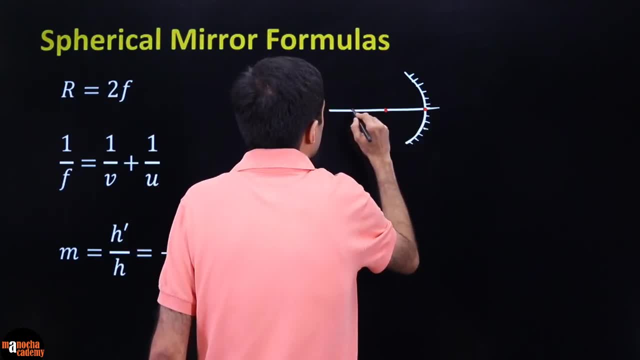 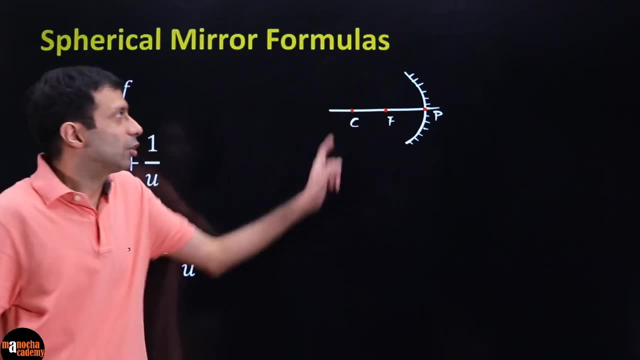 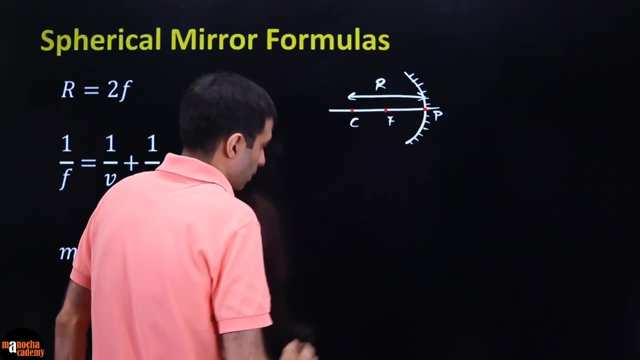 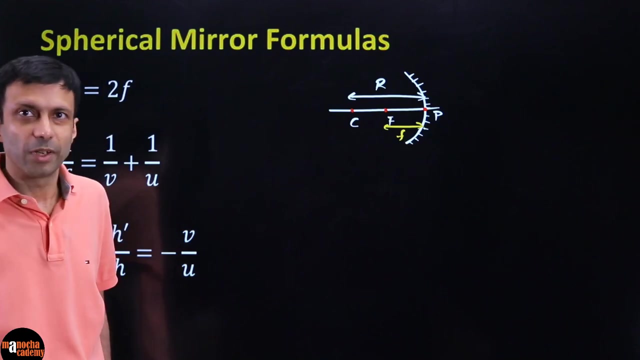 For, let's say, a concave mirror, We have the pole, the focus and the center of curvature. Radius of curvature means P to C. This distance, And this is the focal length, Distance from pole to focus, And what is the relation? 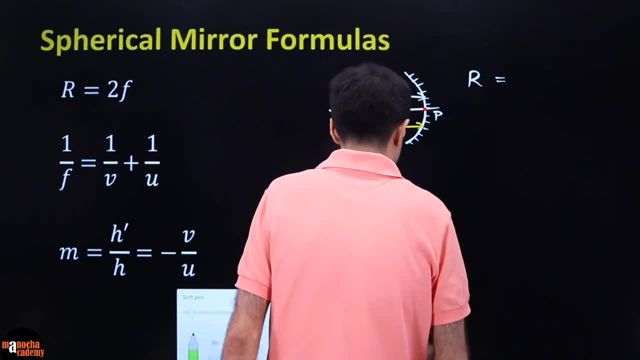 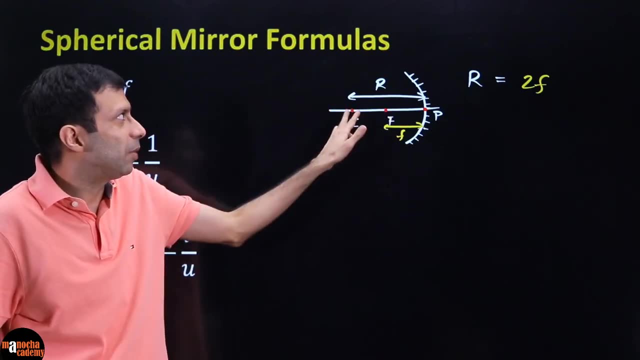 R equals twice the focal length, Because you can see that focus is exactly in the midpoint. Like I told you, If this is 3 cm, this should be 3 cm. So total radius of curvature is 6 cm And focus is exactly in the middle. 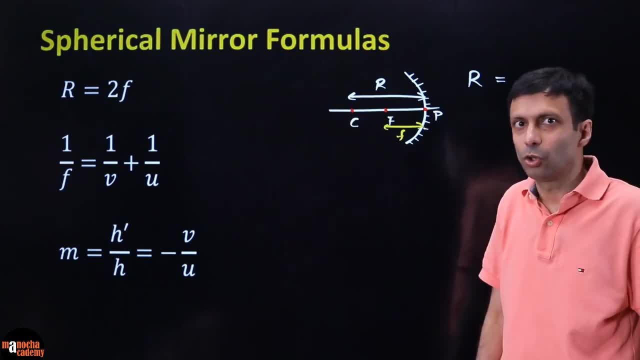 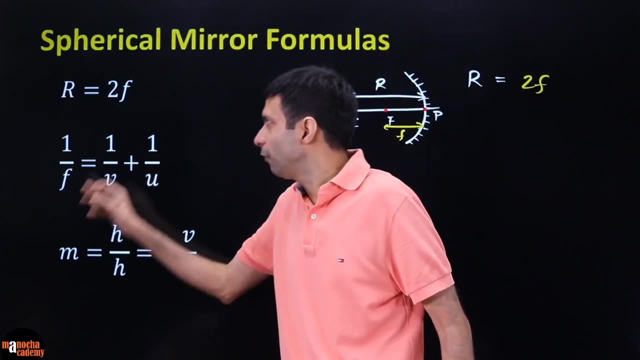 Next formula? So that is the simple relation: R equal to 2F, or focal length is half the radius of curvature. Now what is the next formula? This is very important: 1 by F, equal to 1 by V plus 1 by U. 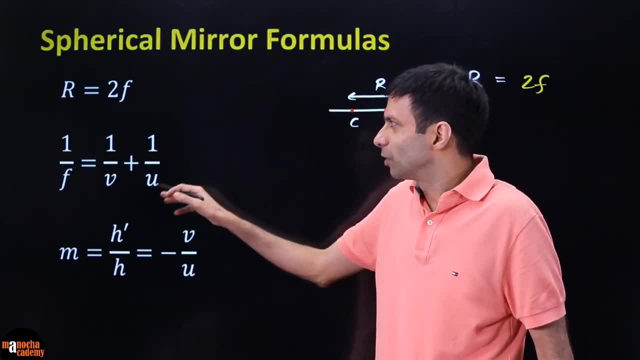 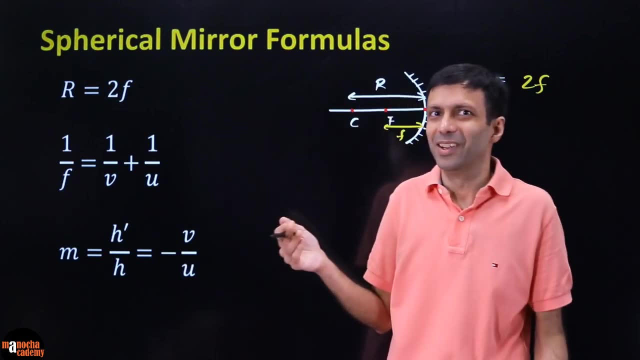 So it is very important to understand what are these terms. U and V is not initial velocity, final velocity. What do they mean here? So in this chapter they mean different things. In Newton's laws of motion or equations of motion, This is our initial and final velocity. 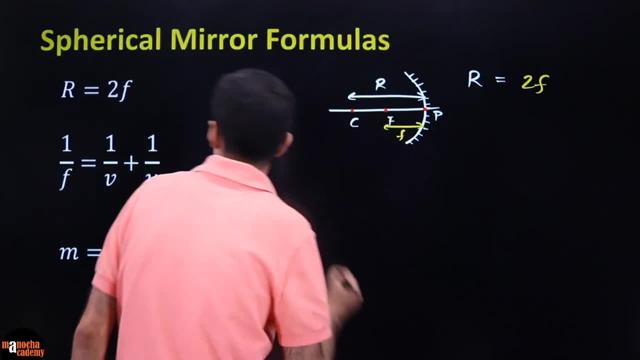 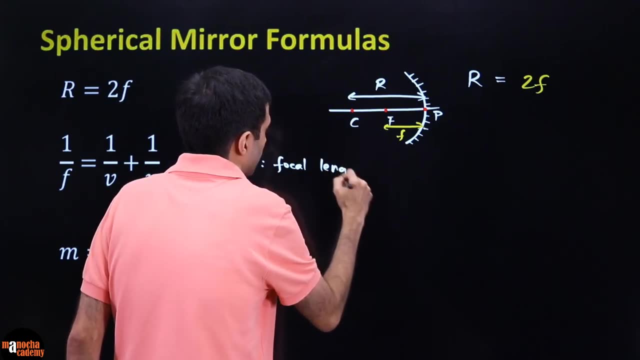 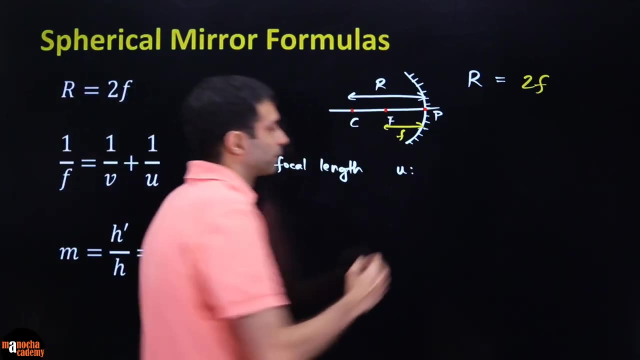 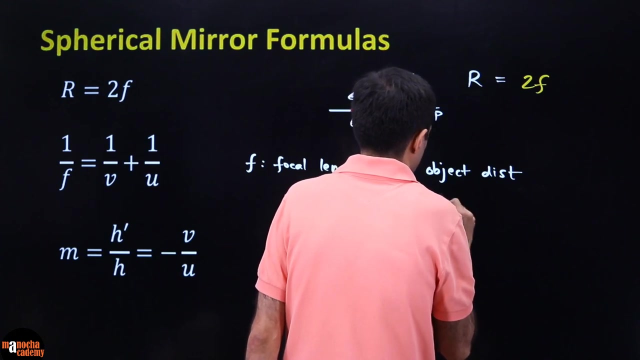 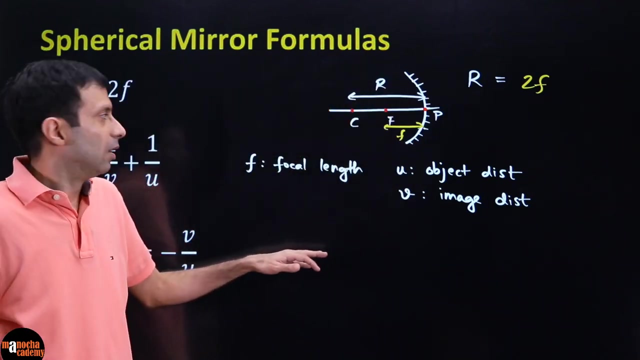 So what do we have here? Here, F stands for F is the focal length. What does U stand for? U is the object distance And V is the image distance. Now, all these distances, where are they measured from? One very important thing: 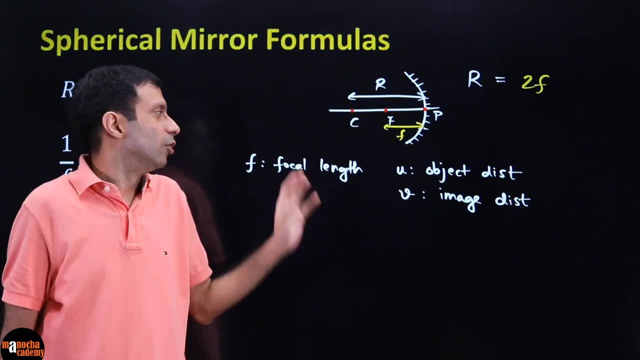 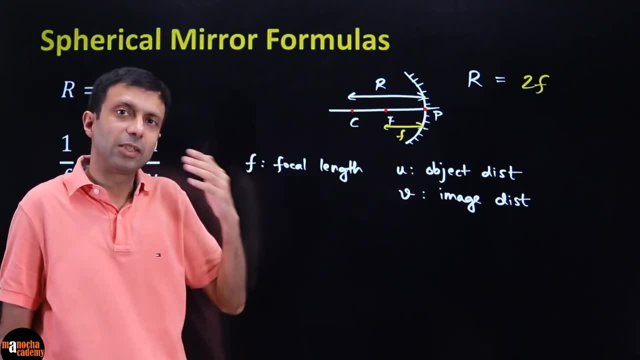 They are always measured from the pole Which is the center of the mirror. So focal length, just like distance from pole to focus, Object distance, distance from pole to the object, Image distance, pole to the image. So please keep that in mind. 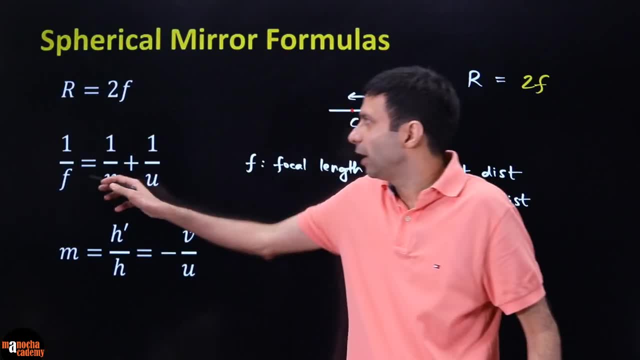 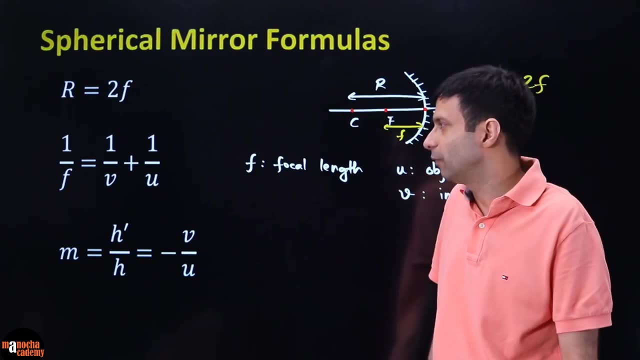 And how are these guys connected? So these reciprocals, It is not F equal to V plus U, Reciprocal of focal length. So 1 by F equals 1 by V plus 1 by U. Very important, And this is how you use the formula. 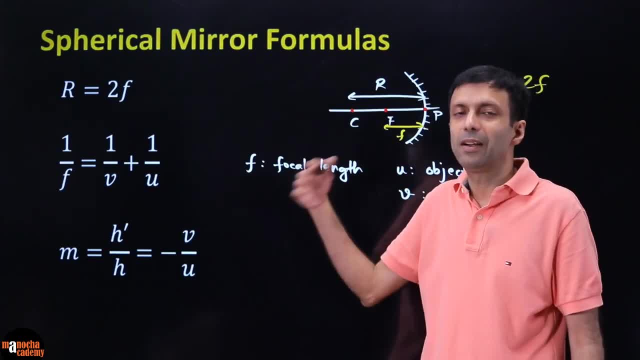 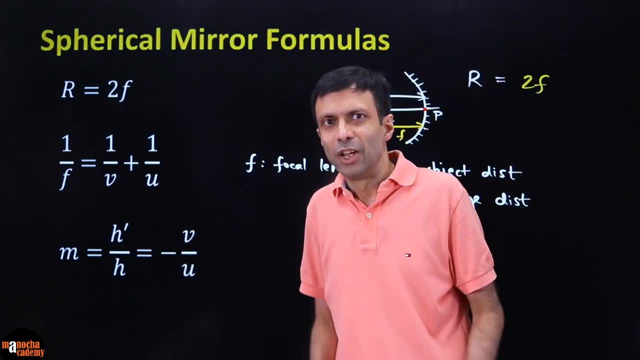 Derivation of this formula is not required. We just need to know the formula and how to apply it. So, for example, if focal length and object distance are known, We can find the image distance. So, given two things, just like we solve a maths equation. 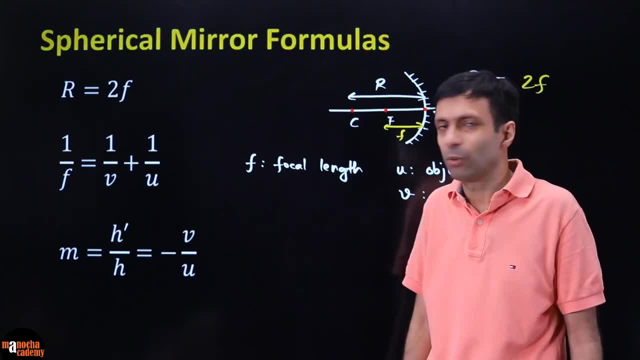 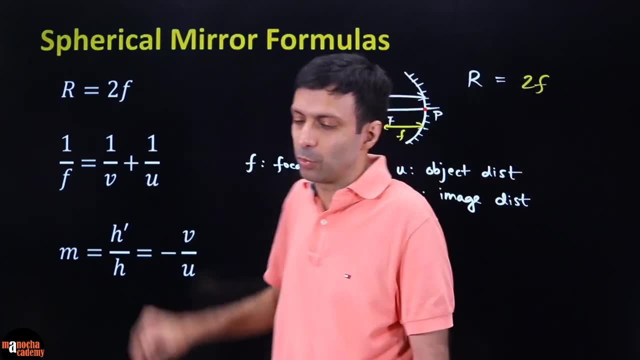 You can find the third guy. If you know two things, you can solve this equation and find it Simple. And then the next formula. So this formula is known as the mirror formula, This famous one which connects focal length, object distance and image distance. 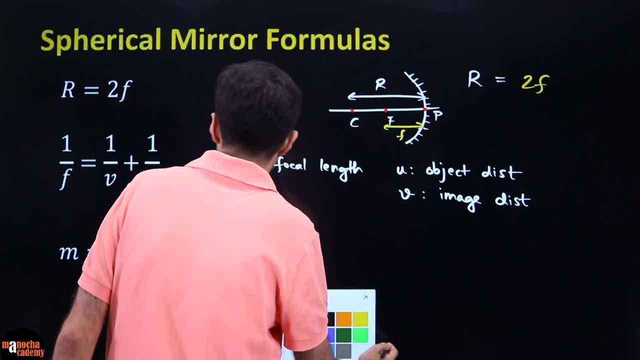 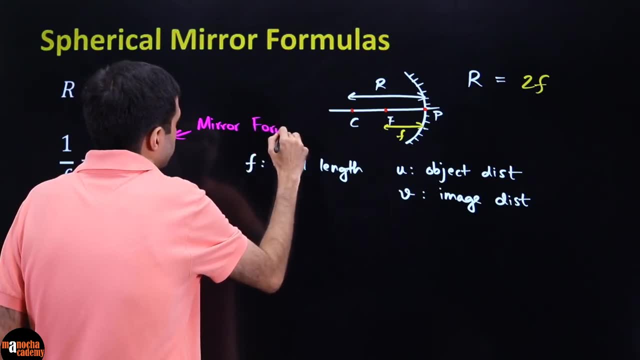 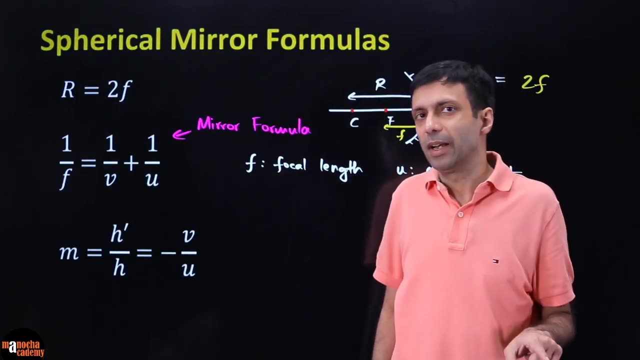 This is called our mirror formula. So let us write this down. This is the mirror formula. When you guys do the lenses chapter, It will be called lens formula And you guys know it will look very similar. But there is one important difference. 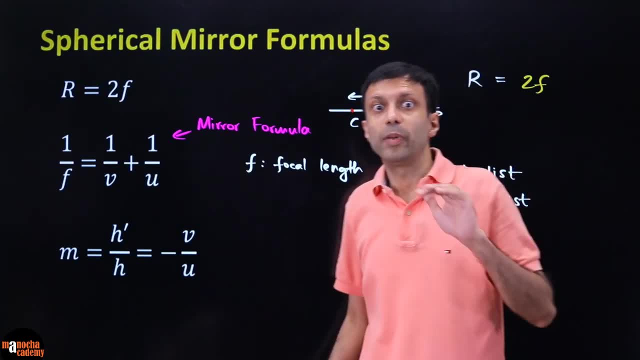 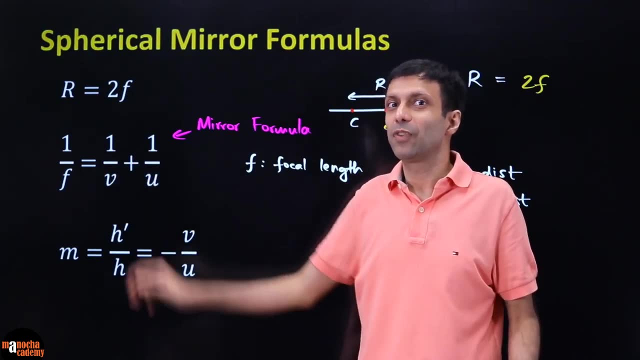 This will become 1 by V minus 1 by U, So please be very careful of the sign. Mirror formula is 1 by F equal to 1 by V plus 1 by U. Lens formula is 1 by F equal to 1 by V minus 1 by U. 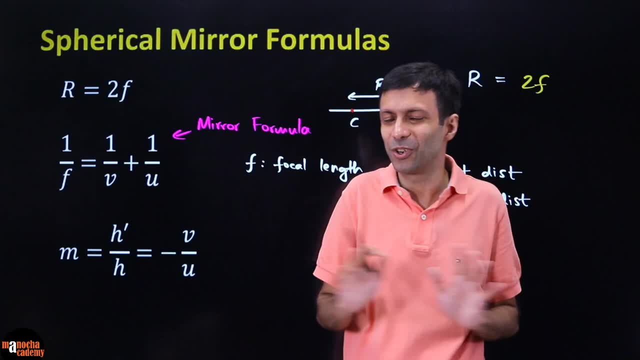 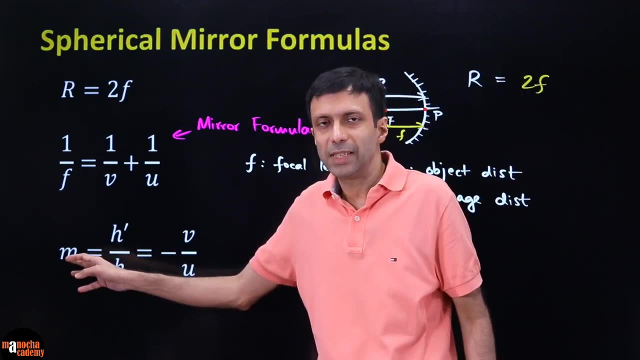 So please do not mix the two. Always check: are you doing a mirror question or a lens question? It is a very common mistake. Next formula is called: Do you guys know what does this M stand for? What is M? M stands for magnification here. 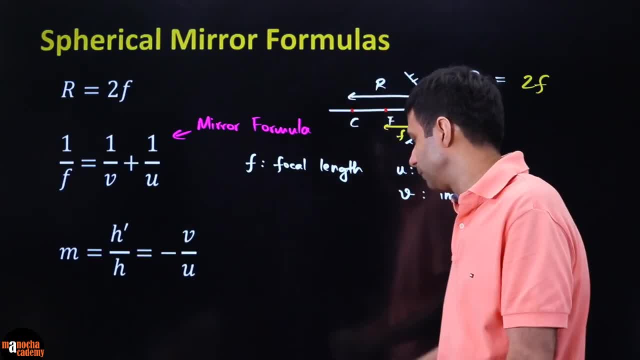 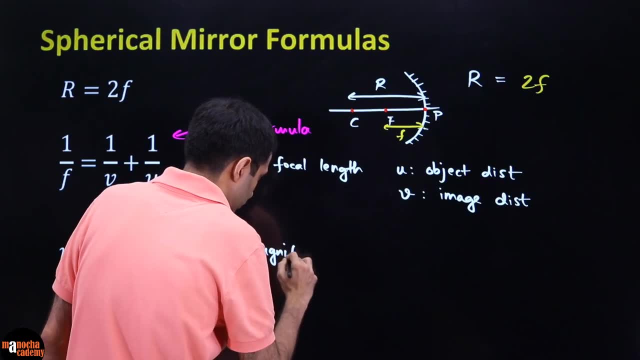 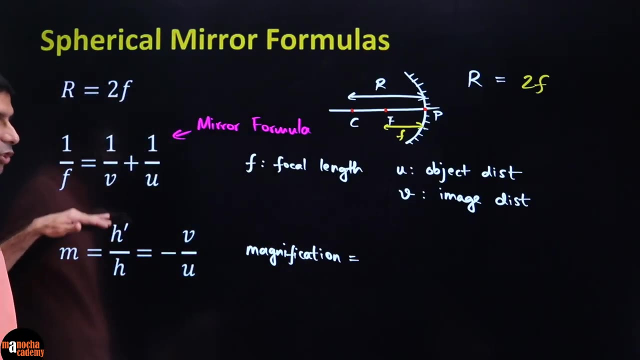 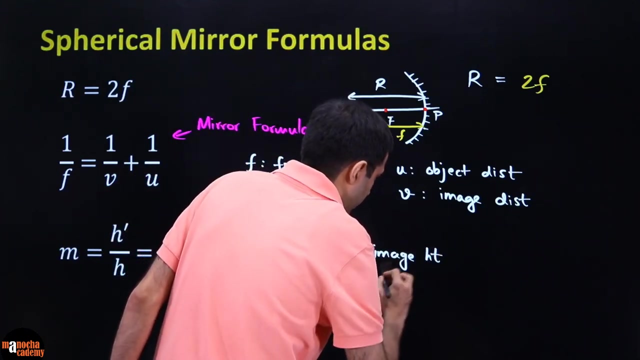 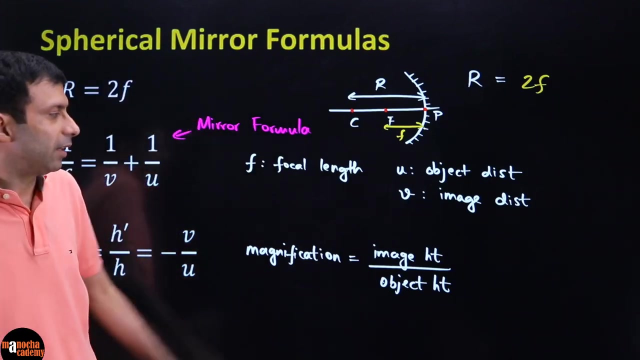 And H dash and H. So basically, what is this formula saying? M is the magnification, So magnification is the ratio of the image height to the object height. So it is. So it is Image height divided by object height. So that sort of makes sense, right? 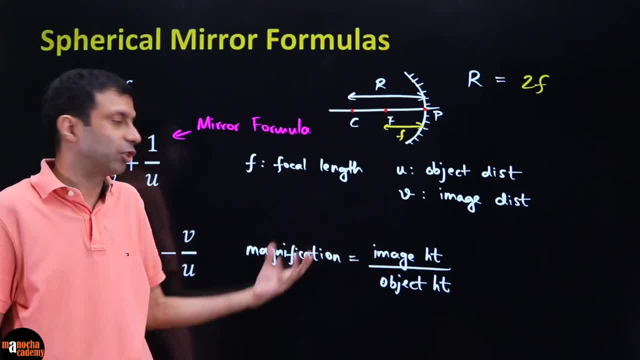 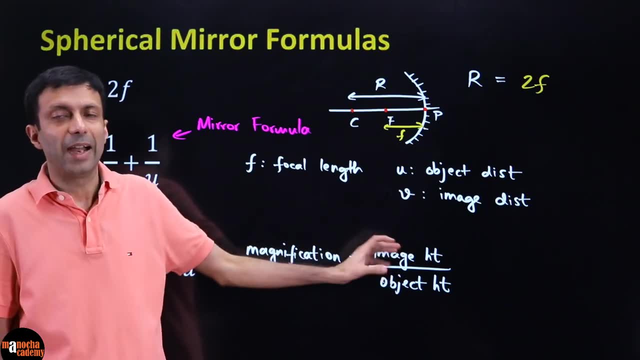 If the image is 2 times the object, it will be 2 by 1.. 2 right Magnification will become 2.. So always, image height divided by object height. This is the ratio. And let us say: if image is measured in, the heights are measured in centimeter. 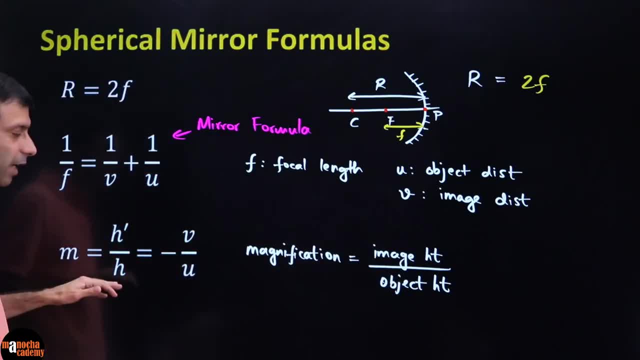 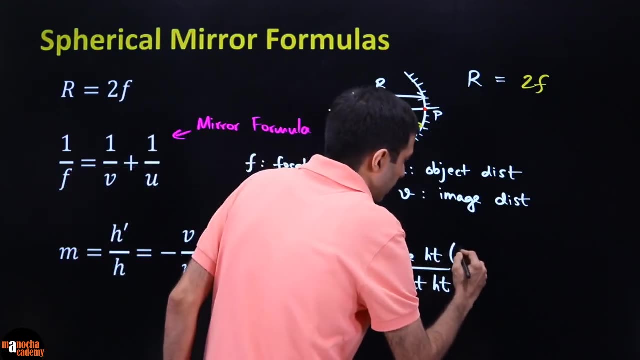 Obviously you can see the unit will cancel. So this is the magnification formula: H dash by H. Now one very interesting thing thing: magnification is connected to the image and object distance. how magnification? image height by object height. so this is our M. image height is labeled as H dash. in some of the books it might. 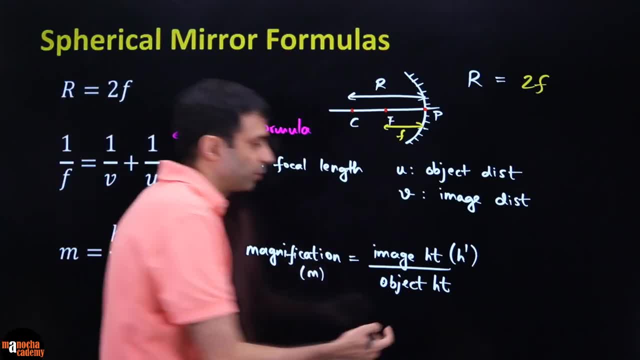 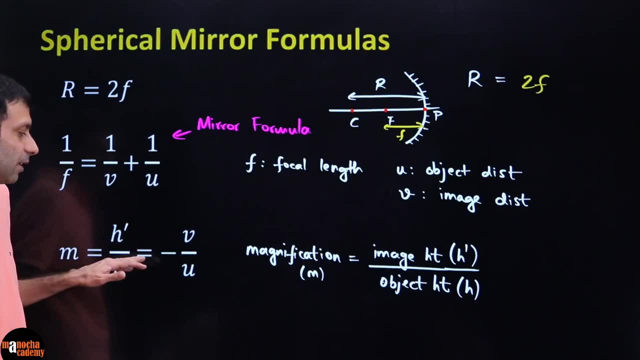 be written as H- I for image and HO for object height, or H- dash and H. so whichever convention you are using, and that is equal to image distance by object distance, but with a negative sign. so again, please don't forget this sign, otherwise your answer will be wrong. okay, so this is the 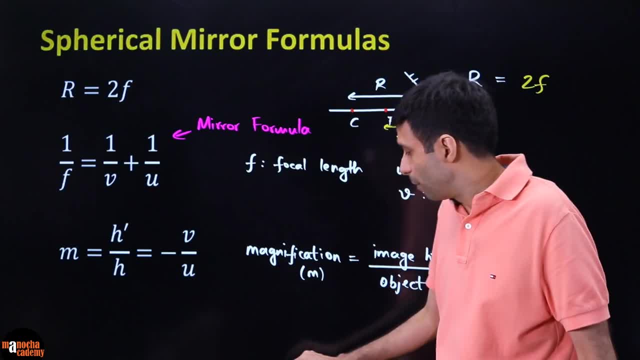 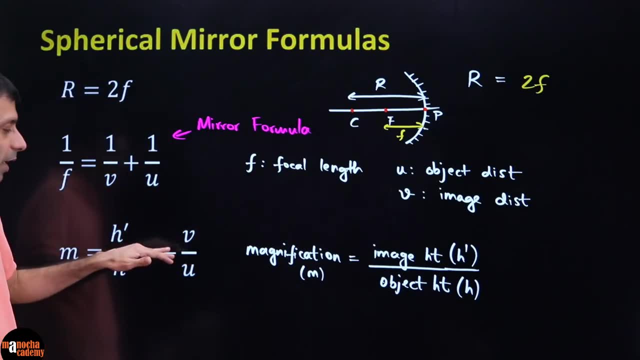 other important formula, and this is that's why it is called as magnification formula, because it is connecting the magnification, the image height by object height. this is the basic formula, but it is also connecting it to image distance by object distance. so this is our magnification. 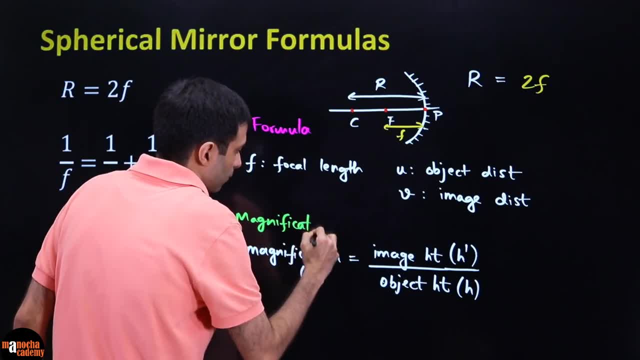 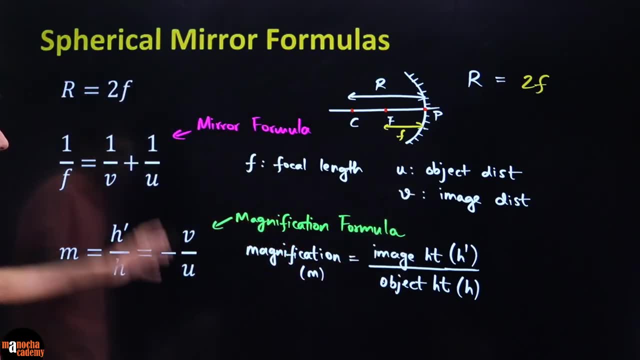 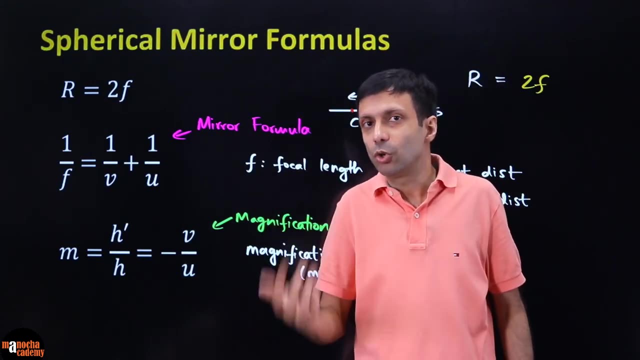 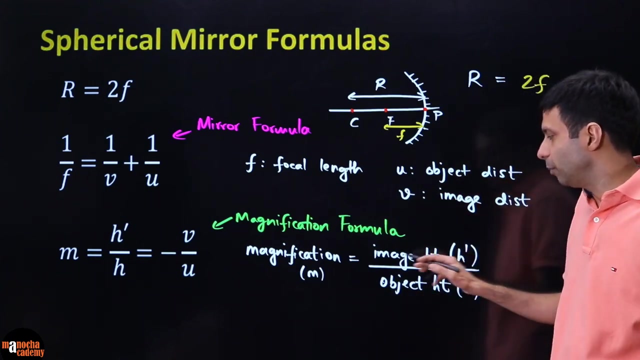 distance very important. please write and learn these formulas. the best way to learn the formulas: write it down and keep using it in the questions and whenever you are doing the sums, please write down the formula, then substitute. don't directly substitute, okay. HT stands for height, image height. 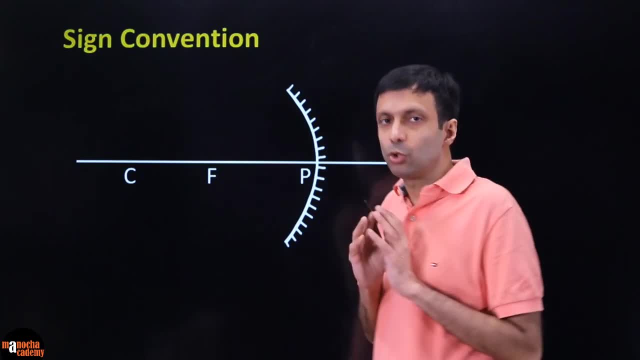 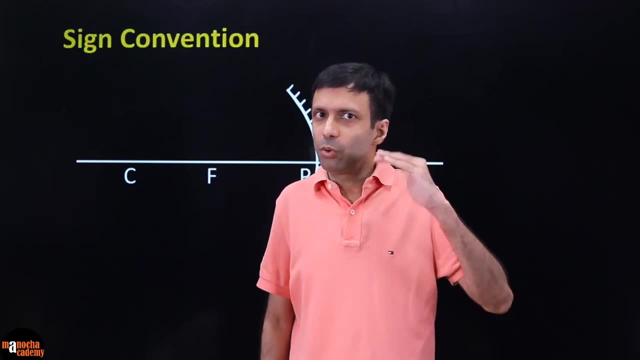 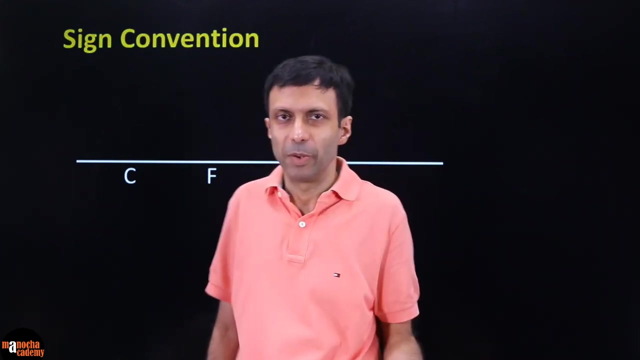 by object height. now, one very important thing: when we are using these formulas, we have to follow a sign convention. this is super important because if you write the wrong sign, gone right, you did everything right, but one sign mistake. the whole answer will be wrong. so let's carefully understand what is sign convention. I've 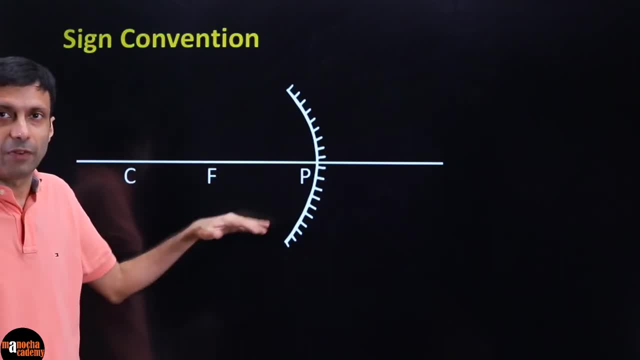 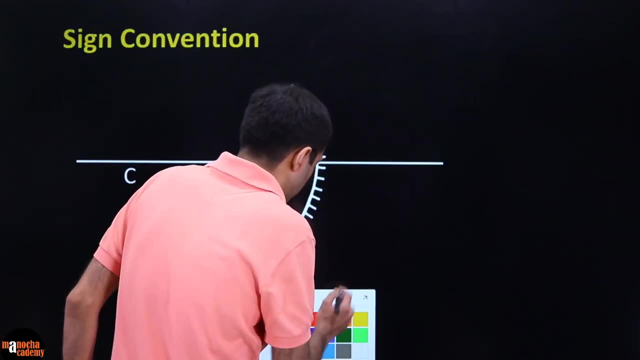 explained it in my video also in detail. please watch that previous video here. we'll do a quick recap. so we are using the example of concave mirror. here you can see there's the back part of the mirror and these are these three important points. pole is the center of the mirror, this is the center of that. 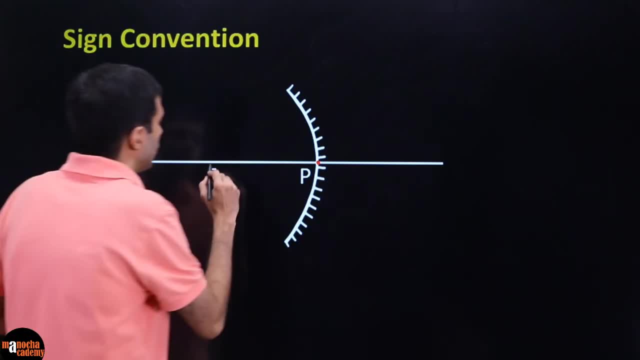 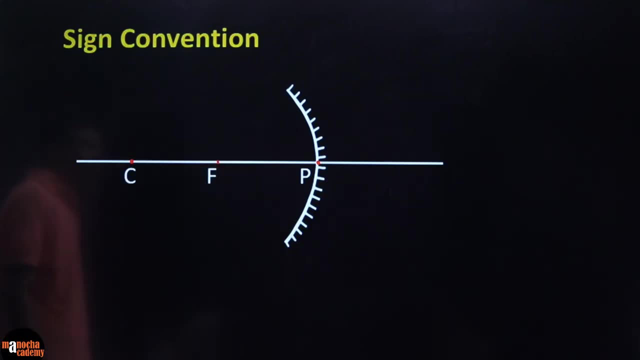 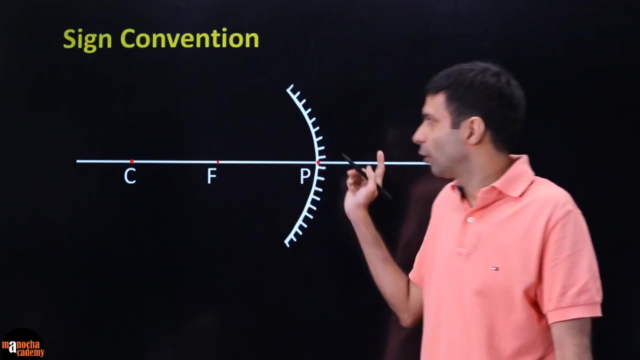 curved circle which is called center of curvature. see, and then you have the focus here, which is exactly in the middle of pole and center of curvature. okay, now, what is the sign convention say? one thing about: very important is when you are measuring image and object distance, they are measured from the pole. 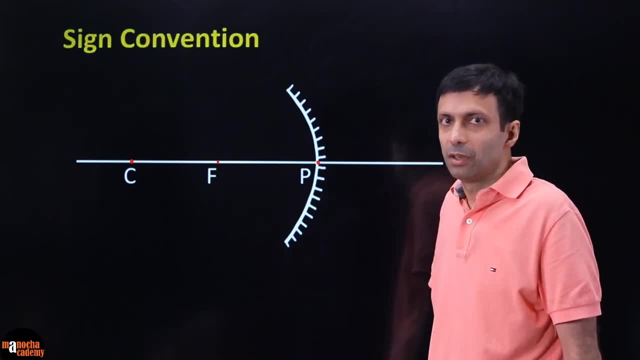 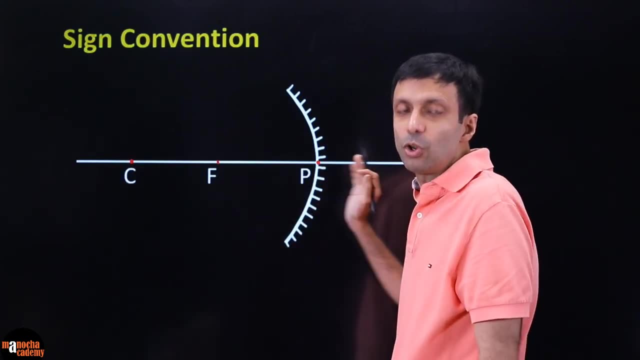 okay, so according to sign convention, distances are measured from the center of the mirror and the center of the pole and the axis that you measure. to this left side they are negative and to the right they are positive. so how can we easily remember that? it's as if you are. 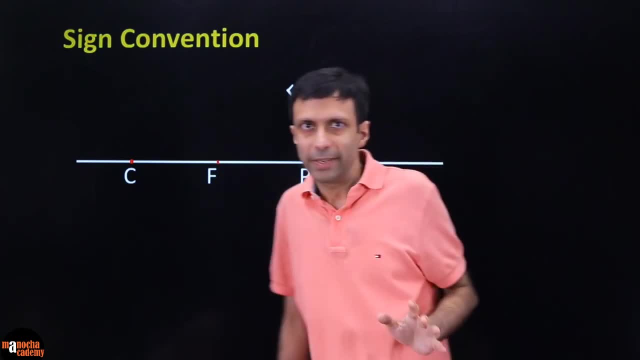 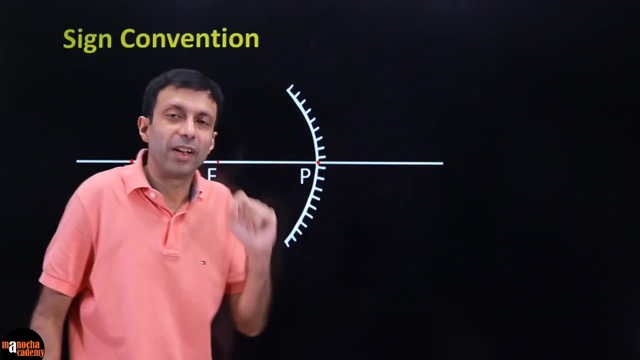 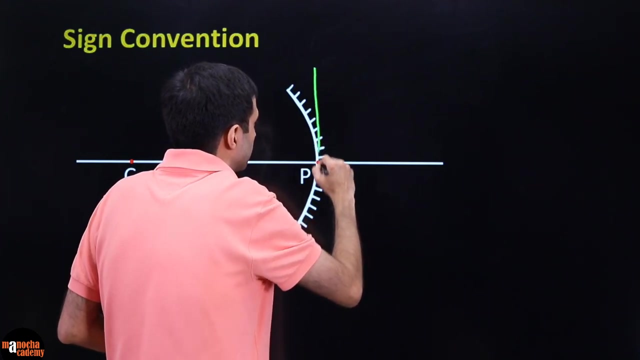 placing the coordinate axis at the pole. you have done coordinate geometry. you know there's the x horizontal axis and by the vertical axis, so please place those coordinate axis here, where the origin is at the pole. okay, so I want all of you to draw the coordinate axis like this: this is my y-axis. 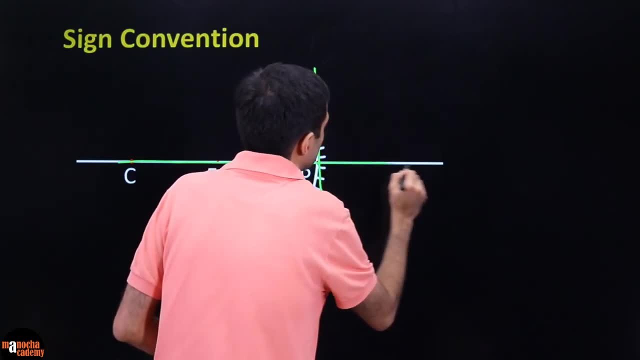 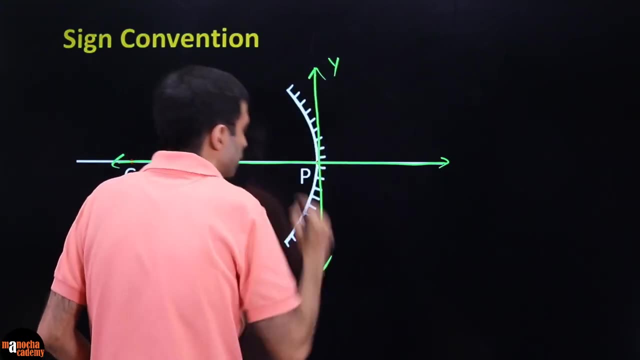 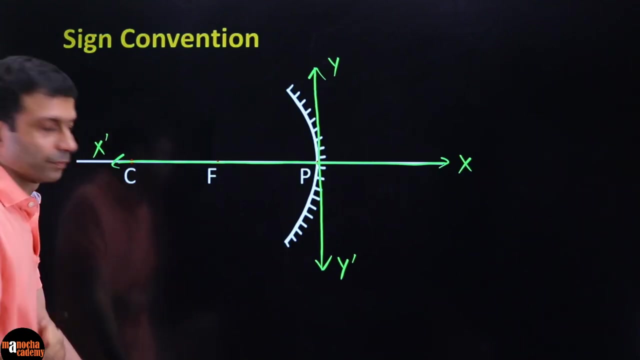 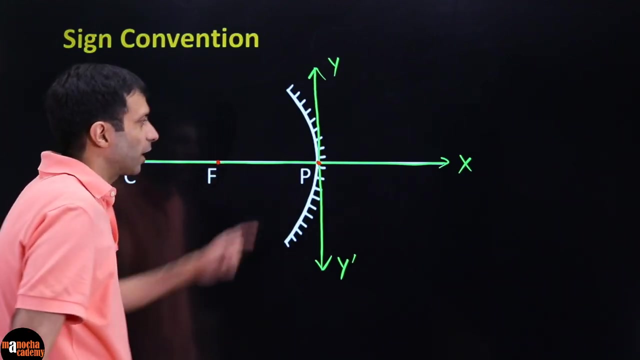 and this is our x-axis. so this positive y-axis we label as Y, negative y-axis, y dash, positive, x-axis, negative, x-axis, x-dash. this is our pole focus and center of curvature. so can you see poles like the origin where the x and y axis meet. so what a sign, convention, mirror ан. 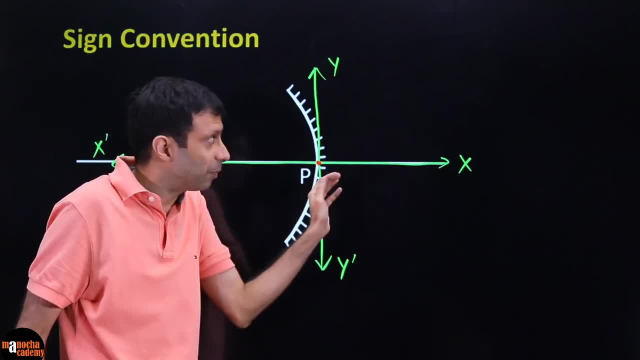 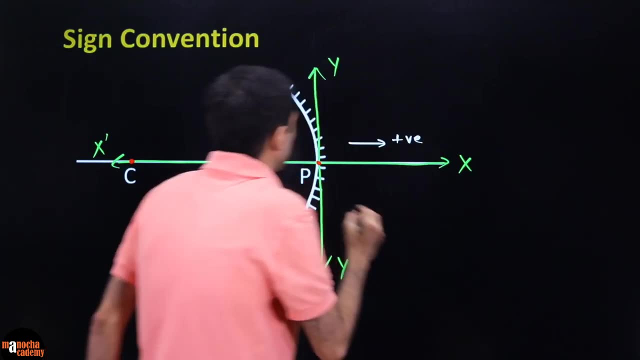 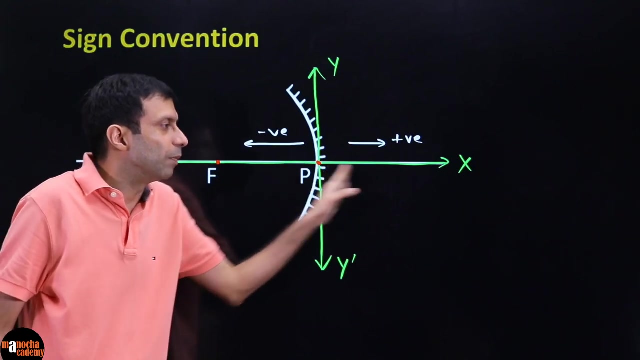 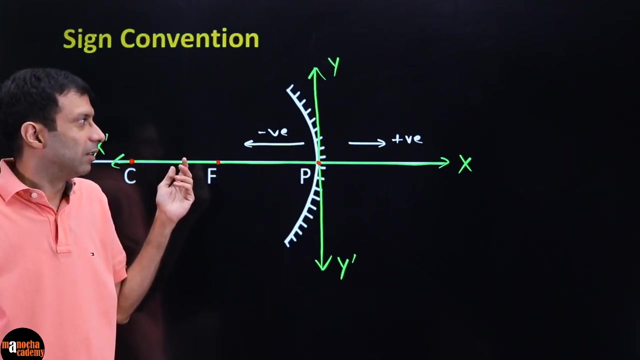 say any distances, you are measuring to the right. that means along the positive x axis. these distances are considered positive. anything measured here is negative. and remember, all measurements are taken from the pole. so you measure just like this, just like coordinate geometry, you measure from the origin. same way over here. okay, and when you are measuring, 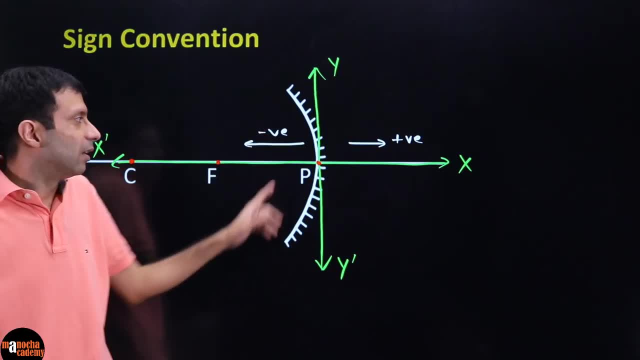 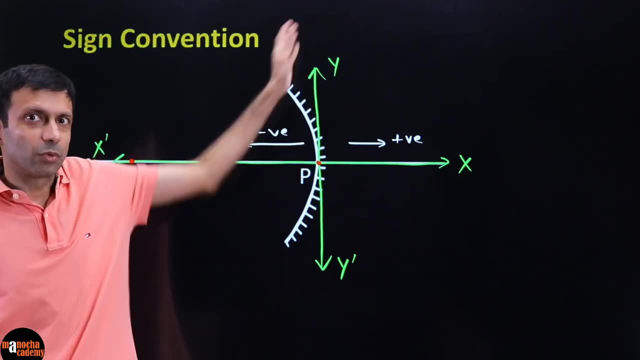 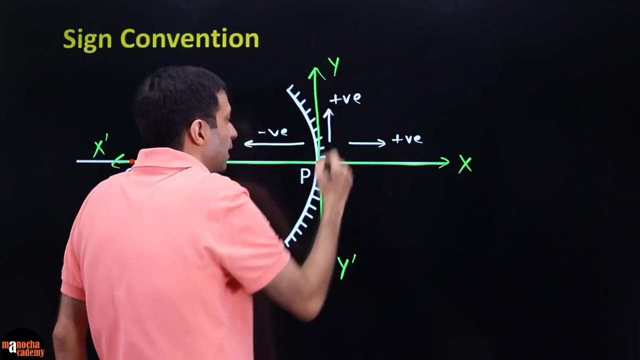 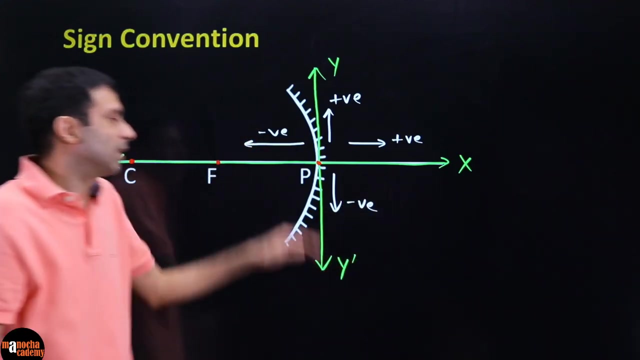 heights. so object height, image height. then you will be measuring along the y axis. that makes sense. so anything measured upwards. so if the object is upright, usually the object will be upright. so all these heights will be positive. but anything which is inverted- like you know, we can get an inverted image- they will be negative. so once again they are. 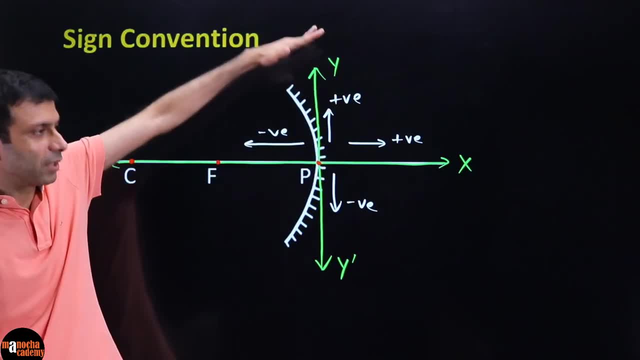 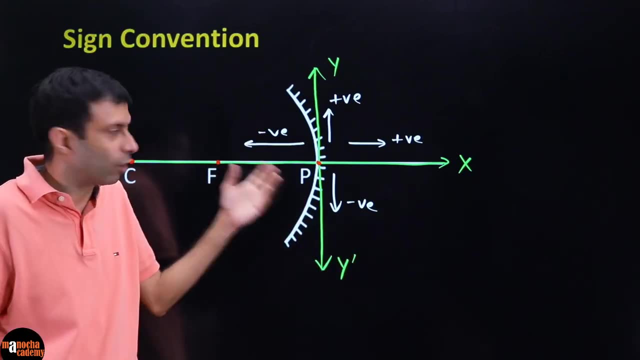 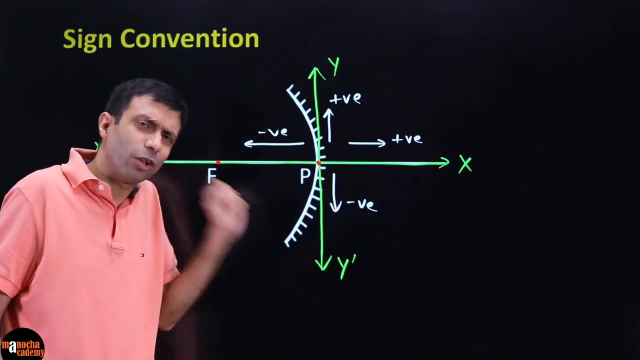 measured again from the principal axis. you are measuring anything above positive, anything below negative. This sign convention is super important. so the easiest way I remember sign convention is I draw this rough diagram: concave mirror, convex mirror, whatever some you are doing, make sure you draw those coordinate axis, because when you draw the coordinate axis automatically, 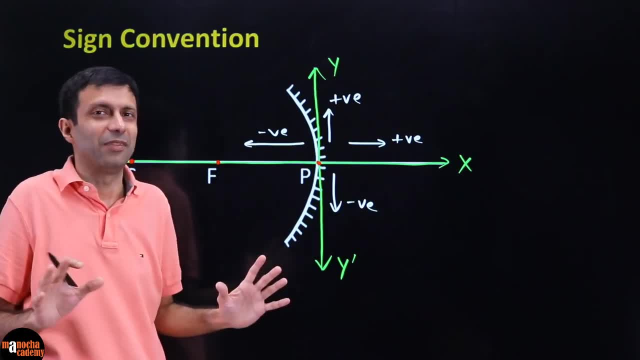 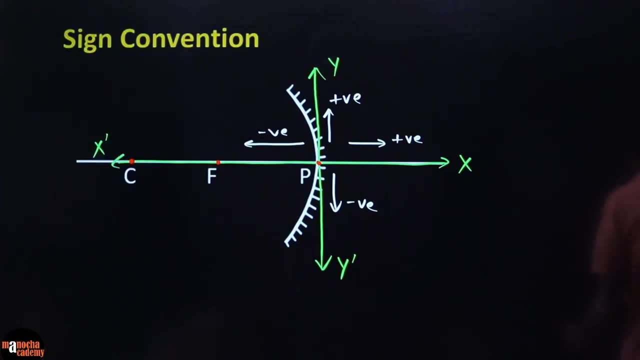 your coordinate geometry brain starts working. you start thinking positive, negative, okay, otherwise the whole thing will go wrong. so be very careful of that. yes, and this is looking like the Cartesian plane with the four quadrants. very good Shiva. very good Jitesh, exactly Okay. 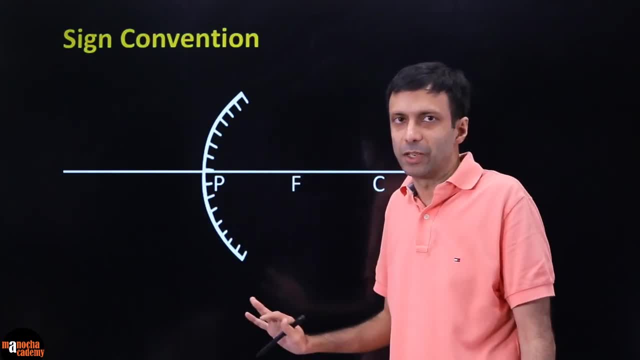 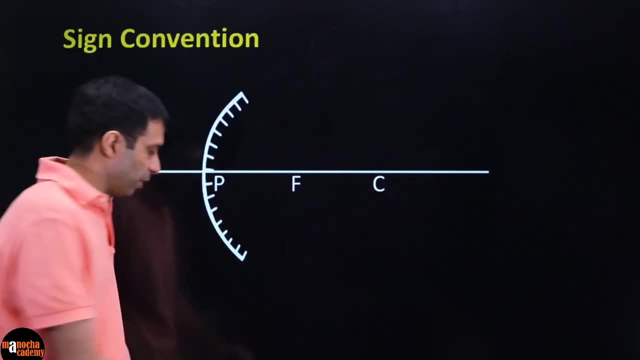 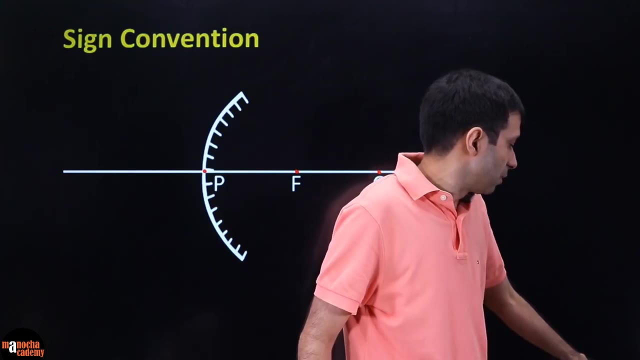 The same sign convention works for convex mirrors also. so here, once again, you will draw your coordinate axis at the pole. so remember again, we have pole focus and center of curvature and remember I told you so, remember, I told you guys that this, this PFC is there is a mistake. 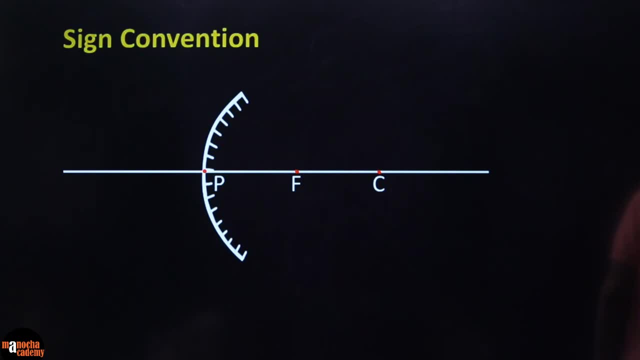 in that previous video. we will have it corrected, okay, hopefully by next week. that editing needs to be fixed, But make sure the these are behind the mirror in convex mirror, right? so important difference here. you can see in a concave mirror the PFC are in front of the mirror. why? because 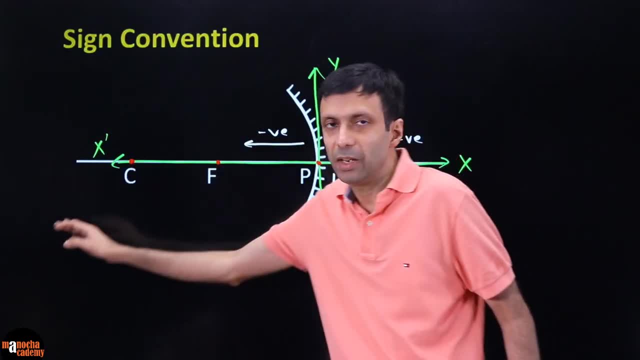 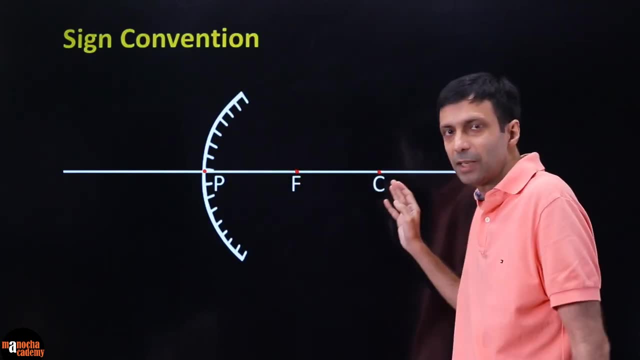 this is the center of the circle. obviously it should be here, so PFC should be in front of the mirror. here the circle completes like this. so this will be the center of the circle, so PFC will be behind the mirror. so this is very important for you guys to remember now. 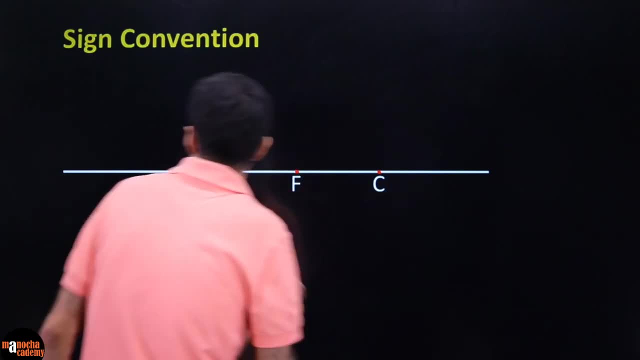 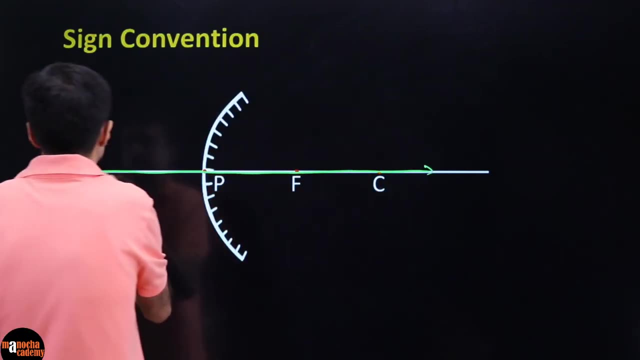 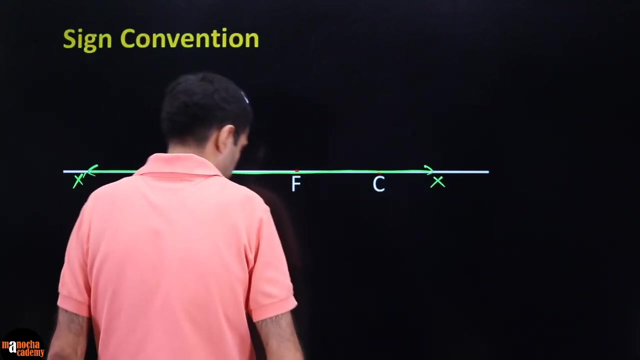 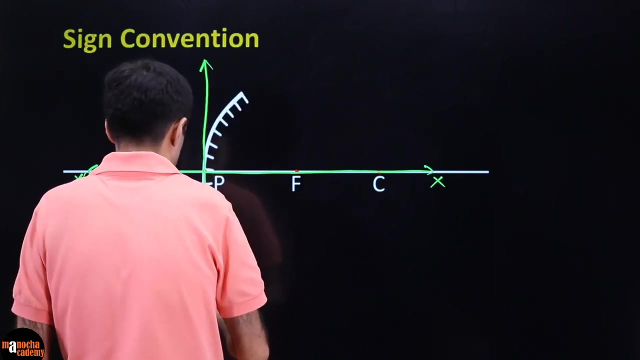 please draw the coordinate axis, So. So coordinate axis will be like this: this is my x axis. so x and x dash. So x and x dash will be foremost. So x and x dash, y and y dash, x and x dash. this is my x and y dash. 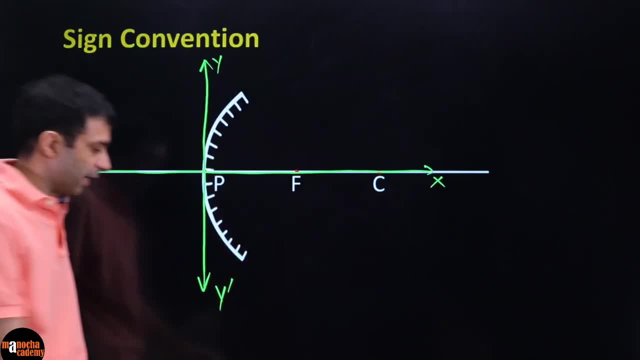 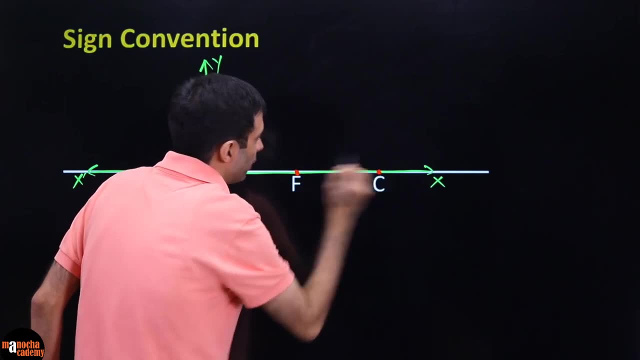 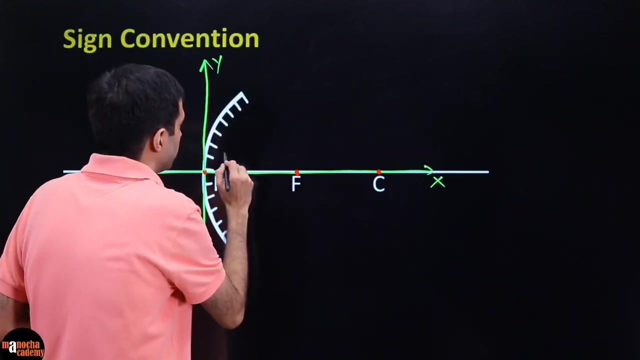 Okay, So this is coordinates. So that will be my y axis, always 6x. Okay. So remember, the pole is the origin. your focus is exactly halfway between pole and center of curvature. So, once again, if we measure distances this way from the pole, this way will they be positive or negative? 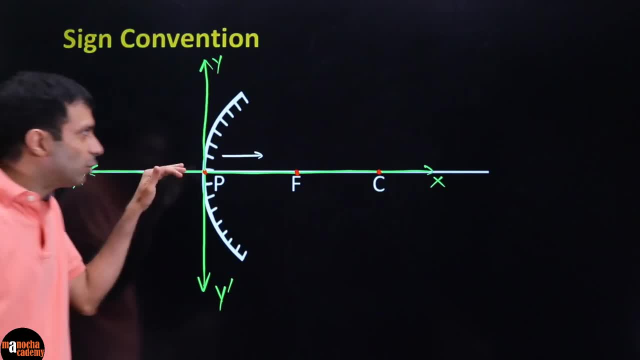 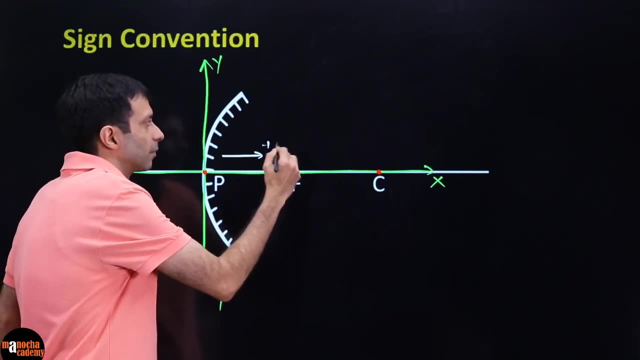 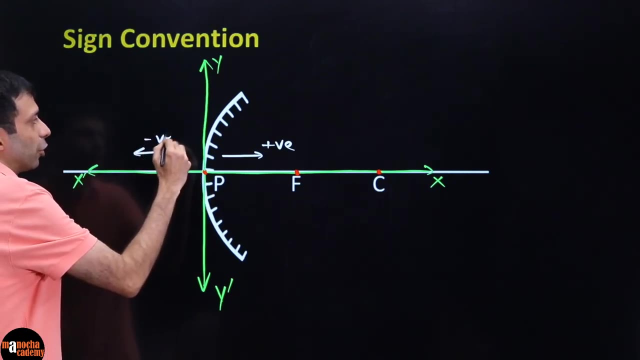 According to sign convention. this is called sign convention. So, as you can see, these distances are measured along the positive x-axis. So definitely they will be positive. Now, if you are measuring some distances this way, this is along the negative x-axis- negative for sure. 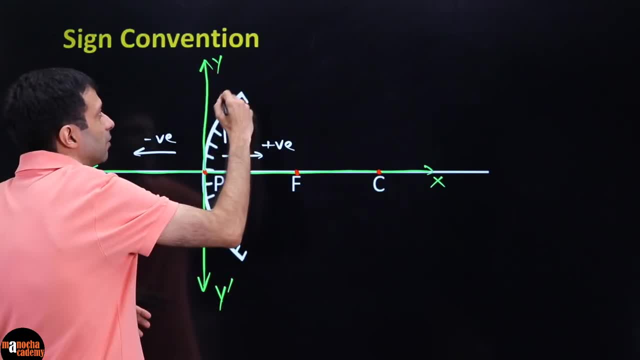 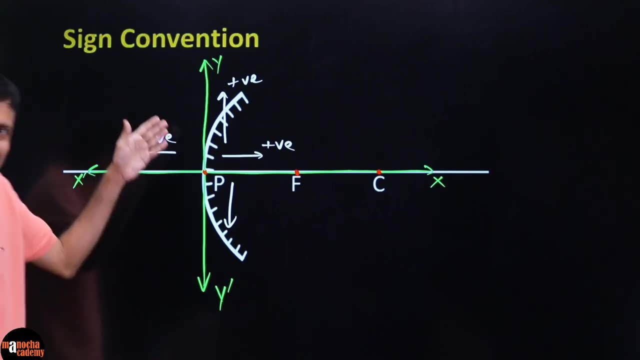 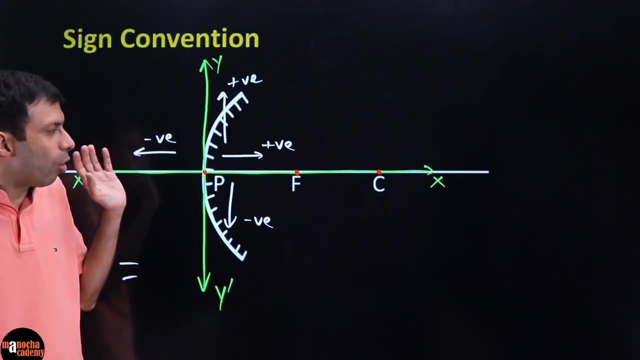 If you are measuring heights above the principal axis, definitely positive, because positive y-axis. If you are measuring below the principal axis, you are going down here. definitely they will be negative. So this is important: always draw this axis Axis. you will never forget the sign convention. 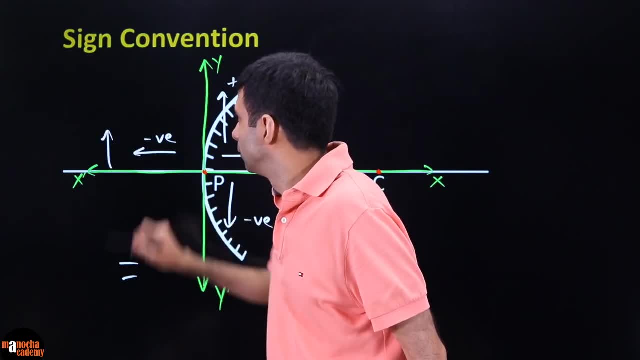 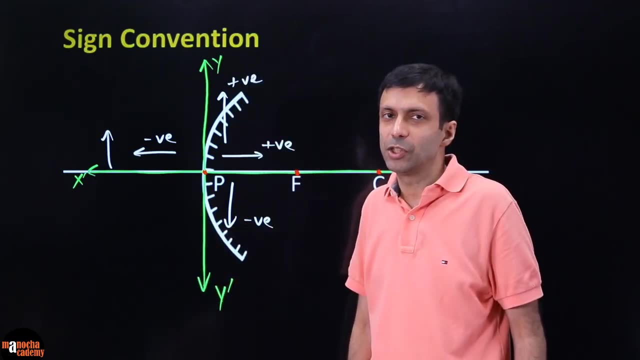 So, for example, you know, if an object is kept here at, let's say, a distance of 5 centimeters, what will be the measurement? Will we write plus 5 or minus 5, if an object is kept over here? 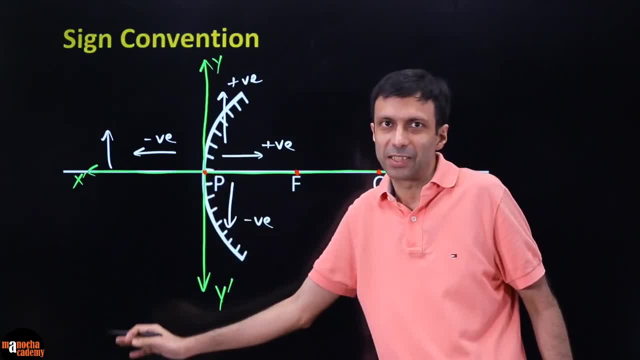 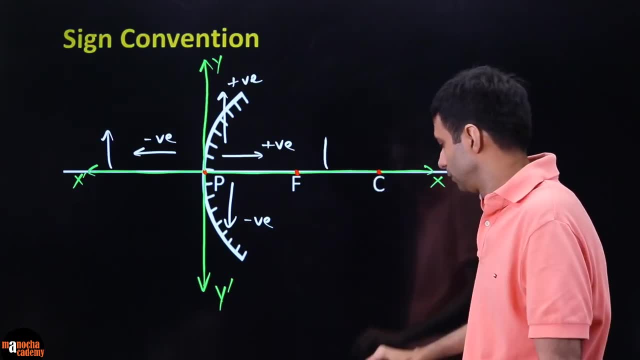 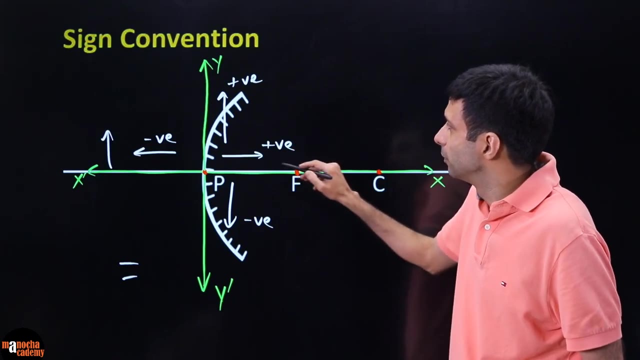 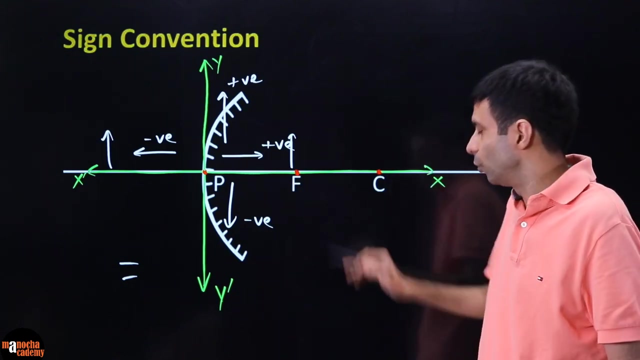 Very good. minus 5, because you can see it's on the negative x-axis. If an image is formed here, let's say an image is formed somewhere here, Let's say it's at 4 centimeters, so plus 4, because it's along the positive x-axis, clear. 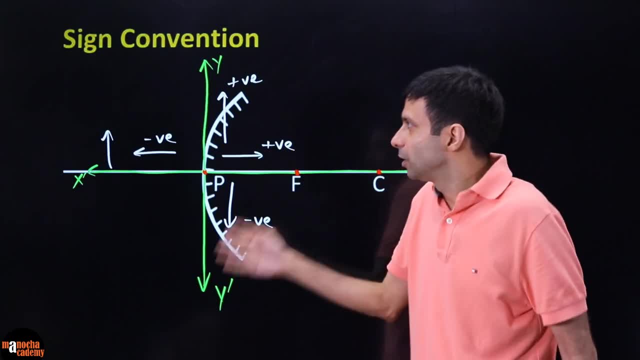 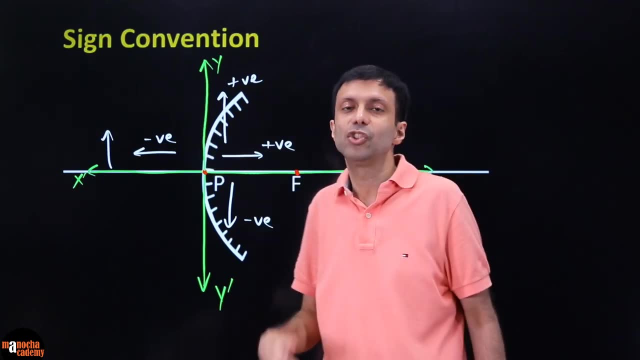 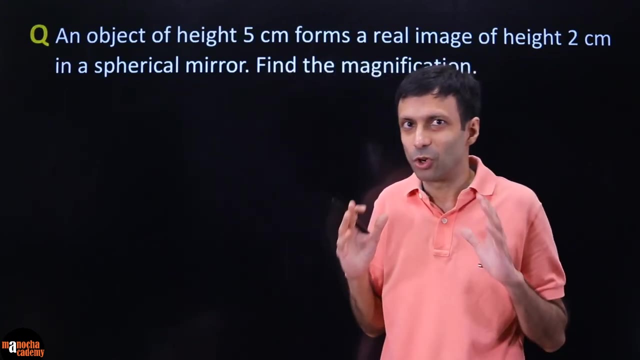 So we have to follow the sign convention: the distance right. Similarly, if it's an upright object, positive height. If the image is upright, positive. If it forms an inverted image, negative height. So let's practice this sign convention in the mirror formulas using sums, because in today's class we are going to focus on sums. 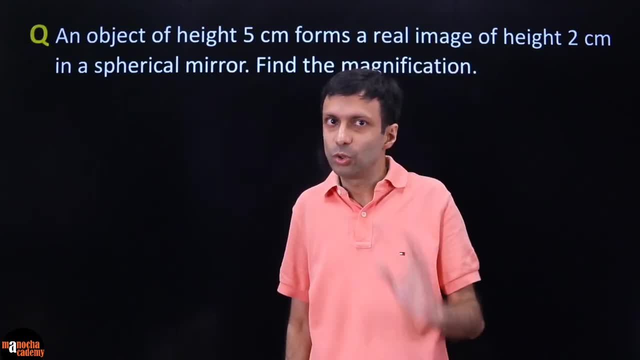 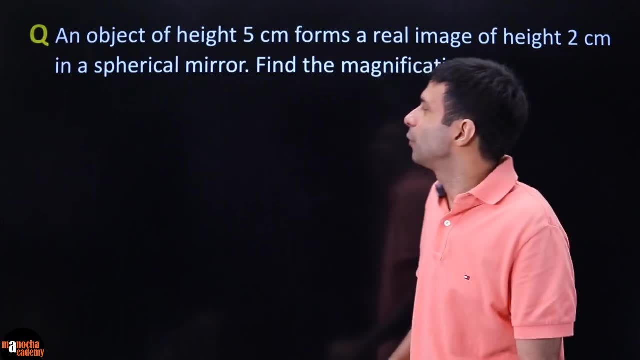 And I am going to show you some very easy, important tricks. if you use that, you will get it right. Okay, so please try to follow these tricks and I am sure you will not make a mistake. So let's start with the first question. 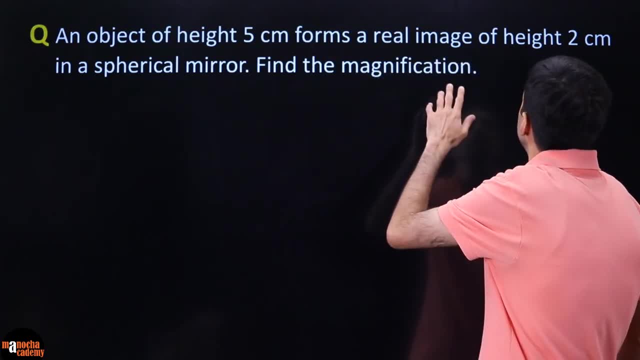 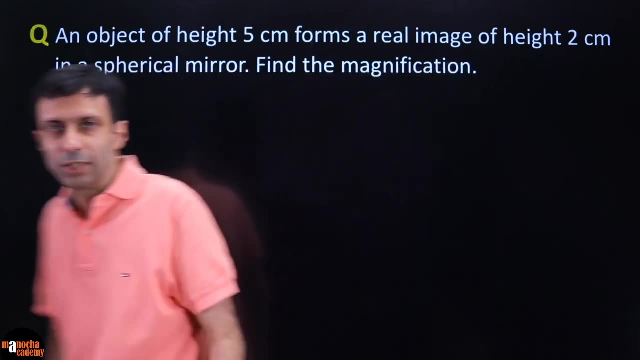 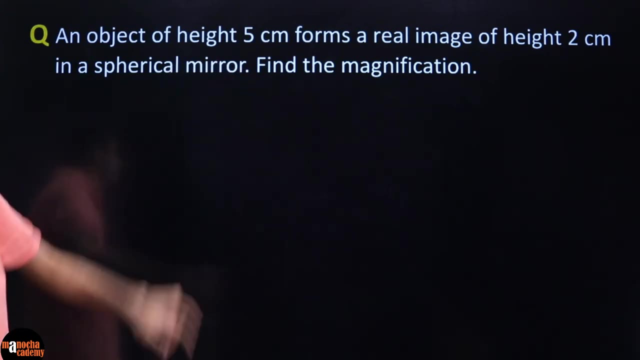 An object of height 5 centimeters forms a real image of height 2 centimeters in a spherical mirror. Find the magnification. So can you guys do this for me? An object of height 5 centimeters forms a real image of height 2 centimeters in a spherical mirror. 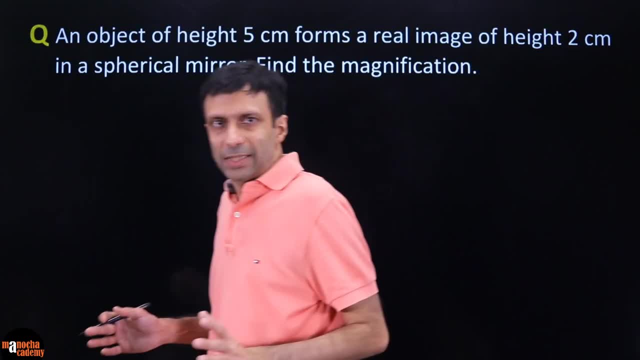 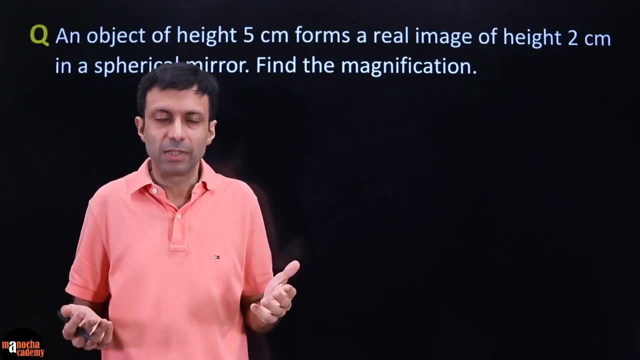 Find the magnification. So always, whenever you are doing sums, first thing is read the sum carefully, note down all the data and use the kind of symbols, the standard symbols that you know, like u, v, f or h, h. dash right. 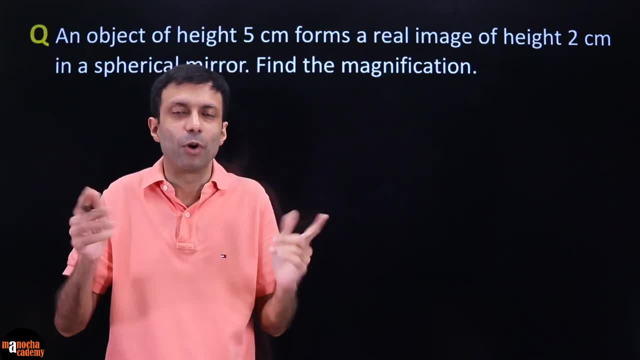 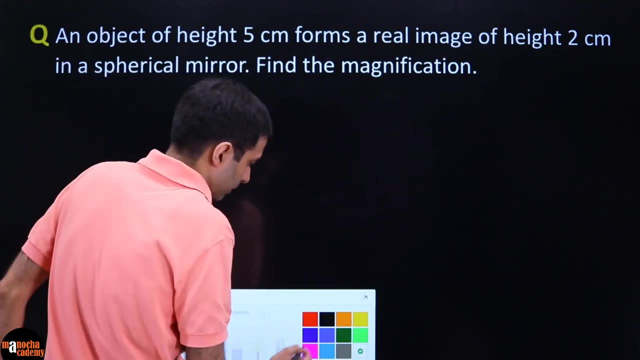 Because that will relate you to the formulas. That way you can easily remember the formulas if you write it in terms of standard symbols. So let's read the formula: An object of height 5 centimeters forms a real image of height 2 centimeters in a spherical mirror. 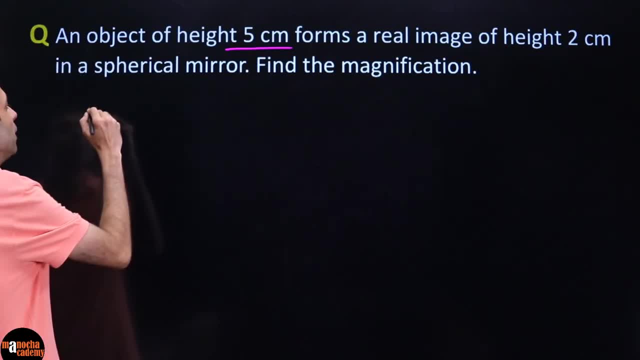 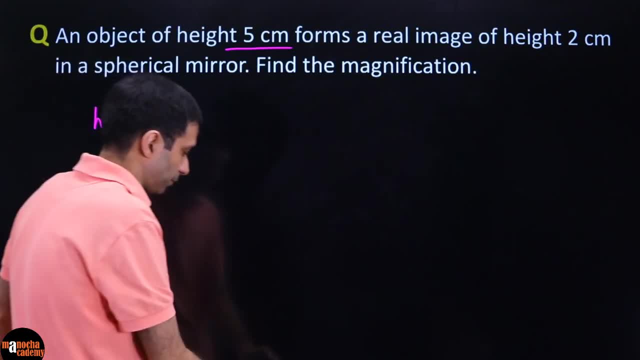 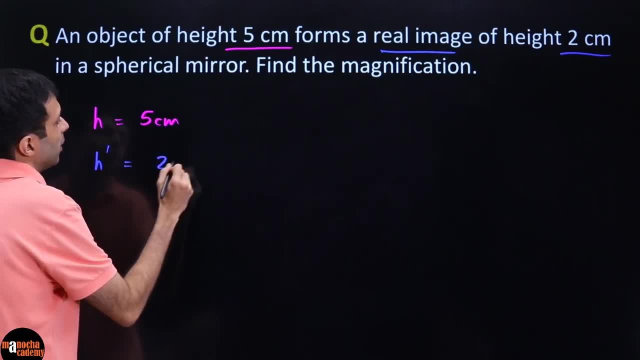 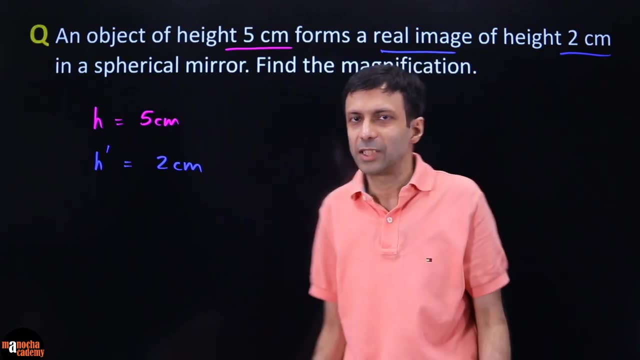 Find the magnification. An object of height 5 centimeters forms a real image of height 2 centimeters in a spherical mirror. Find the magnification in a spherical mirror. so they haven't told us whether it's a concave or a convex mirror, so it 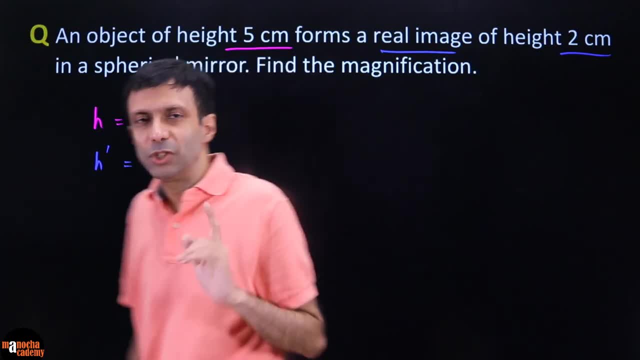 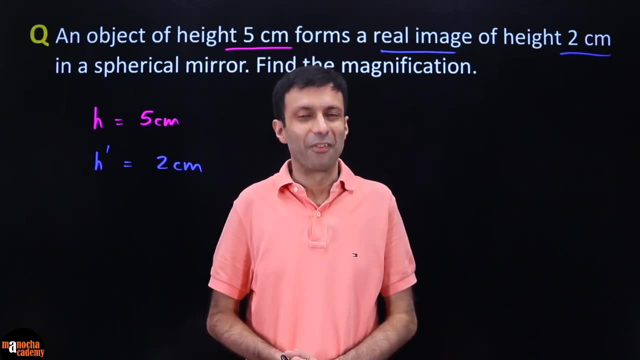 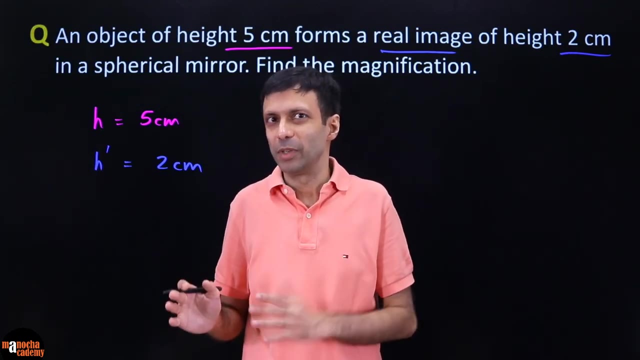 could be either, but which one do you think it will be? real image? who gives concave or convex mirror? can you guys tell me who gives a real image, a concave or a convex mirror? very good, correct answer is: only concave mirror can give real image. convex mirror only gives virtual image, which means 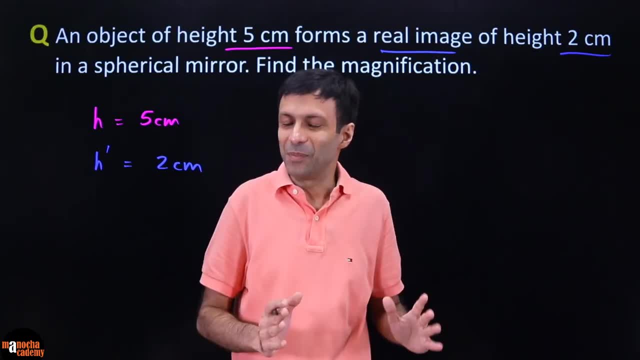 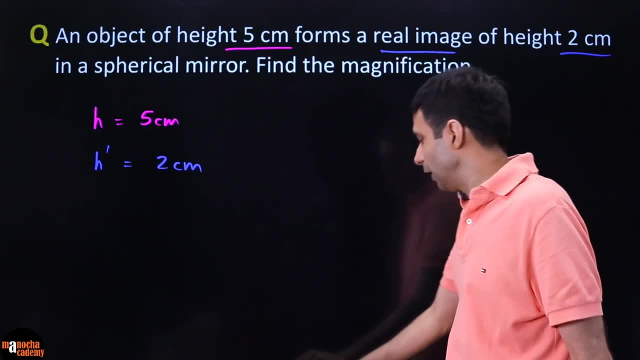 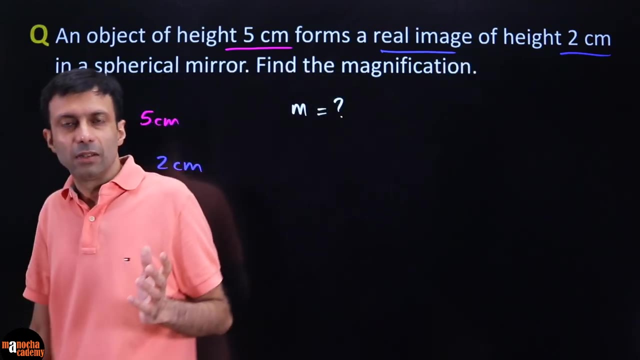 only the image can form behind the mirror. for convex, concave mirror can give real image very good. so that that's another thing that you guys know. and now the question is: find the magnification. so we need to find what is the magnification here. so if you guys remember what is the formula for magnification, see, we are going to use that simple. 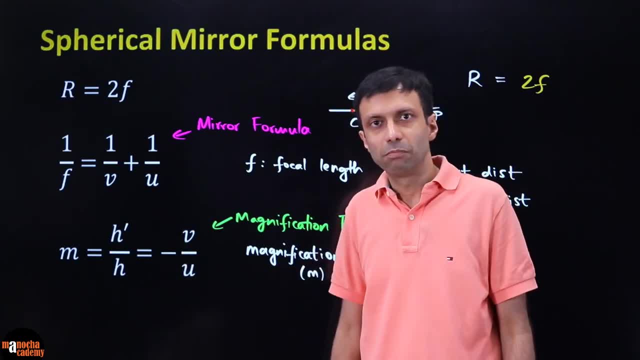 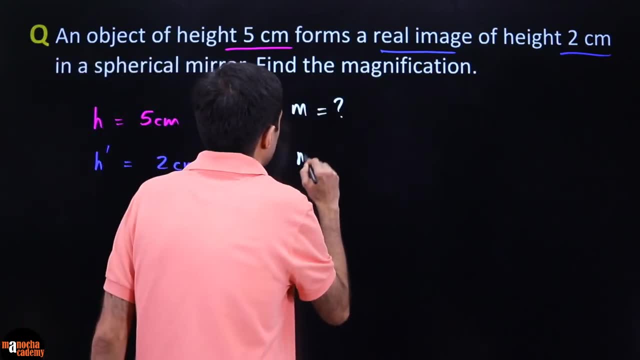 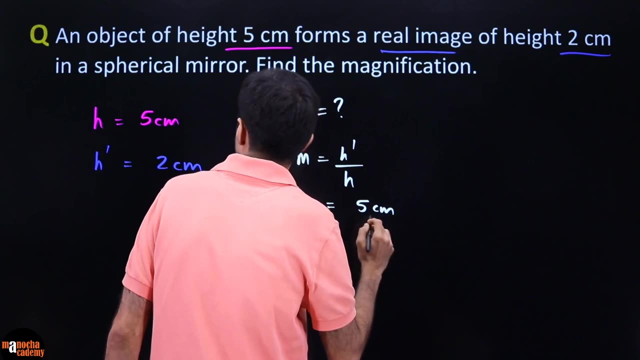 magnification formula m is h dash by h. so that's it. we just go ahead and use it. so let's go ahead and substitute the values here. magnification is h dash by h, 5 centimeter by sorry, 2 centimeter by 5 centimeter. 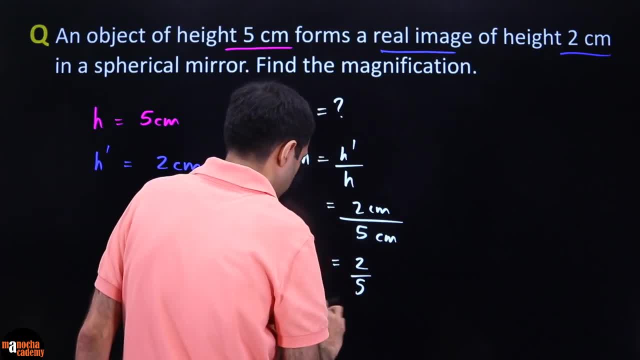 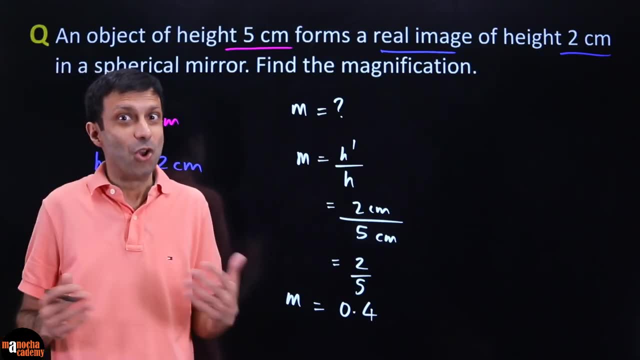 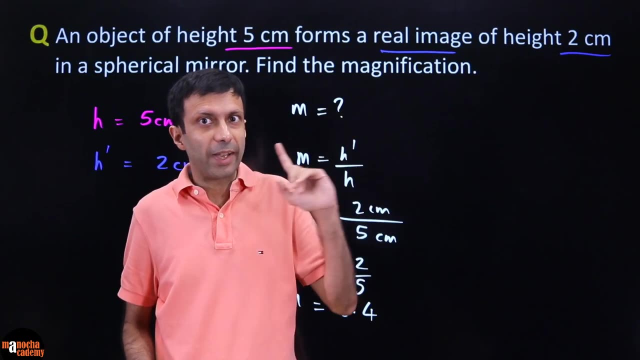 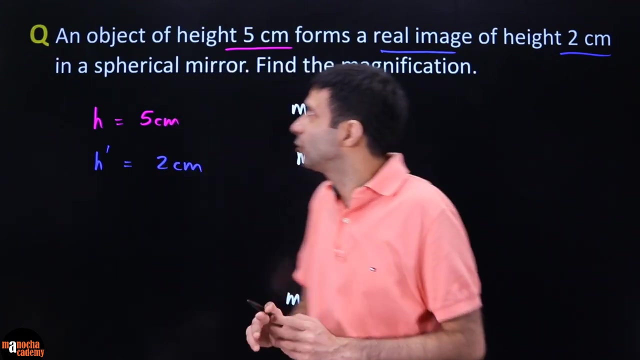 so 2 by 5- which is magnification- is 0.4. so is this the correct answer? many of you are thinking no. so this is what i told you: sign convention is very important. do not just write down the data. you need to write the data with the correct sign. so what is the mistake we have done here? so let's read it. 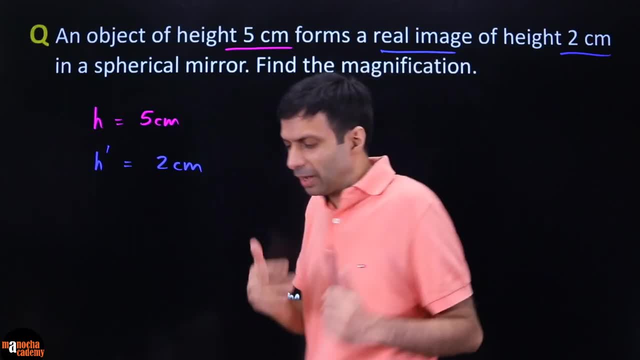 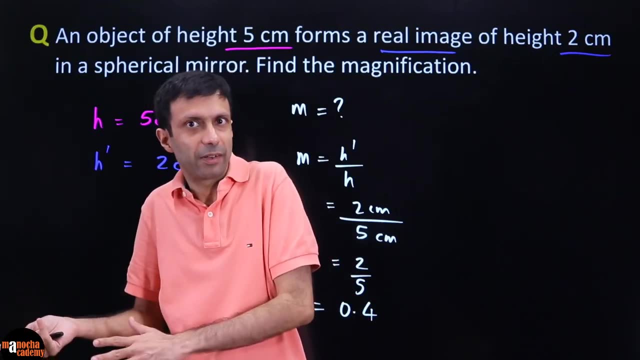 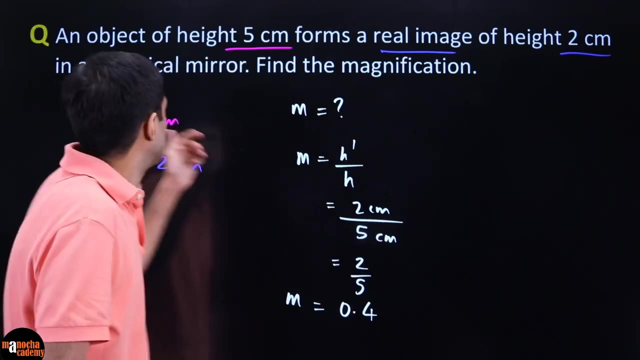 carefully. object of height: 5 centimeter. now they haven't told us whether the object is upright or inverted, but usually object is upright, otherwise they would have said inverted object. right. so if object is upright, that means it's along the positive y axis. this sign is correct, positive, in fact. to remember it, you can even write plus 5. 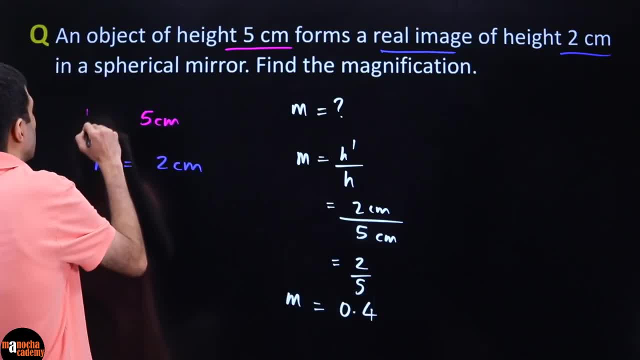 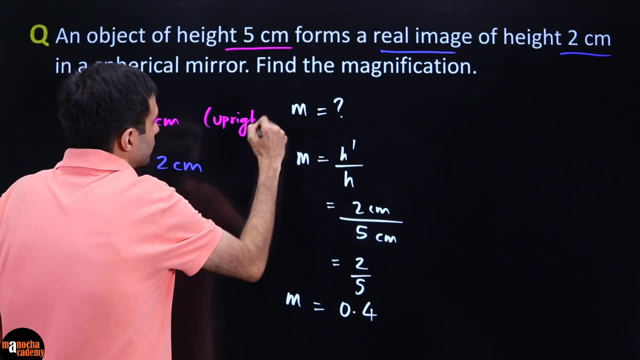 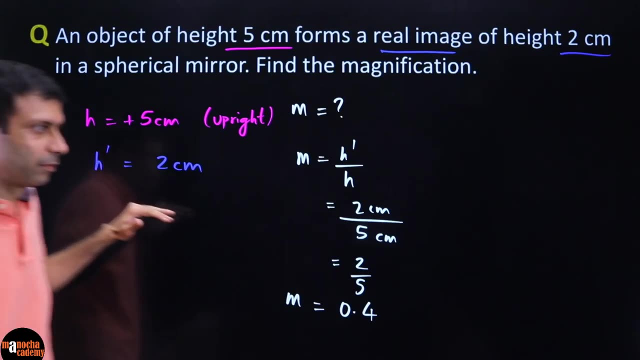 so you, that means you have thought of the sign. so you can write: h is plus 5. why? because it is upright. you don't have to write the reason. this i'm just telling you to explain you. what about the image? image, you can see it clearly says it forms a real image. now, real images are they? 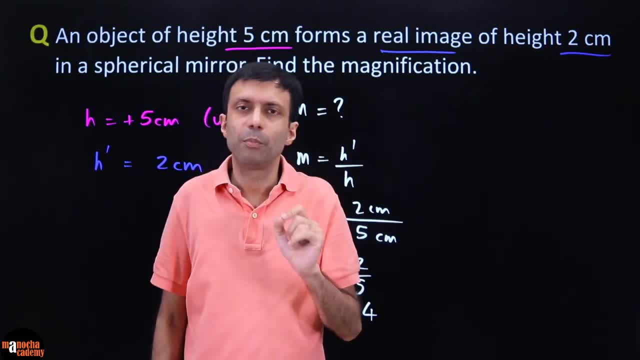 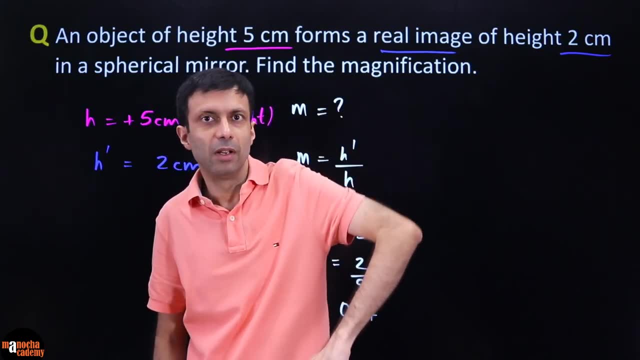 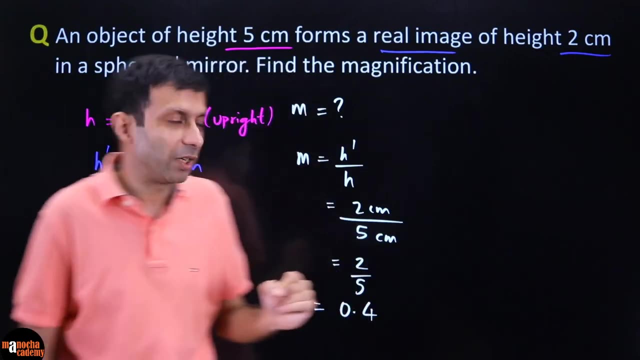 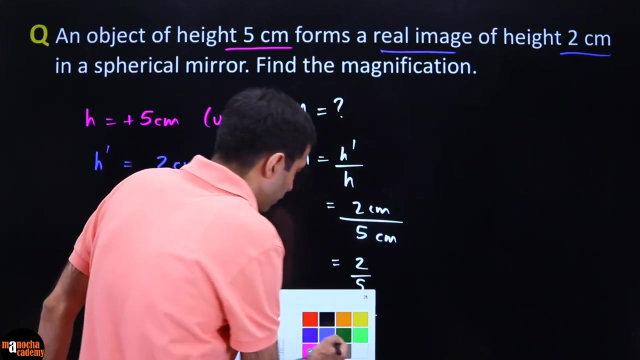 upright or are they inverted? this is very important rule: real images are always inverted. real images are always upside down. inverted virtual images are always erect or upright. okay, so that means real image means it must be inverted. so if the image is inverted, it's along the negative y axis. yes, so it has to be. you have to write it with the correct sign. so 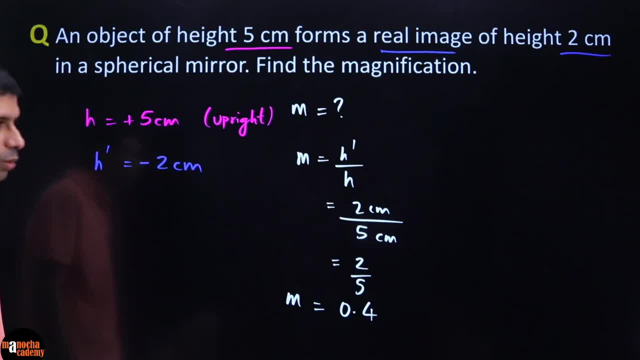 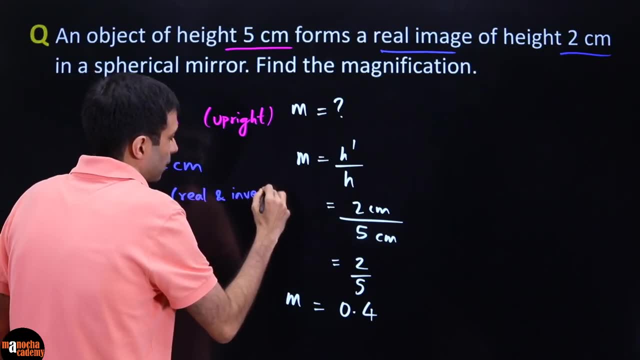 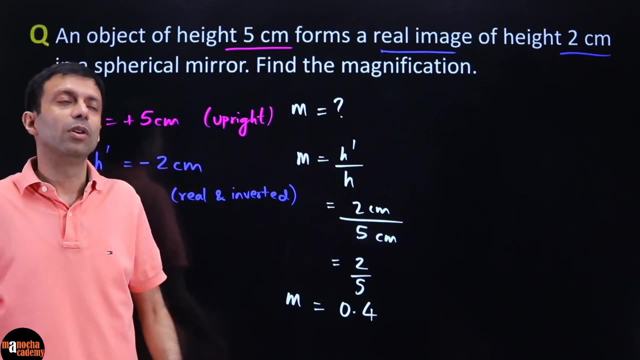 all this data has to be at the right sign. it should be minus two centimeters does, because it is a real and inverted image. they won't tell you in the question. please write minus two. you have to work out the correct sign. it's like you know somebody made a loss of rupees. 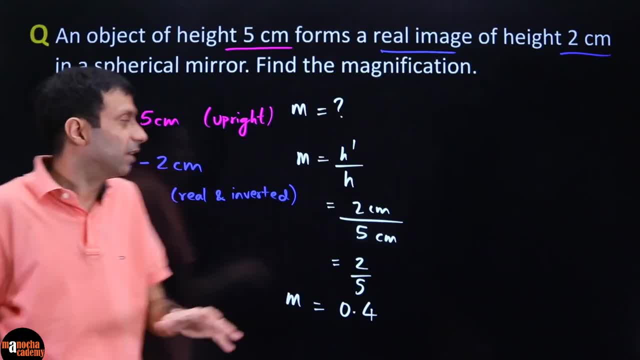 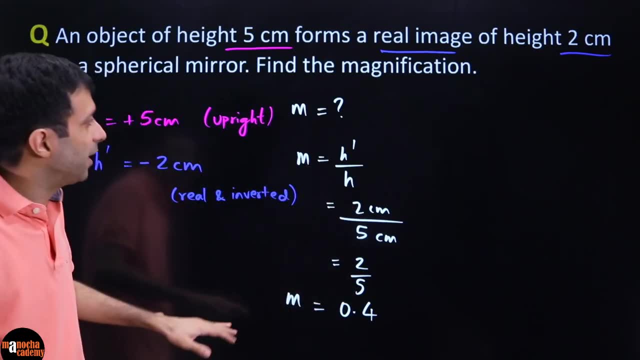 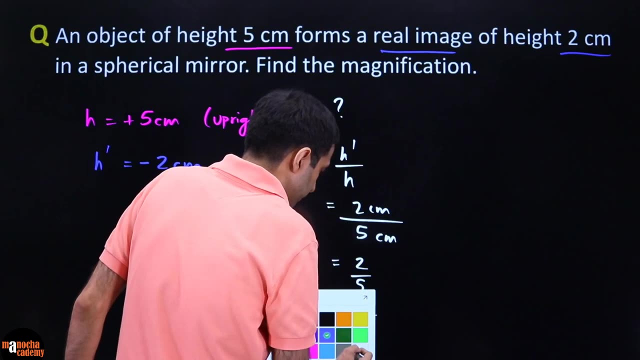 hundred. so you write profit is minus hundred. if you are writing profit, same thing over here. so now, when you find the magnification on your, everything was correct here except this sign right. so this is plus, this is minus 2 centimeters. so see, this will be negative here. 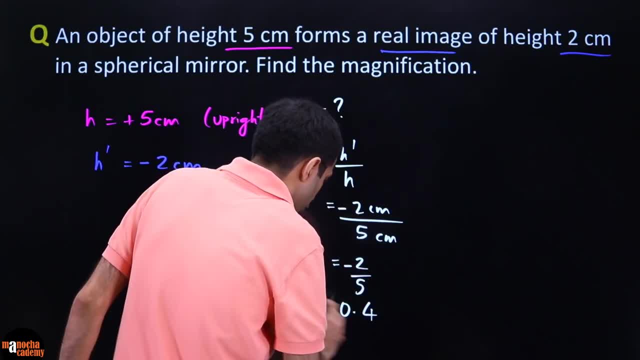 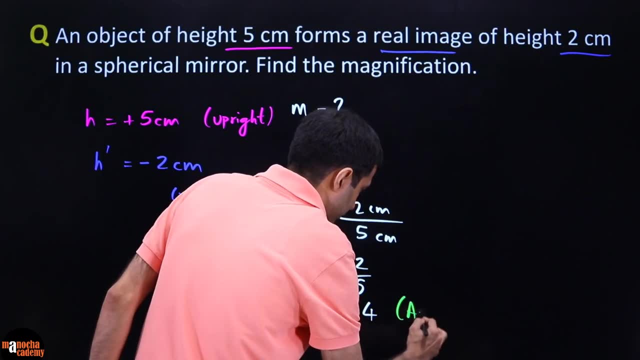 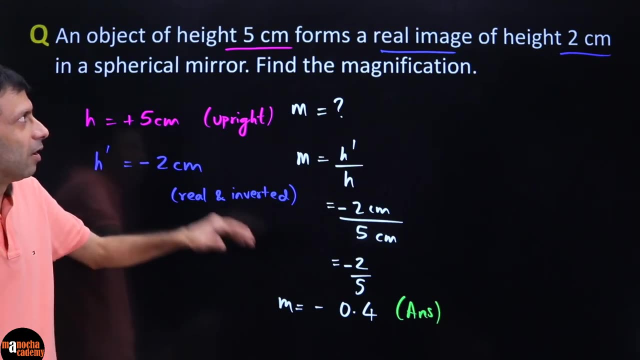 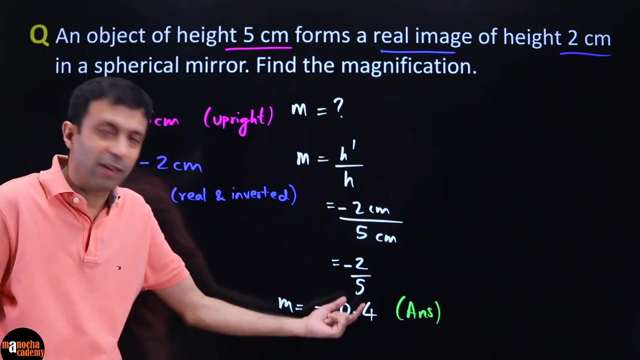 minus, and so magnification will turn out to be negative, very, very important. so your final sign is very important. minus 0.4 is the correct answer. usually we write it as decimal in physics rather than fraction. so what is the meaning of this negative sign? minus 0.4 is the correct answer. 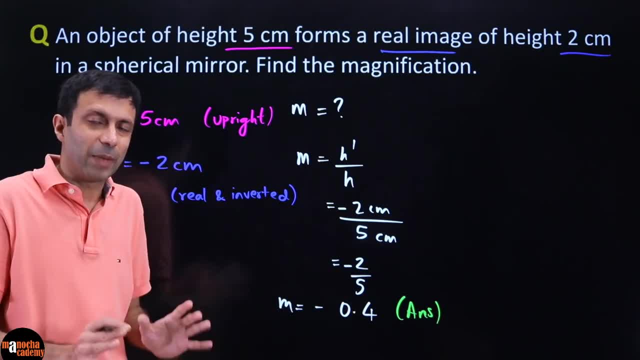 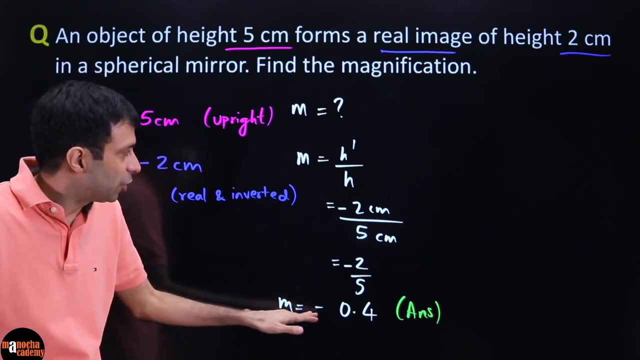 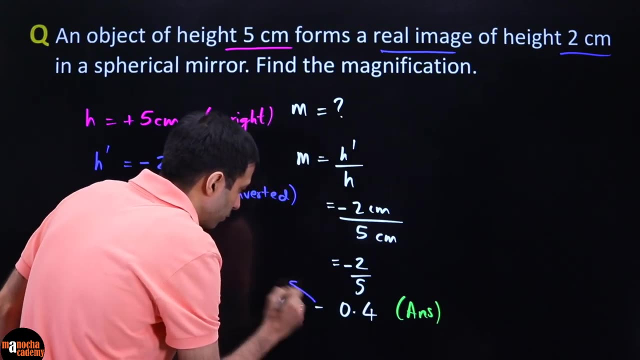 negative magnification. always, when we look at the magnification, number, divide the means, consider the sign separately and then the number. the negative tells you that it is an inverted image. so this minus part tells you, because there is a minus, means image is inverted. and since the number is, 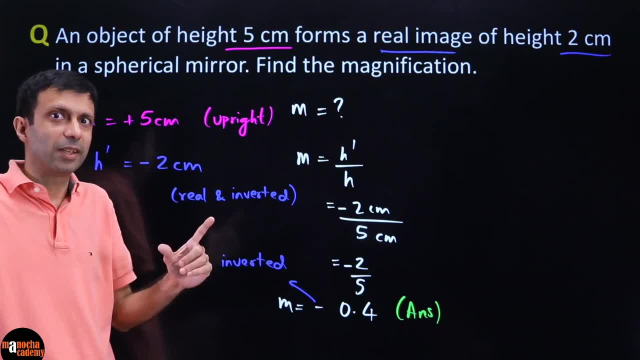 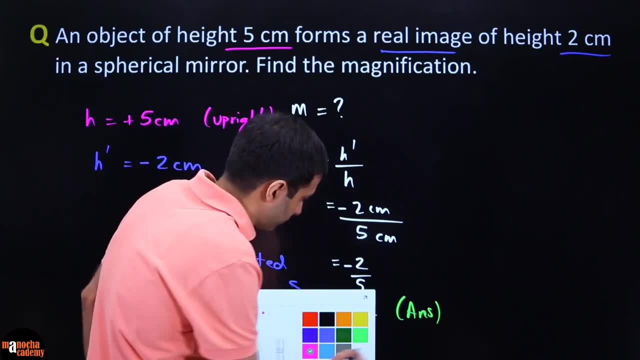 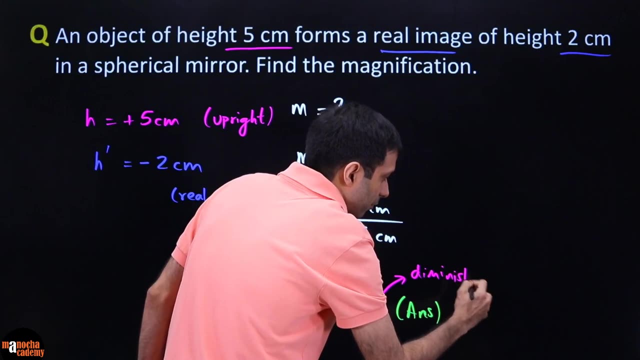 0.4 lesser than 1. that means what type of image it is, because magnification is of image height by object height. now, since the number is less than 1, this means it is a diminished image. size of the image is smaller than the object. that's why the ratio is 2 by 5, not 5 by 2. 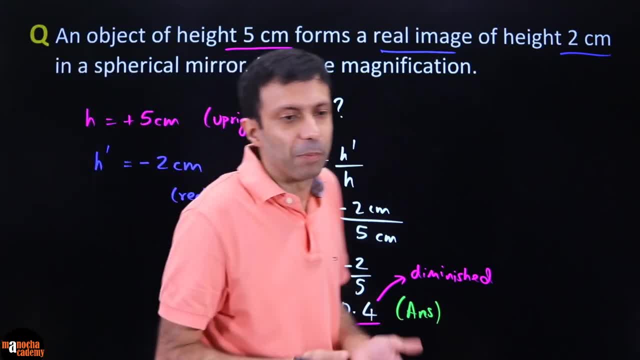 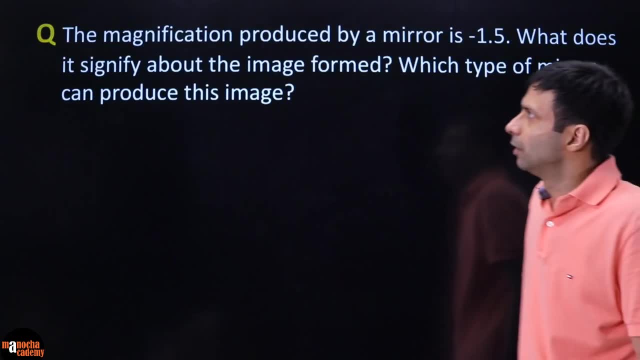 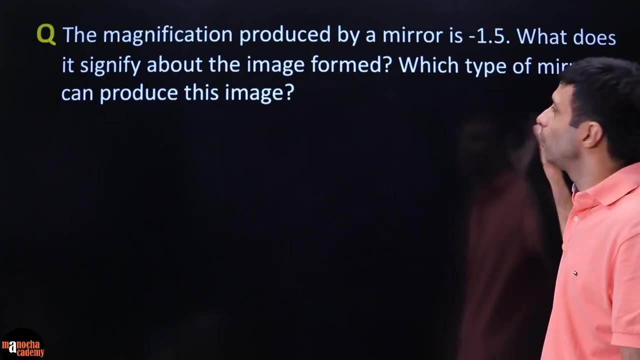 clear. so that's how you understand. that's the meaning of that final number minus 0.5. minus means inverted image, 0.4 means diminished image. next question: the magnification produced by a mirror is minus 1.5. what does it signify about the image formed? which type of mirror can produce this? 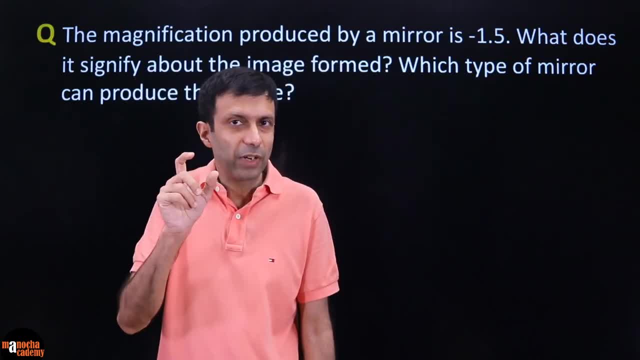 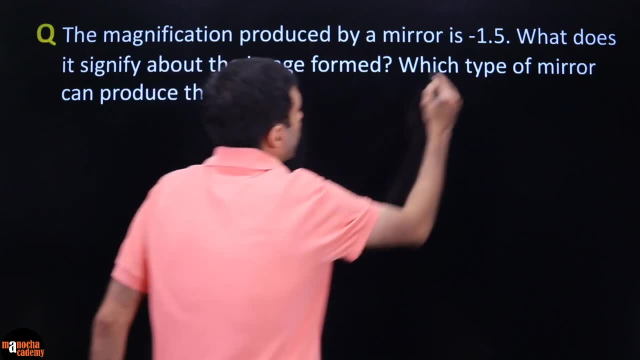 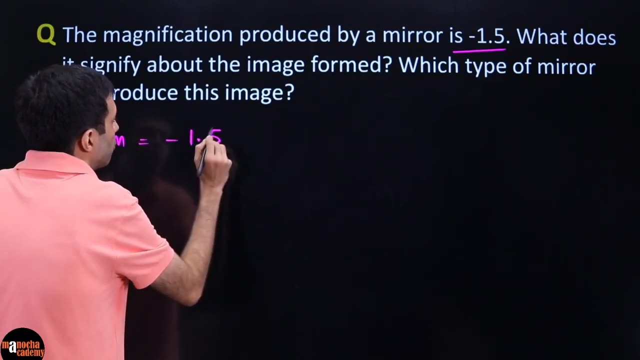 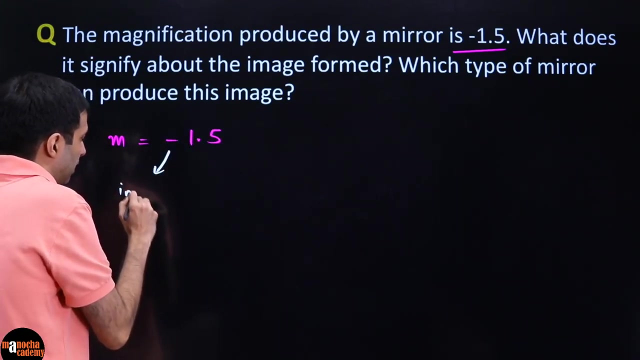 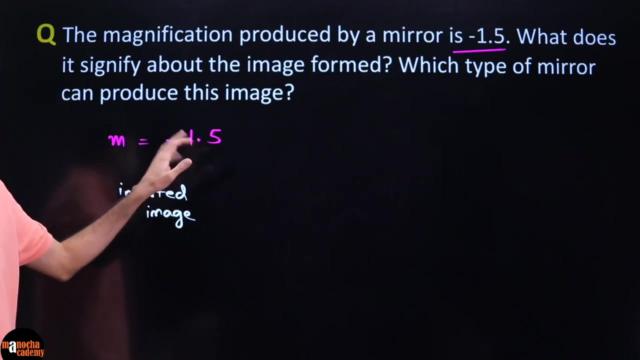 image. so, like we were discussing, look at that magnification number, break it down and try to solve this. so what have they told us? magnification is given as minus 1.5, so m is minus 1.5. so split it up. sign and number. negative means what it is: an inverted image: 1.5 or 3 by 2? what 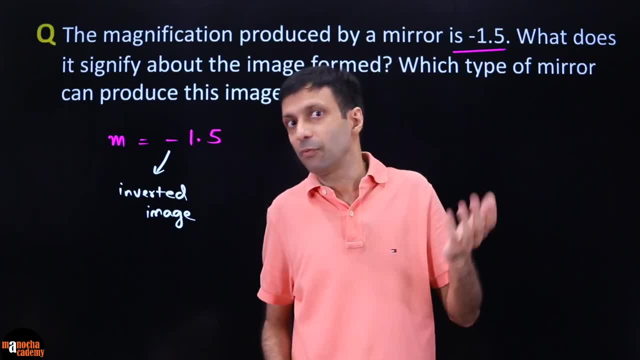 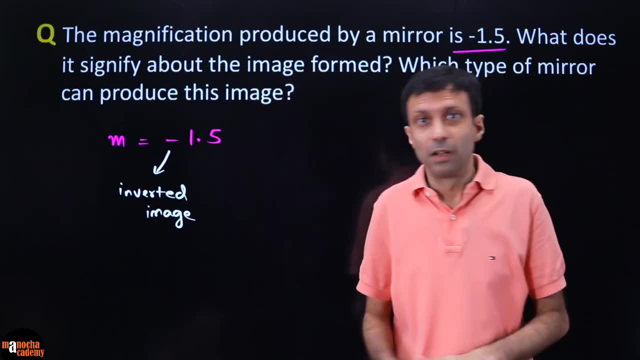 does this tell you about the size of the image? is it magnified, inverted or same size? what do you guys sorry, magnified, diminished or same size? what do you guys think? clearly it's bigger than 1. the ratio is bigger than 1. that means images than 1. 1, that is 1.5. that means there is a similar thing. 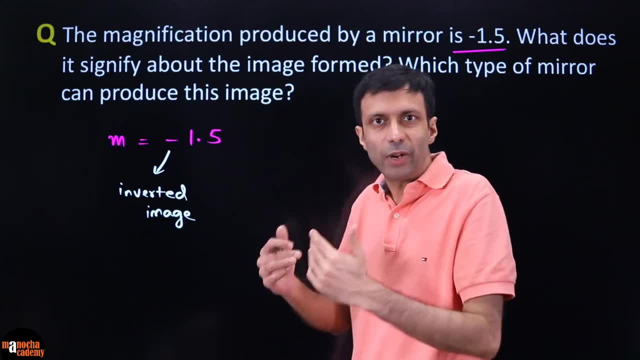 so let's say you want to separate this image by 4. you want to separate this image by 3. so you let's say you want to separate this image by 4. you want to separate this image by 4. you want to separate is bigger than the object because it is a ratio right, image by object. so if that ratio 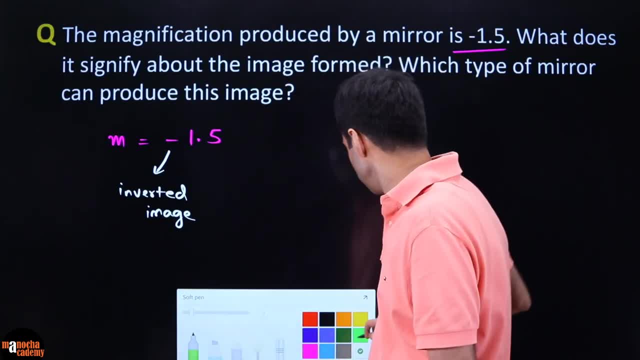 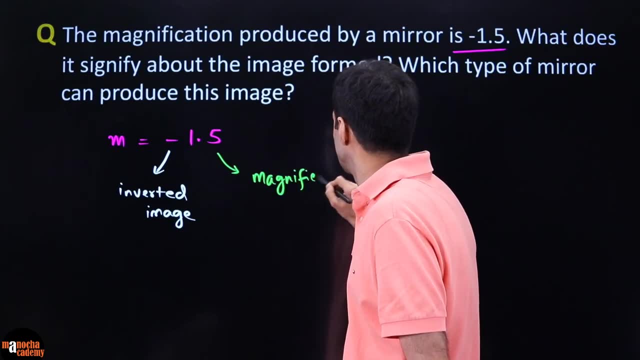 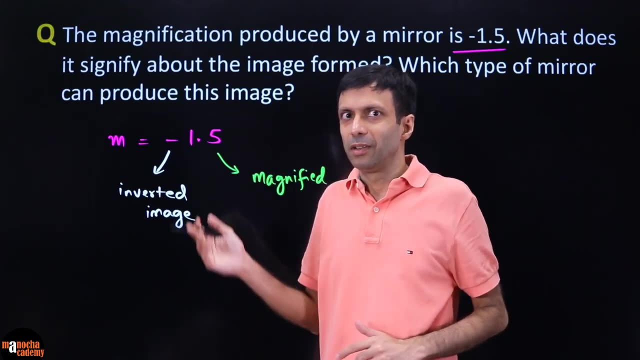 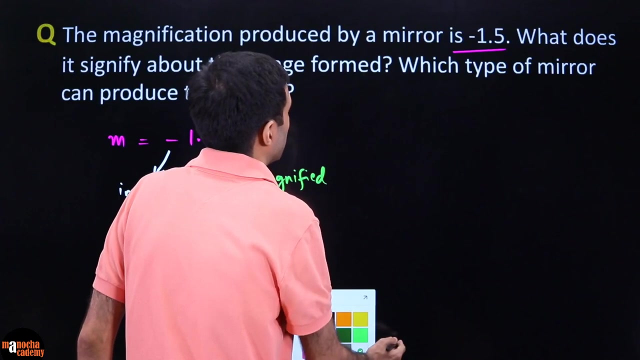 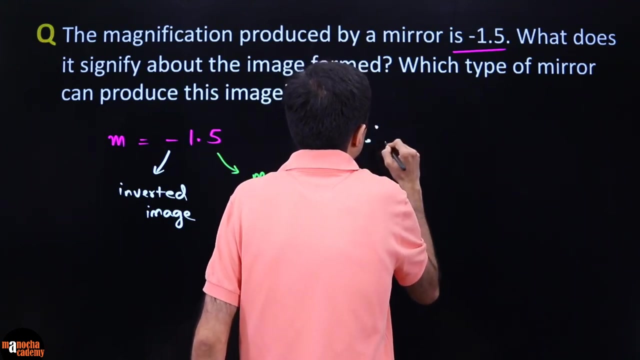 number is bigger than 1, clearly it is magnified. so we can clearly say it is a magnified image because it is inverted. what type will it be? real or virtual? inverted means the right answer is: it will be a real image. so what does it signify about the image? we can say, therefore: image. 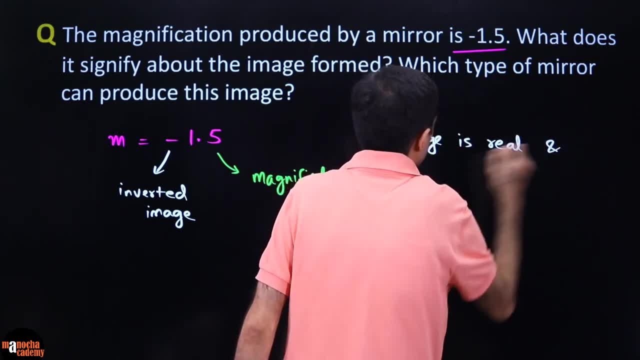 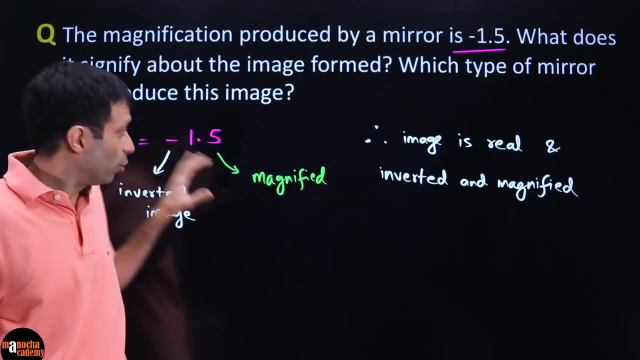 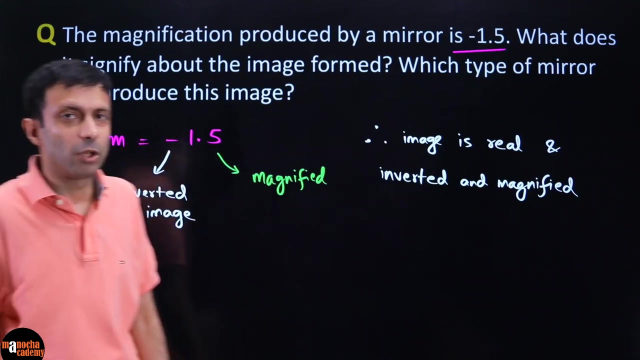 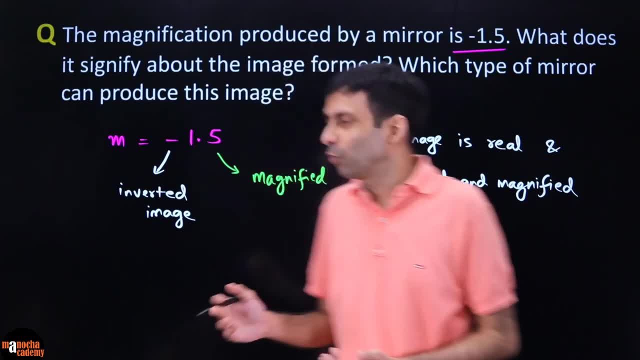 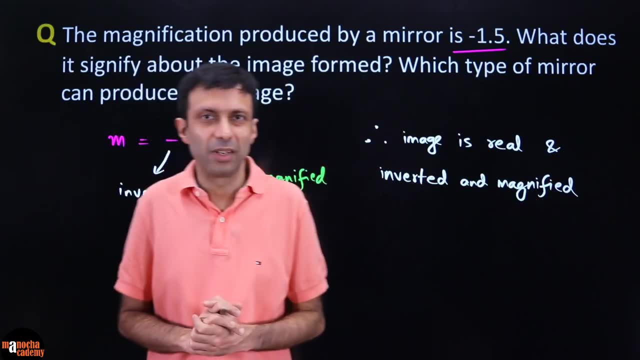 they may ask: plane mirror, you know, concave mirror, convex mirror. so which type of mirror will form this magnification? so very good, once again we get the clue, because negative magnification means it's a real image, inverted image, convex mirror never forms an inverted image. it never forms. 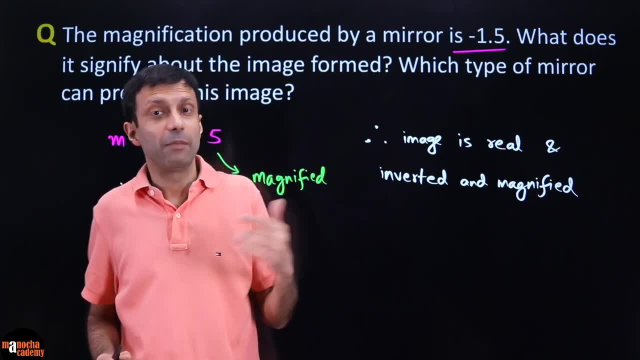 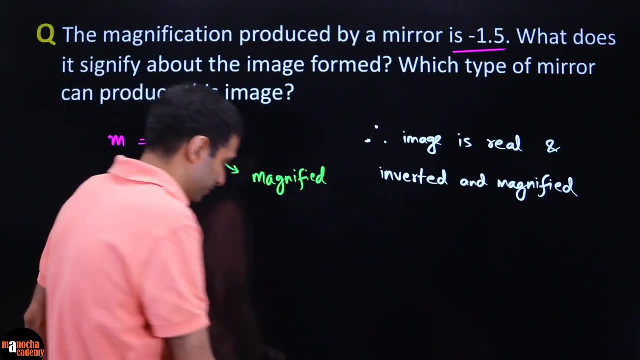 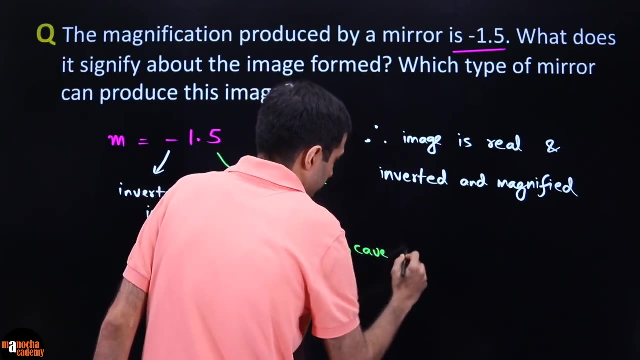 a real image. so definitely this has to be concave mirror. and concave mirror produces magnified image. convex mirror: it's always diminished. so both things are telling us definitely it's a concave mirror. so answer is concave mirror. and please think carefully sometimes, you know you're. 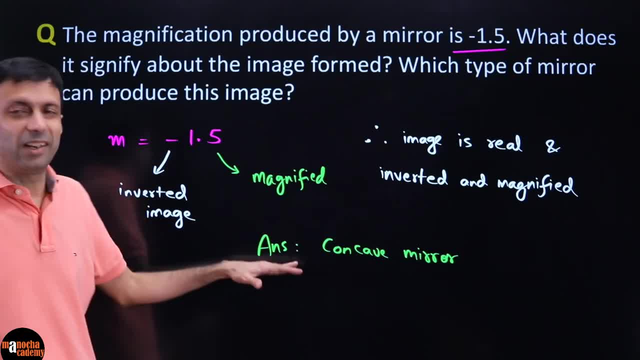 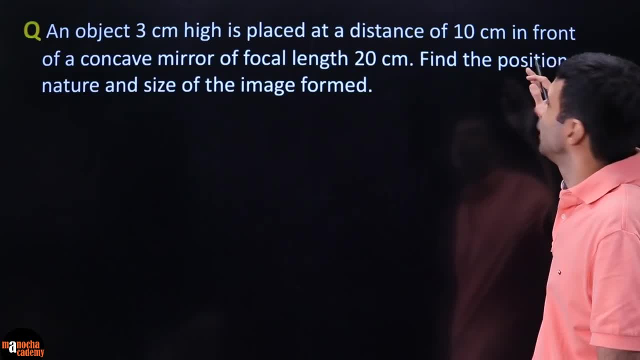 thinking concave, but right now you're thinking concave mirror and you're writing convex or thinking the opposite. clearly it will be a concave mirror here. next question: an object three centimeters high is placed at a distance of 10 centimeters in front of a concave mirror of focal length 20 centimeters. 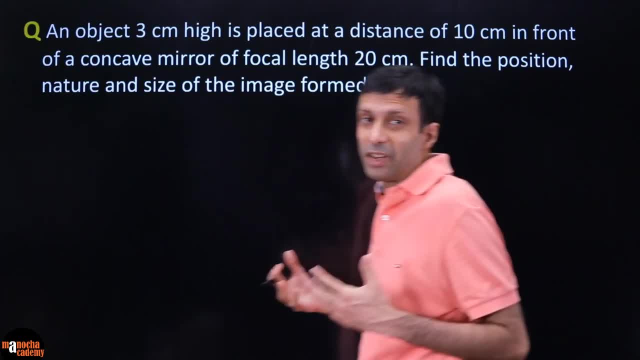 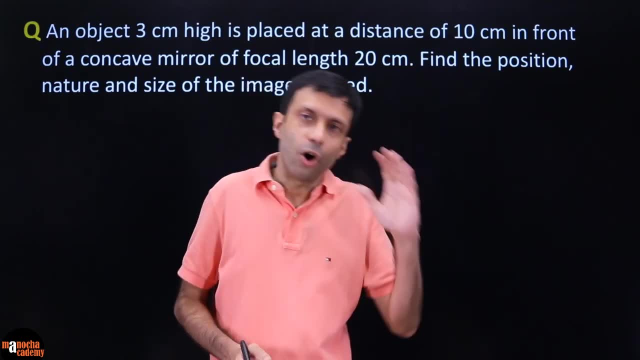 find the position, nature and size of the image form. so now the real sums are coming, because those sums are very simple. you know they were just magnification based, formula based. right now it's really coming that you know object distance, image distance, you know finding those kind of things, so that 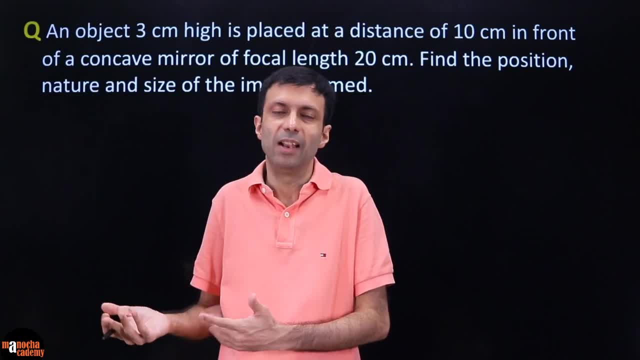 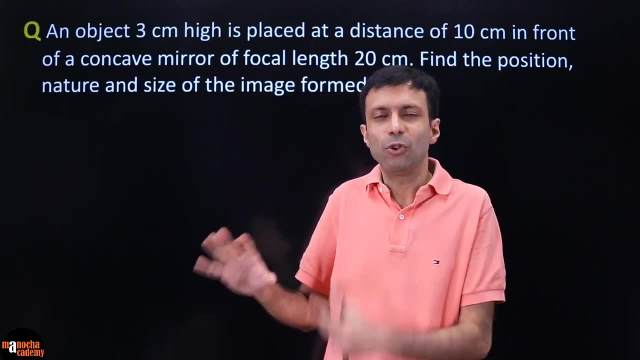 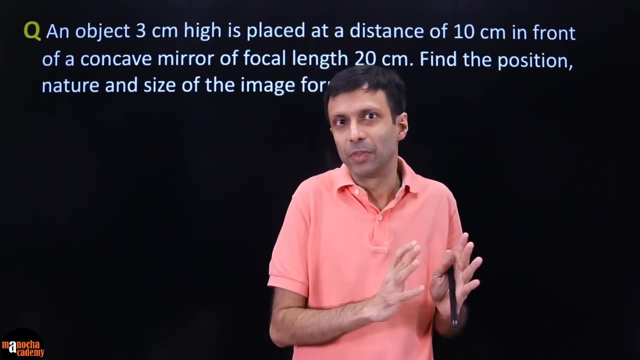 means we have to use maybe mirror formula or magnification formula as well. so now let's see how to solve this and what is the simple trick here, rather than, you know, just directly applying formula and doing something. first important trick is the dad trick. what is that trick? draw a diagram, or rather draw a rough diagram, because 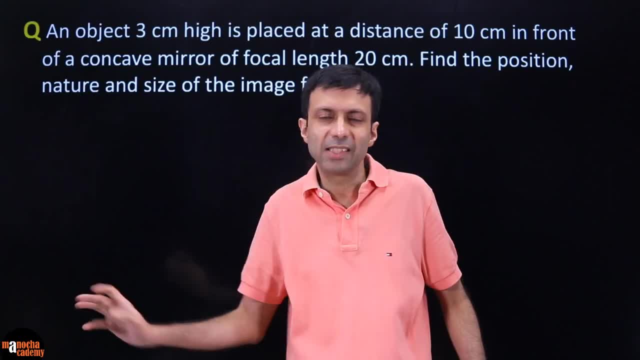 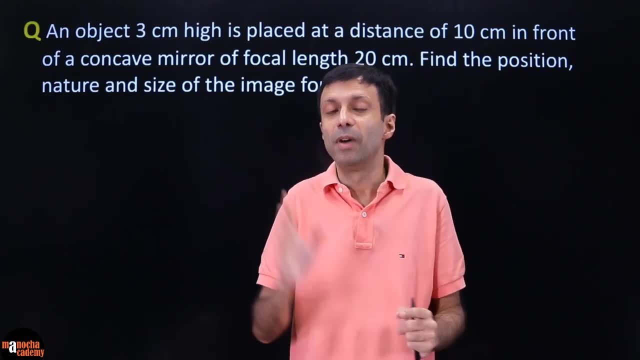 you have not been asked to draw a perfect ray diagram. you know, with all the rays and all of that. that was done in a separate class. so, first thing, draw a rough diagram, because that will help you visualize the problem and that will help you check the signs, because remember all these- 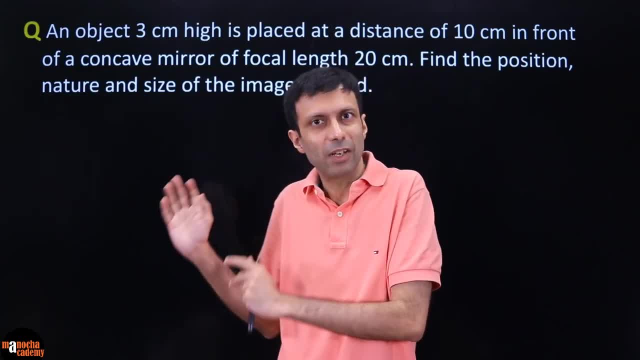 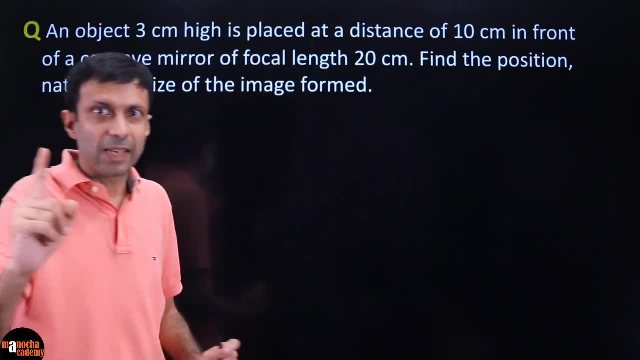 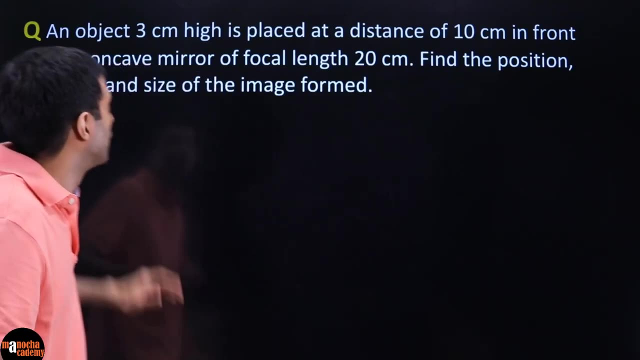 numbers, UVF. we have to write with correct signs, just like we did with magnification. one sign mistake gone. so you don't want to do that, okay. so first step, all of you, please promise me, let's draw a rough diagram. don't jump into the well, don't jump into the sum, okay. so what is the? 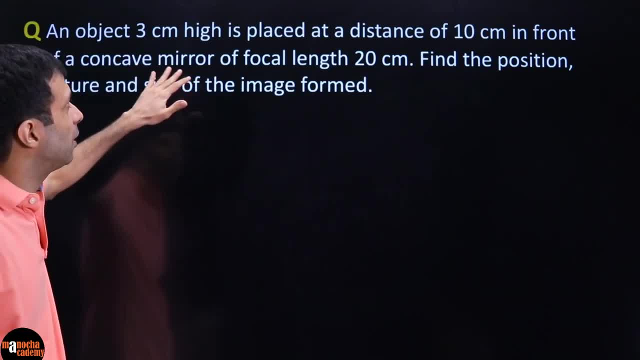 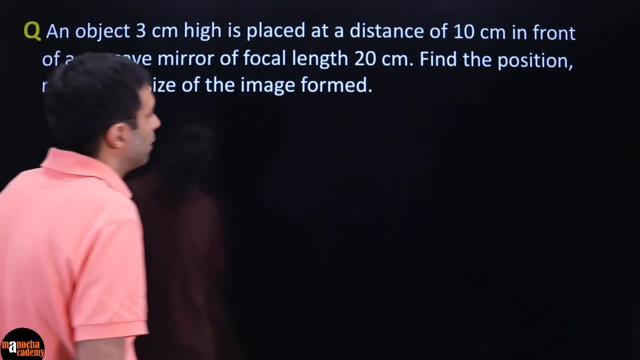 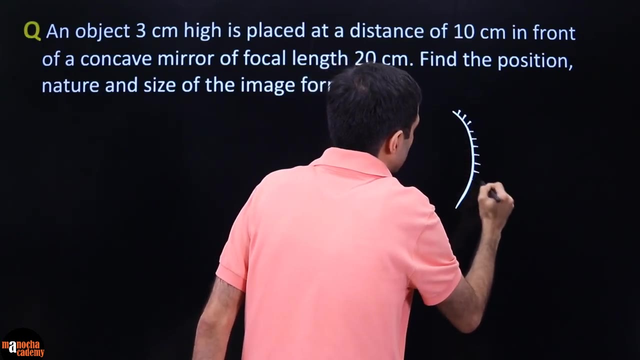 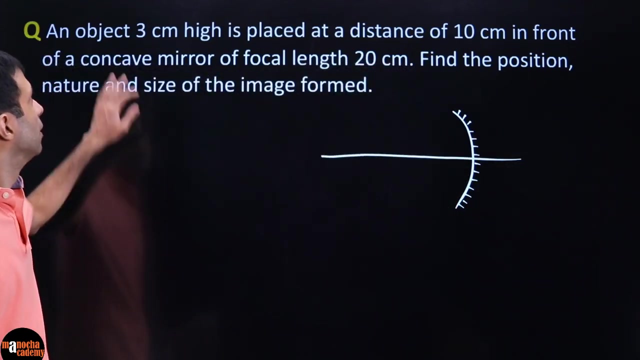 thing given here. let's look at the data. it says: okay, there's a concave mirror, some things are given, so let's draw a rough diagram again. it's rough, so let's go ahead and do a rough diagram here that we have been told there's a concave mirror and object three centimeters high is plated. 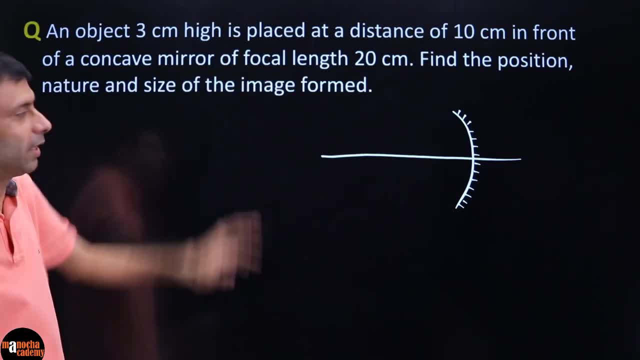 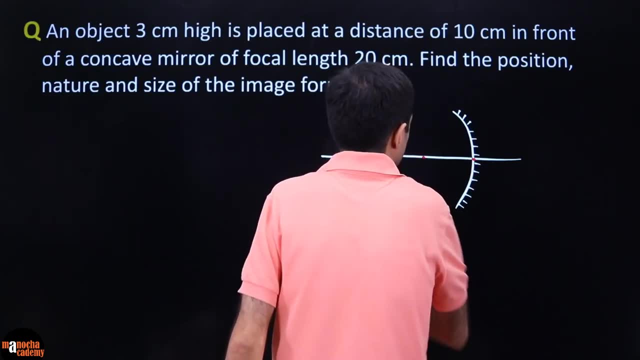 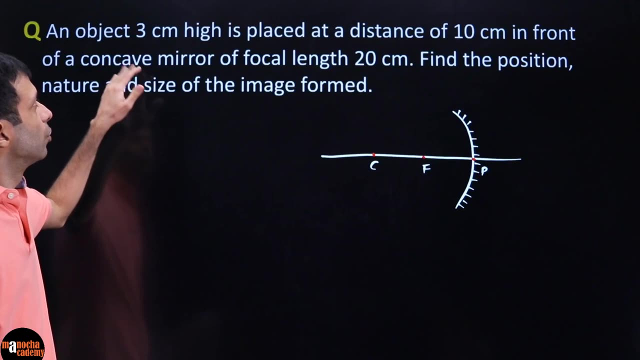 at the distance 10 centimeters in front of a concave mirror focal length 20 centimeters. okay, so here we can mark the pole focus, center of curvature. so it says the concave mirror focal length 20 centimeters. so let's mark that focal length. 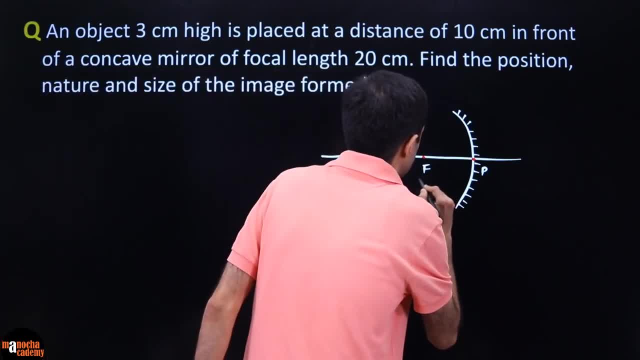 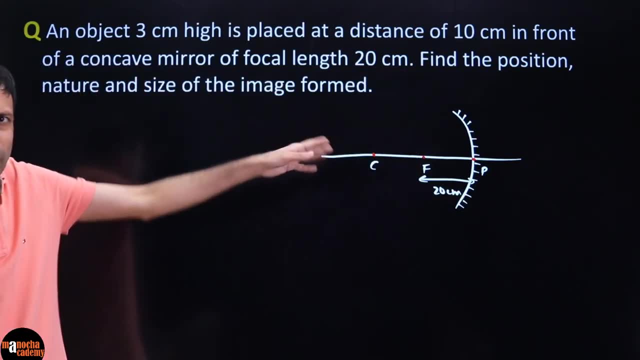 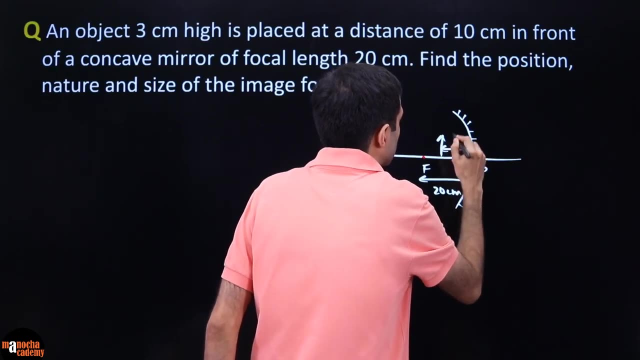 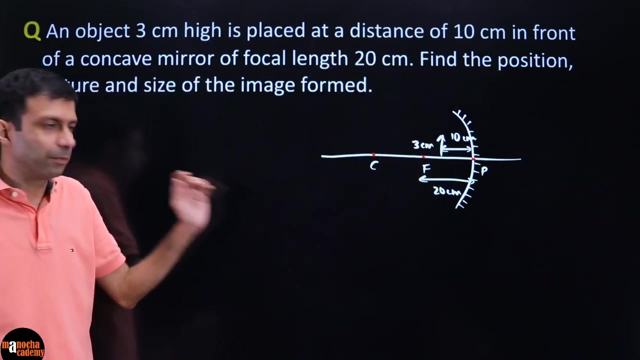 means distance from pole to focus. so this is given to us 20 centimeters. object is placed at a distance of 10 centimeters, that means between pole and focus. so somewhere here. object height: three centimeters- see again rough diagram. okay, now one very important thing: when 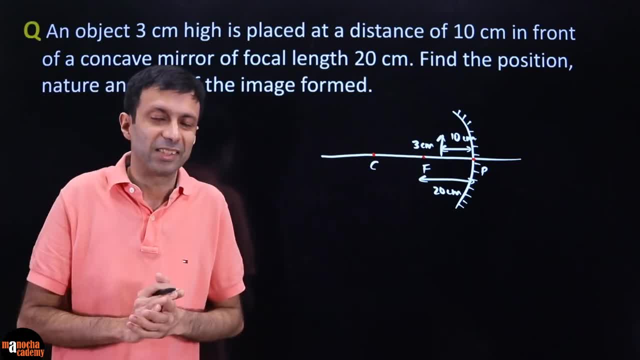 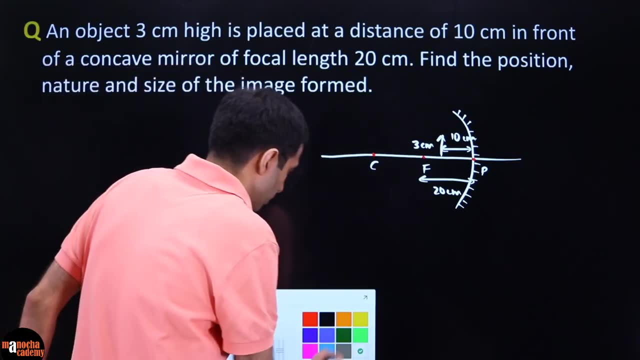 you draw the rough diagram. please draw that coordinate axis, that sign convention axis. i told you, otherwise you'll forget to take the signs. so please do that right now. so we are going to draw our x axis here. so we are going to draw our x axis here. 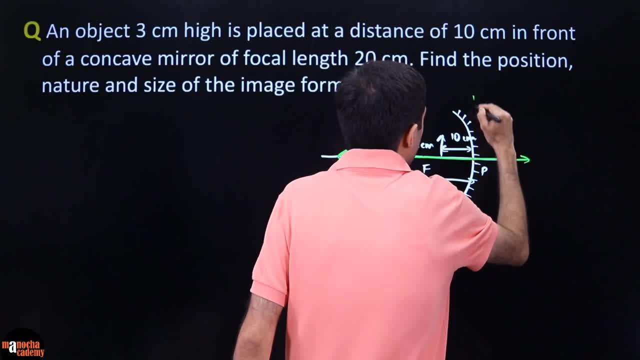 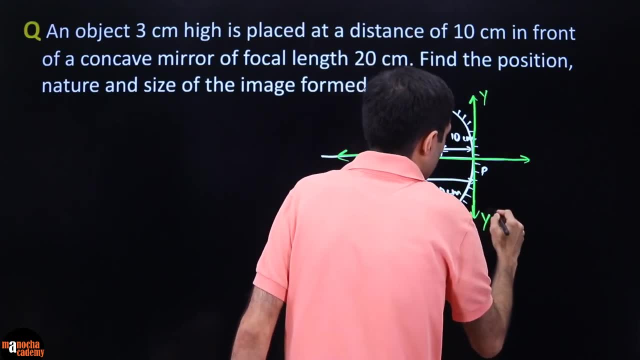 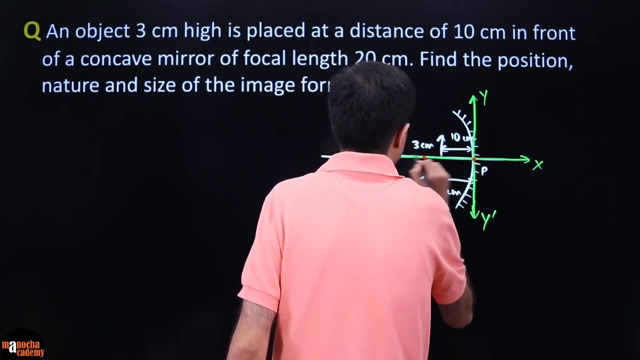 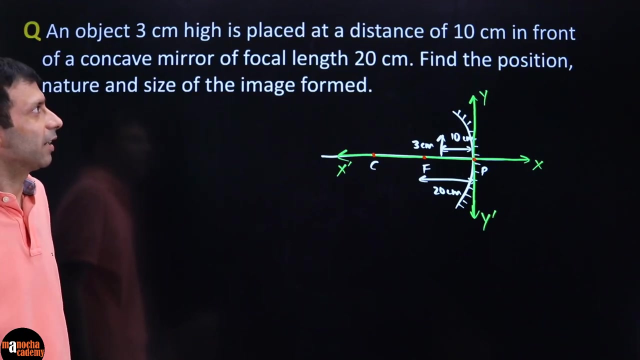 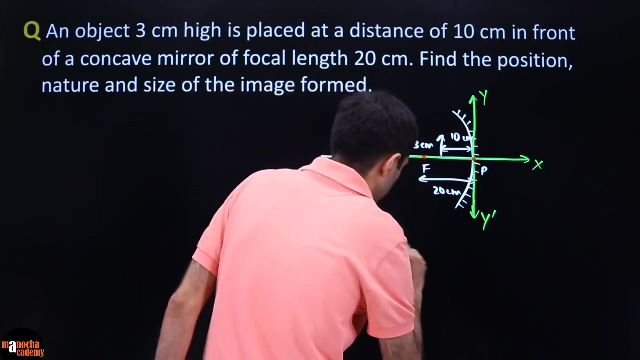 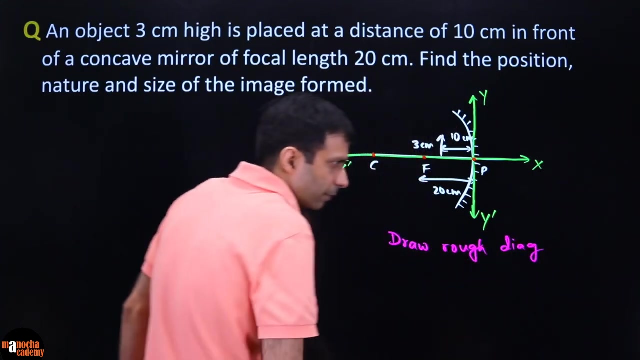 so we are going to draw our x axis here and the y axis. okay, so this will remind us to take all the distances and heights with the correct sign. so you have, has everybody done this? please draw the rough diagram equalằng. now let's past the final point. 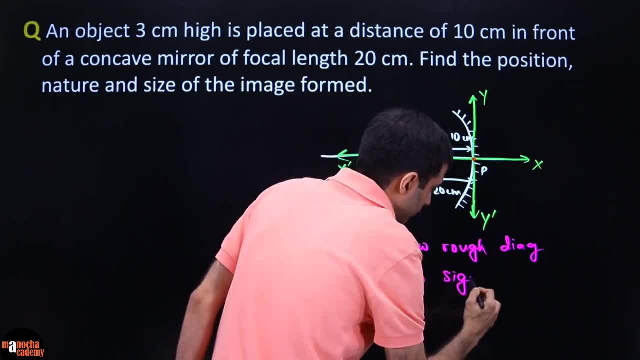 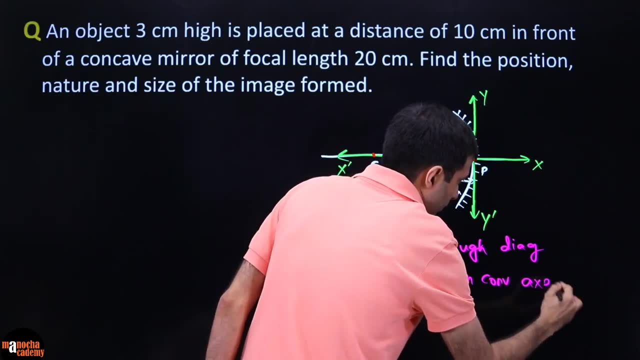 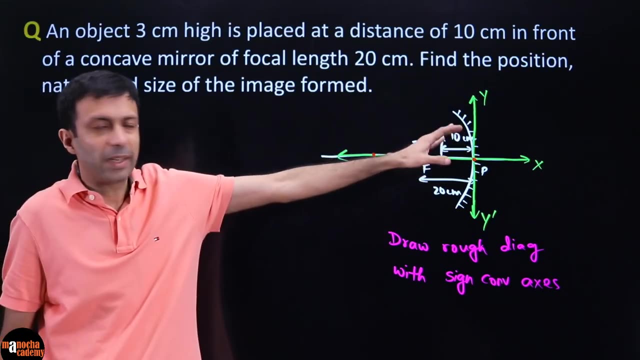 and with theta n, since theta is a music with this coordinate axis or sign convention axis, this sign WiFi. now let's write down the data, because here of you don't have to write the plus-minuses just for a visualization. plus-minuses, typical round table is just for a visualization work. please, the coordinate axis correct, brding я. 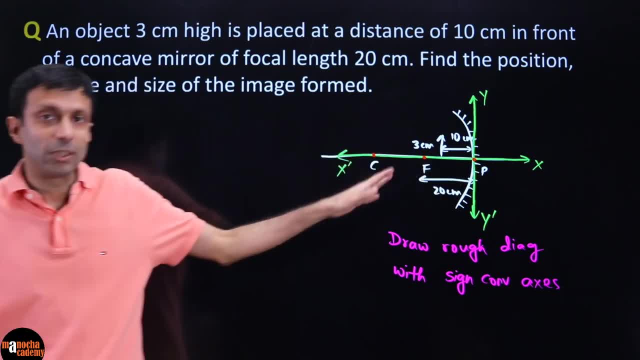 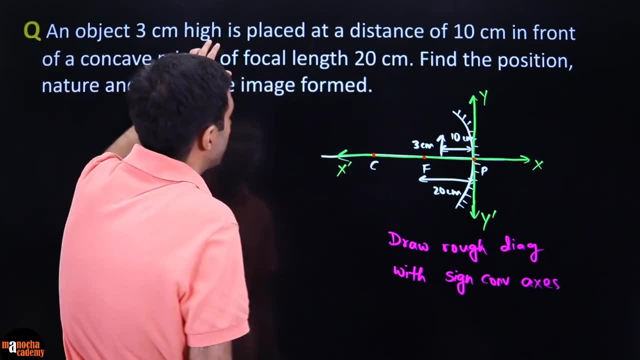 qi przekش procent. now we can think of the plus-minus based on this coordinate axis. so let's quickly write down the data here. so what is given to us? object 3 centimeters high. so everything you're reading you note it down in your data. so object height, that means this object height will denote it. 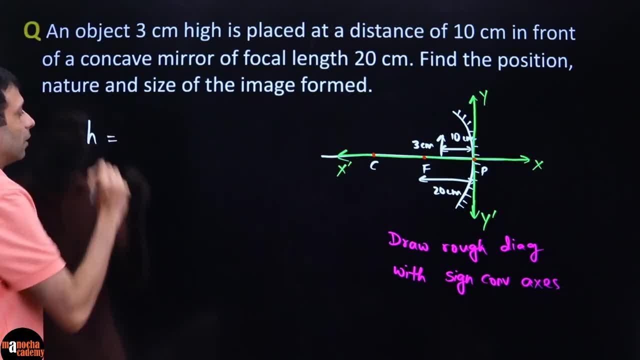 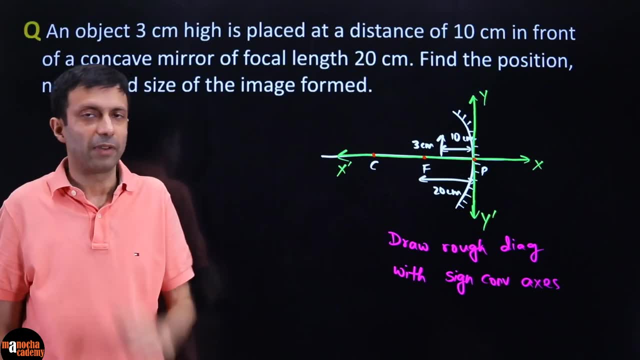 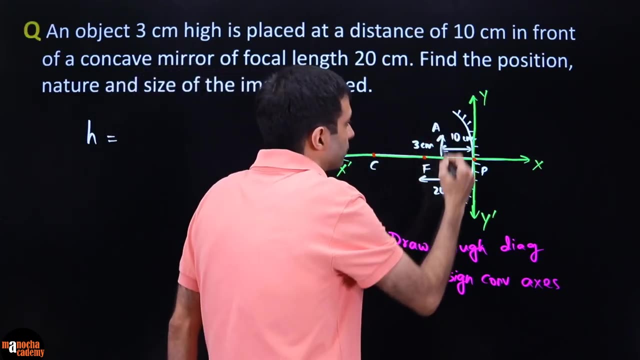 with capital, with H, it is 3 centimeters. should I take it positive or negative? based on our rough diagram? what should I take? positive height or negative height? what do you guys think? very good, clearly you can see the object is along the. if we call this object AB, it is clearly along the. 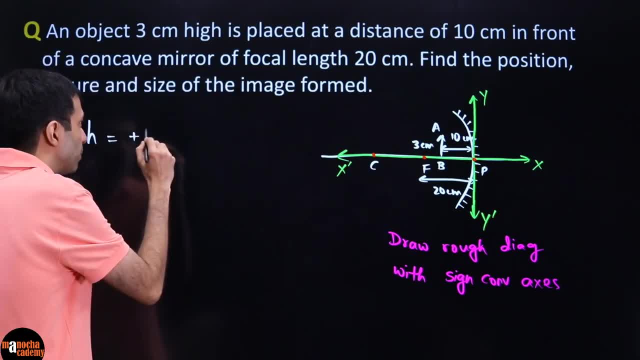 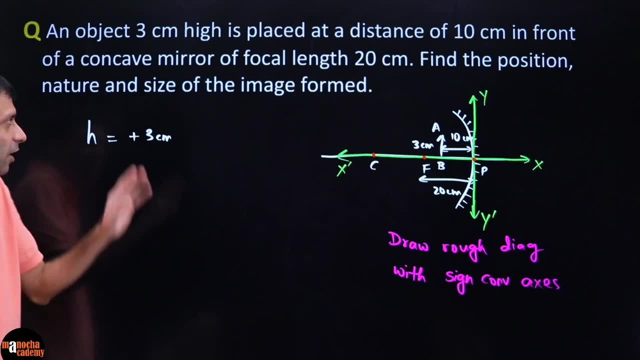 positive y-axis. so definitely object height and put this plus. I know it sounds silly to put plus, but it will remind you. hey, I thought of the sign. okay, I didn't miss the sign- plus 3 centimeters. so these are the tricks. you know that. don't miss out on any sign, otherwise you will miss out on the. 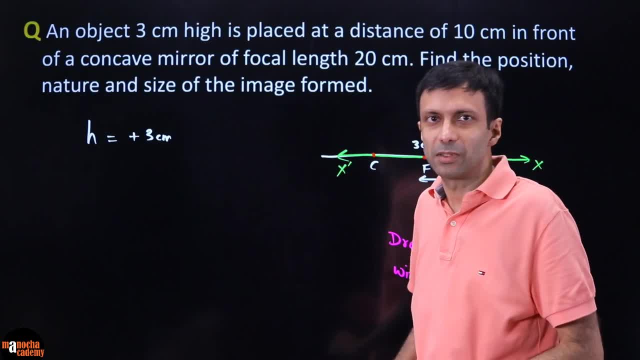 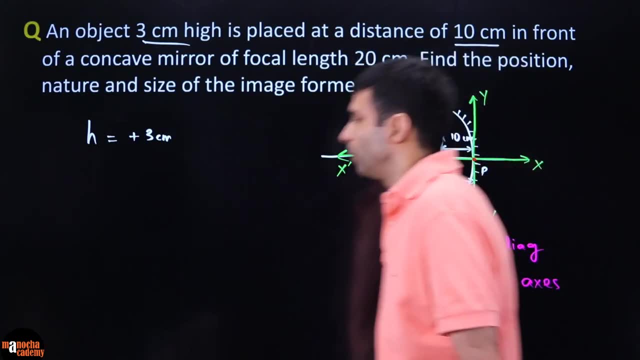 marks or your sum will go wrong. so plus 3 centimeters object height. next thing given, so this part is done. it is placed at the distance of 10 centimeters in front of the concave mirror. so when we look back here, 10 centimeters in front of the concave mirror, that means this is object distance. 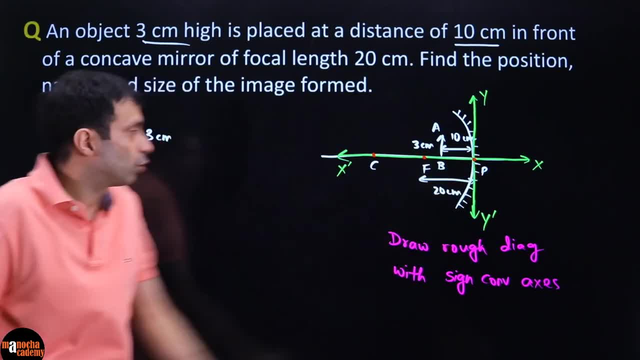 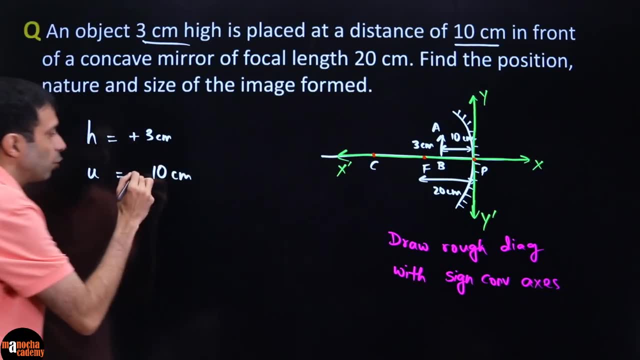 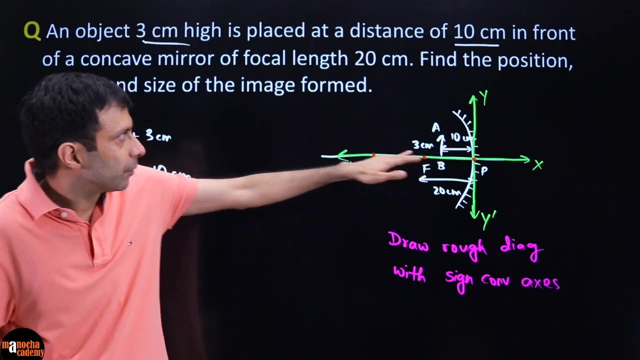 we are talking about the object. distances are measured from the pole, so object distance means you. that is the symbol of object distance: 10 centimeters. what sign should I put here again? keep thinking positive or negative, positive or negative? so according to this, this is clearly along the negative x-axis, simple. 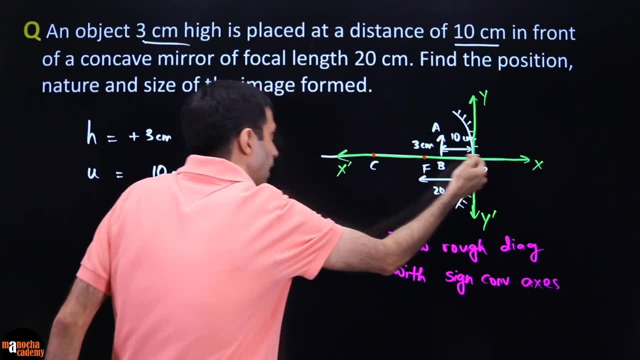 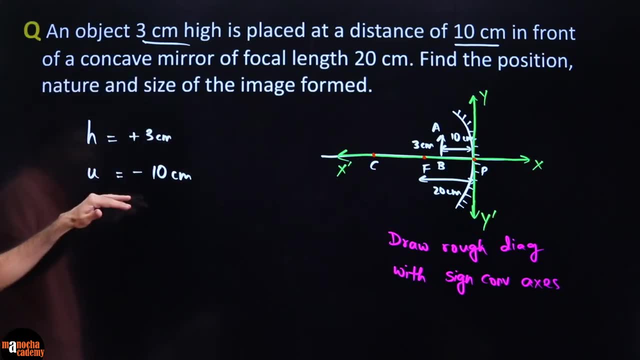 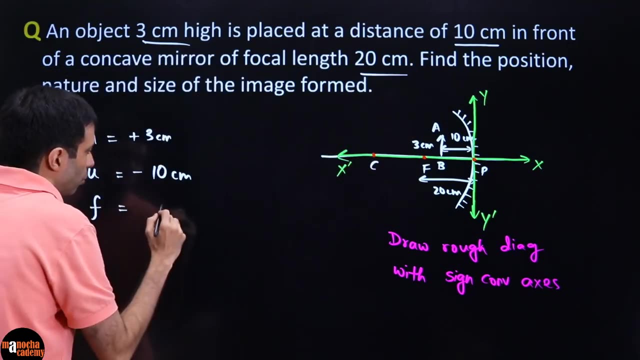 coordinate geometry. this is your origin in the pole is like the origin I am measuring from here, so it is along my negative x-axis definitely minus 10. okay, done, see. so we have done that. next let's look at focal length: 20 centimeters. focal length means small f: 20 centimeters. 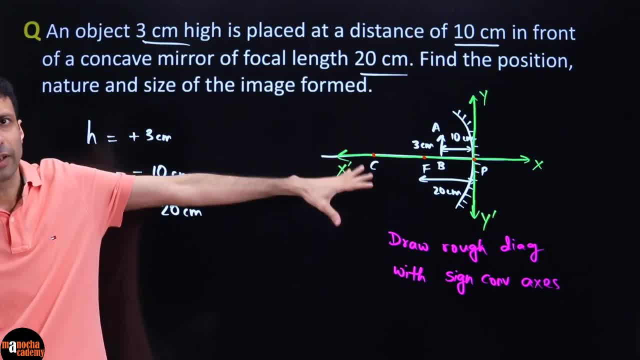 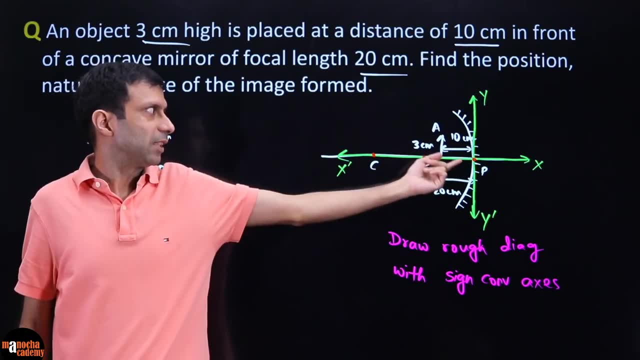 again, positive or negative. you don't have to memorize this. if you have this drawn in front of you, you will easily get the sign. so again, the pole is like the origin. focal length means distance from pole to focus. so is it along positive or negative axis? 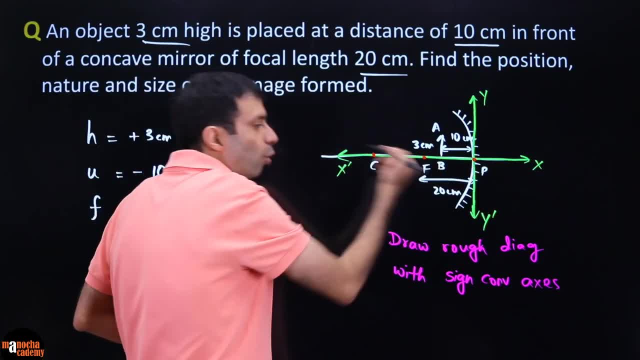 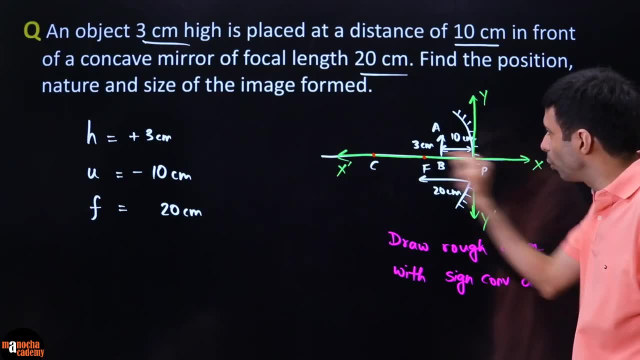 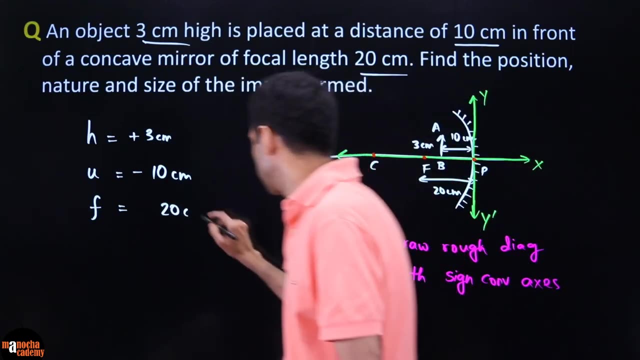 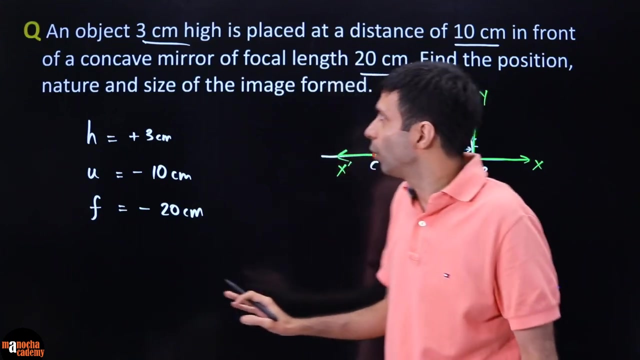 because, remember, you are not going from focus to pole, you are going from pole to focus. always you are measuring from the pole, always you are measuring from the pole, pole to focus. very good, negative x axis minus 20 cm. so is everybody comfortable with this data? so we have noted what all we want. 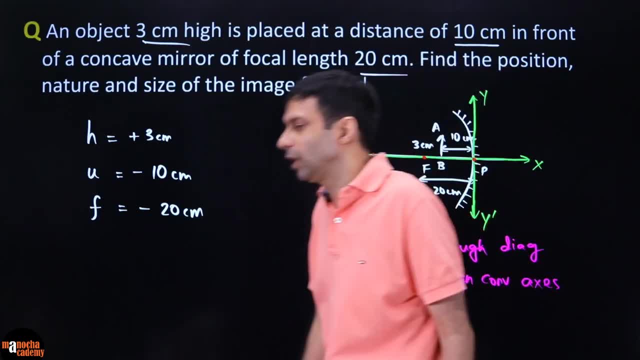 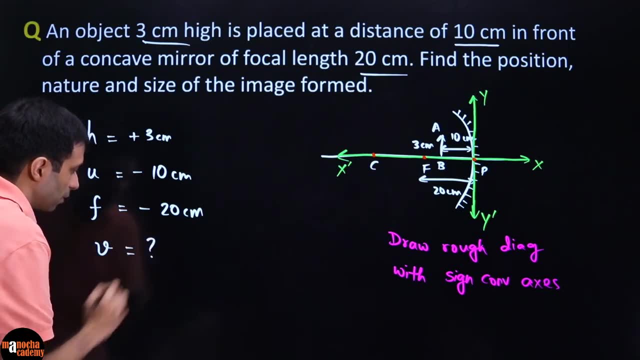 and then it says what? find the position, nature and size of the image form. so what do we need to find here? position means we need to find the image distance, so that is unknown. size, which means we need to find the image height, again unknown. so you can put a question mark. 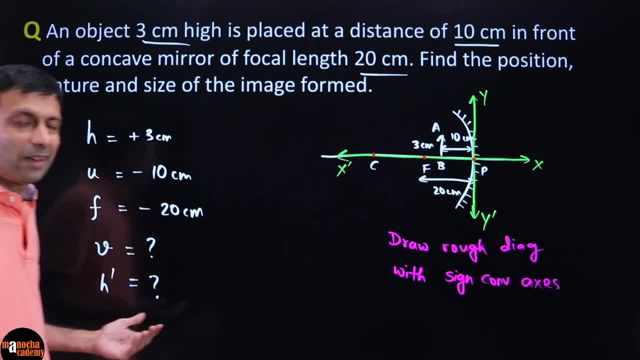 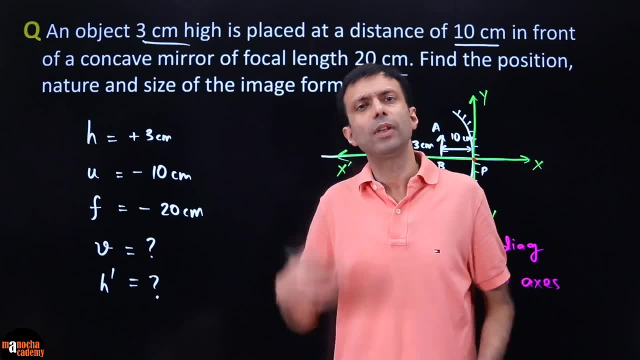 so, for the ones that are, for the things that are unknown, do I need to worry about the sign? do I need to write plus or minus here? no, it is not. no, it is just like mathematics: unknown is x. we don't think plus x or minus x. 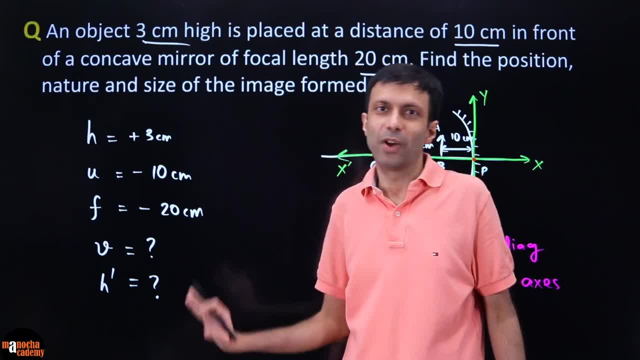 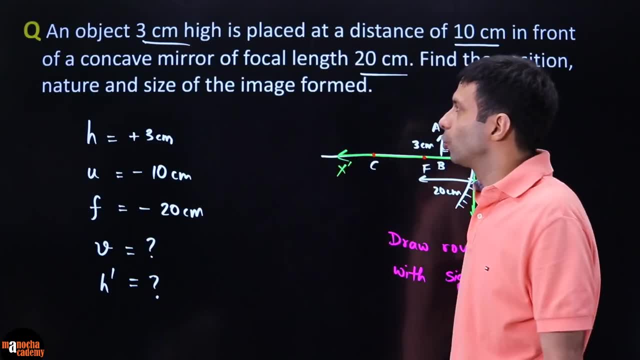 we just write ok, unknown. so here you don't have to worry about the sign, but the things which you are writing, the data that is given. you have to write positive or negative. so let's go ahead and work that out and, based on you know these properties. 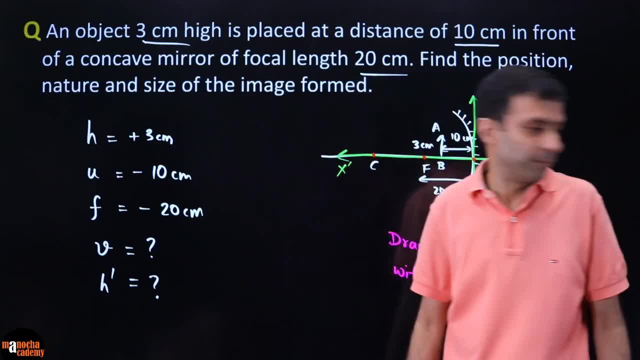 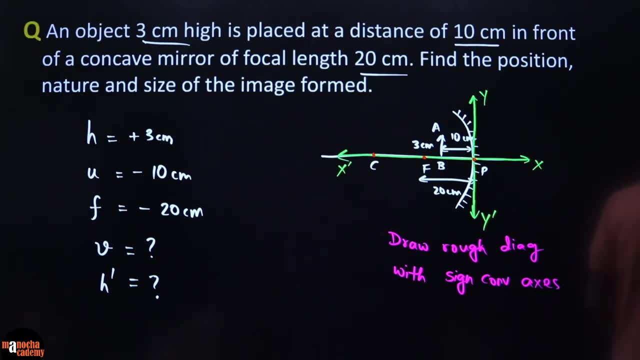 we can guess the nature of the image. is this crystal clear to everyone? are you guys all clear about this? so please note this down. please draw the rough diagram. I don't want anyone being lazy or taking shortcuts. please practice it this way in my classes and when you are doing it. 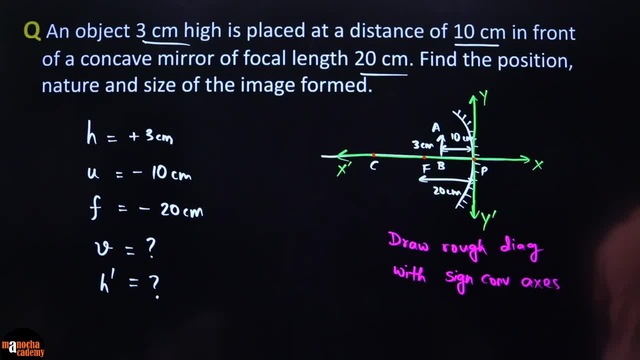 trust me, you guys will get your questions correct. everybody, everybody, don't be lazy. please pick up your pen and paper. now you have got this. now you know that, ok. so everybody, please write down the data like this: you will get the sums right. trust me on this. 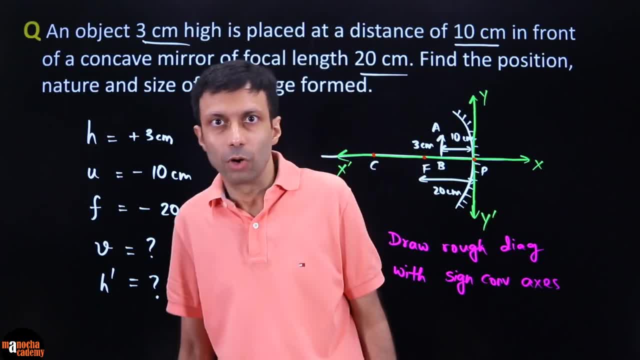 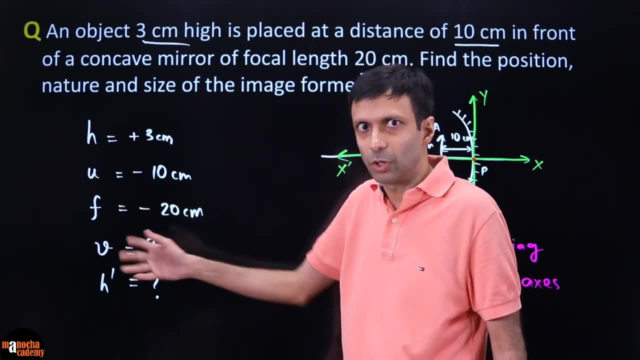 now let's go ahead and write down the mirror formula or whatever magnification formula. so most probably we need mirror formula here. why F and U are known, V is unknown. ok, so let's write down our mirror formula, plug in these numbers and solve the question. so there you can see. 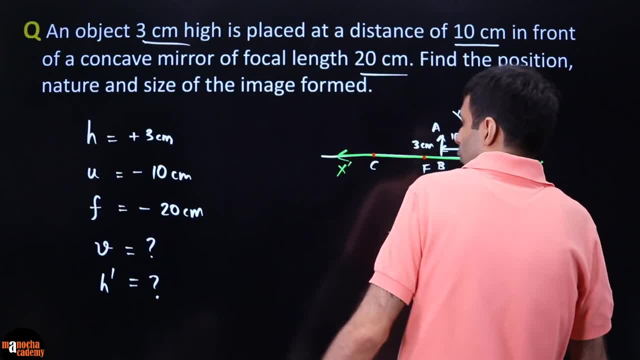 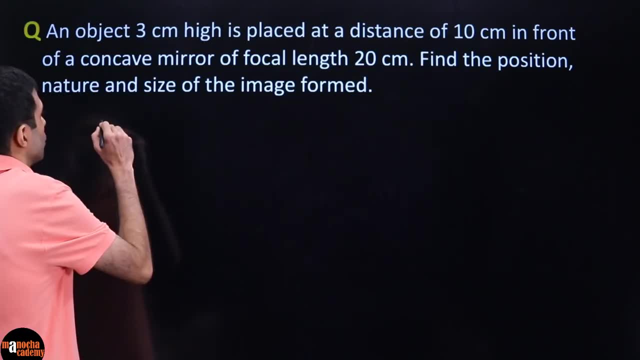 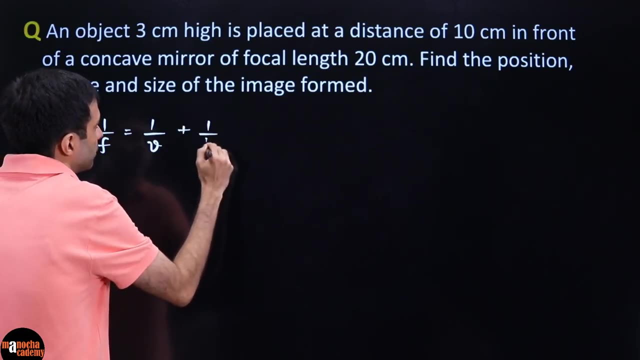 we are going to write the mirror formula for this guy, so we have already drawn the rough diagram here. the rough diagram is already done for us. so mirror formula is: 1 by F equals 1 by V plus 1 by U. ok, and so focal length. we saw. 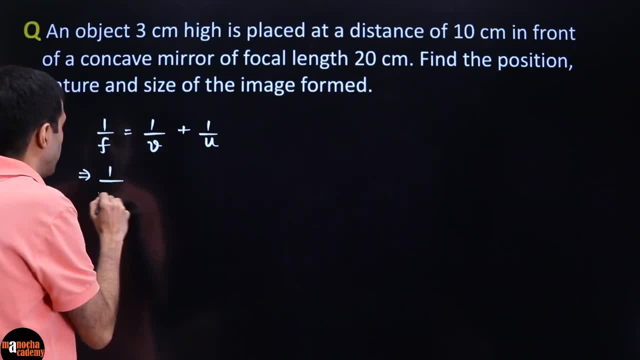 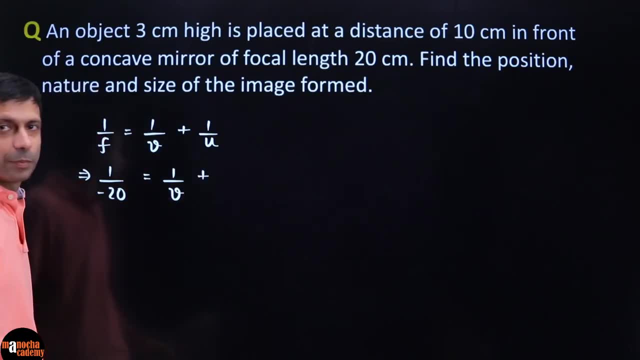 was on the negative x axis, so focal length was minus 20, the image distance we need to find. so that's our unknown and object distance. remember we took it as minus 10. so that's it. you just have to solve this equation, which means you have to solve for V. 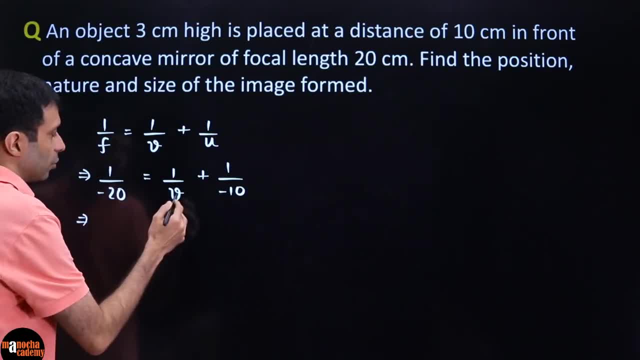 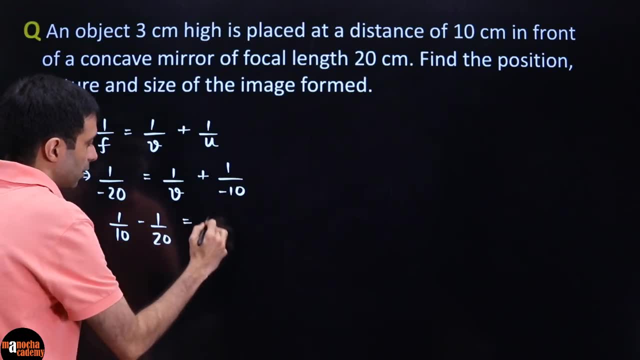 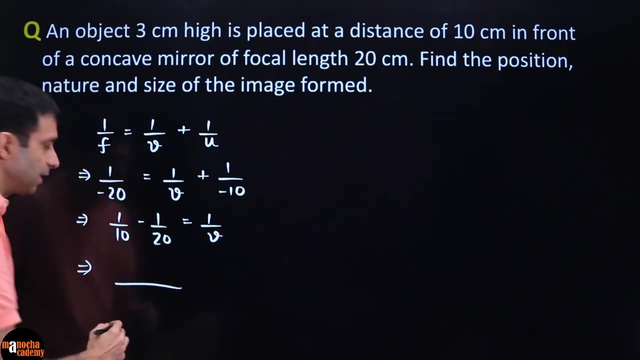 so please go ahead and do that so we can bring the 10 over here. so 1 by 10 minus 1 by V plus 1 by U, 1 by 20 is 1 by V. so please take the LCM over here. 20 is the LCM. 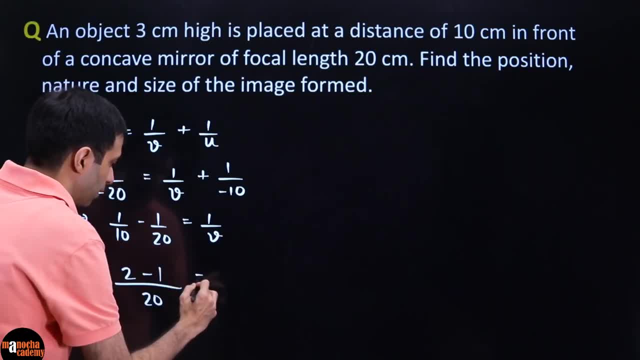 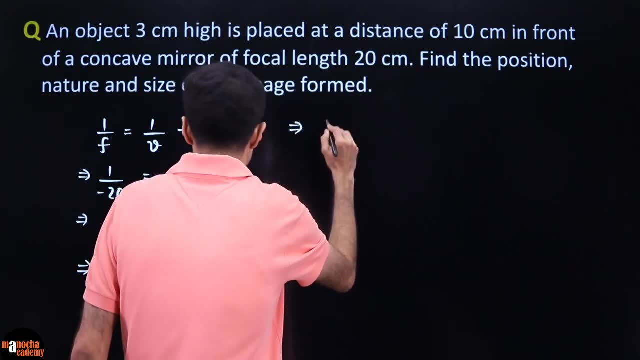 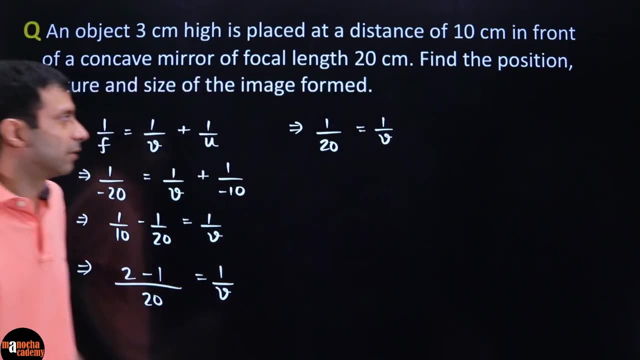 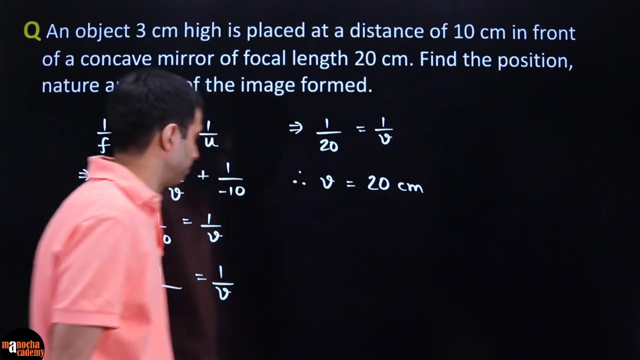 2 tens are 20, 2 minus 1, so this is 1 by V. so therefore, what do we get here? 1 by 20 is 1 by V. so what is the image distance? 20 centimeters, all of you got this: 20 centimeters. 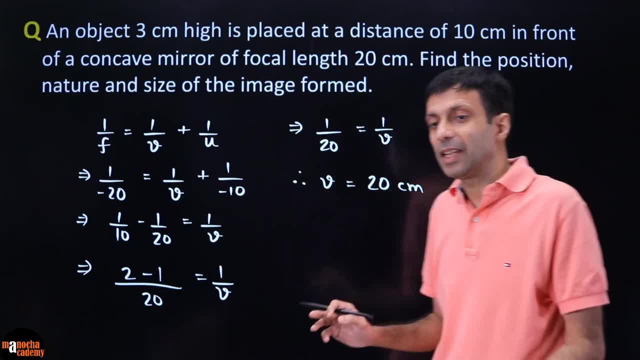 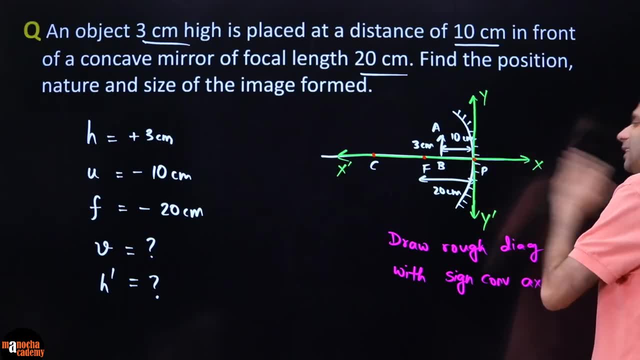 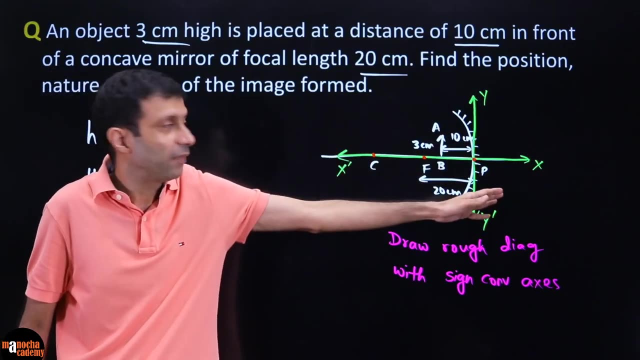 now, is it positive or negative? positive, which means image is formed. if you go by the sign convention, image is formed along the positive x axis. and did we expect that? in this concave mirror, did you guys expect the image to be formed in the positive x axis? 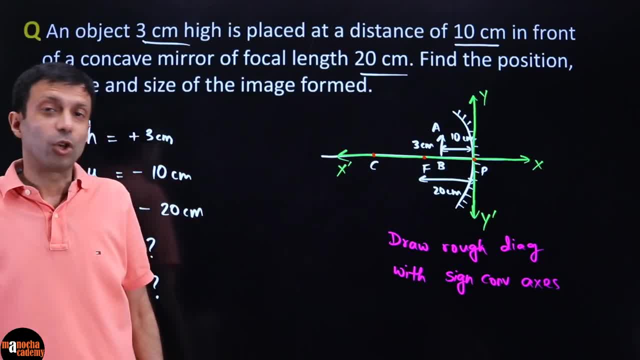 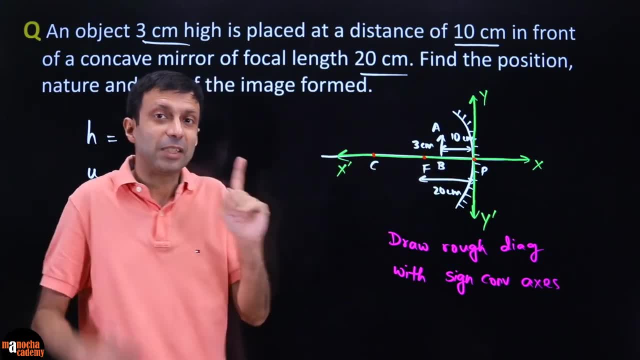 which means behind the mirror, yes or no? tell me, because clearly you can see. what case is this? where the object see without solving the object is between pole and focus. that means this is shaving mirror case, or make up mirror so we will get a magnified image. 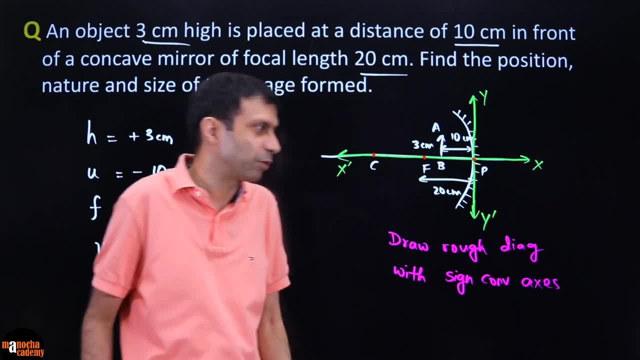 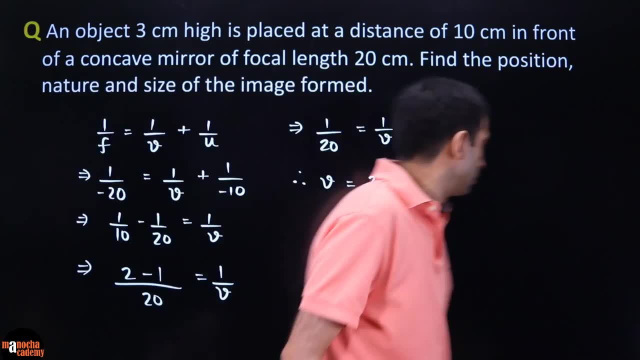 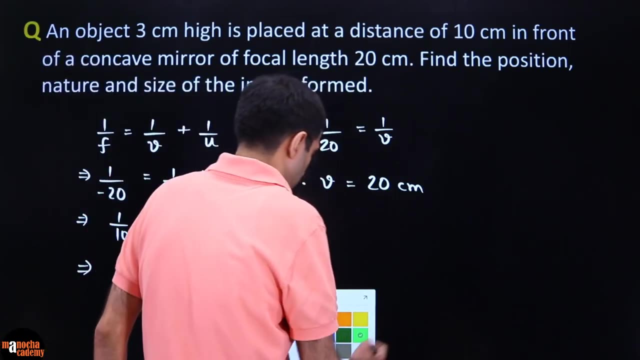 which will be behind the mirror. so it looks absolutely right that the- because the object was placed between pole and focus, image will be formed behind the mirror. this answer, at least, is making sense right. so we have found the, we have found the image position, so this one is done for us. 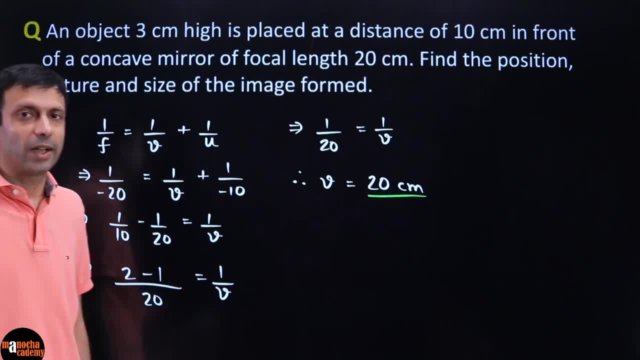 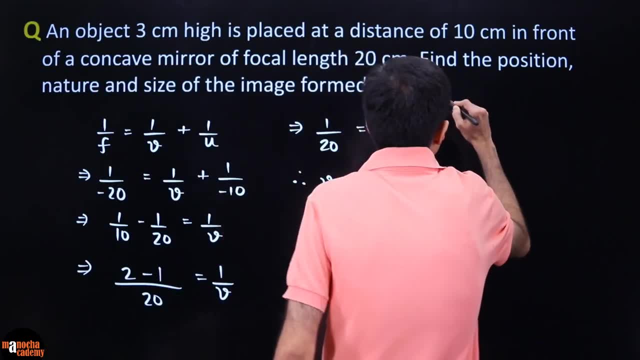 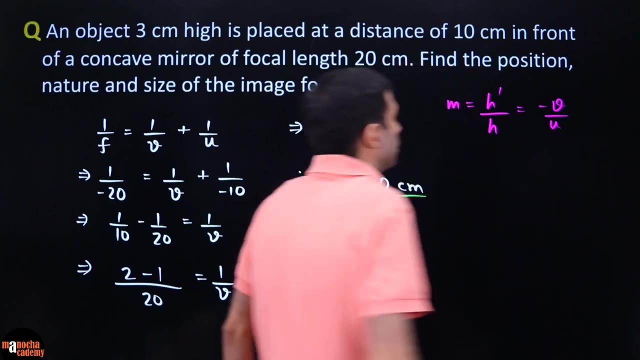 now we need to find the size of the image. how do you find the size? using magnification formula. magnification is h dash by h. so magnification h dash by h is minus v by u, remember. so let's go ahead and find the image height. so image height is unknown. 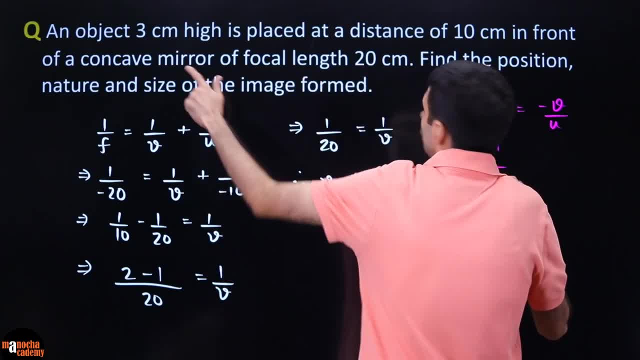 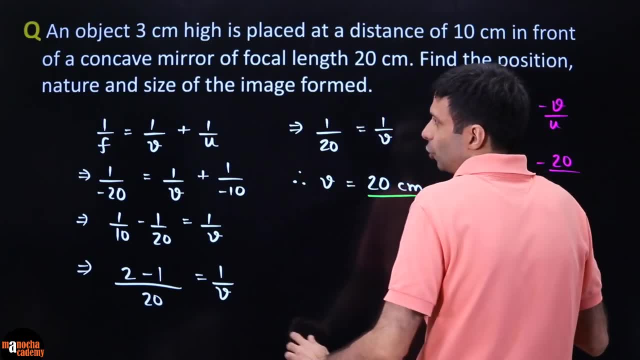 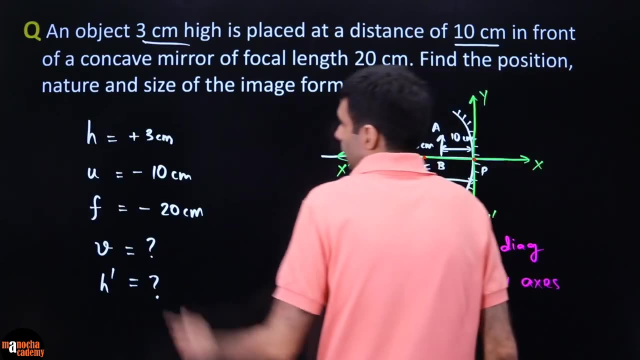 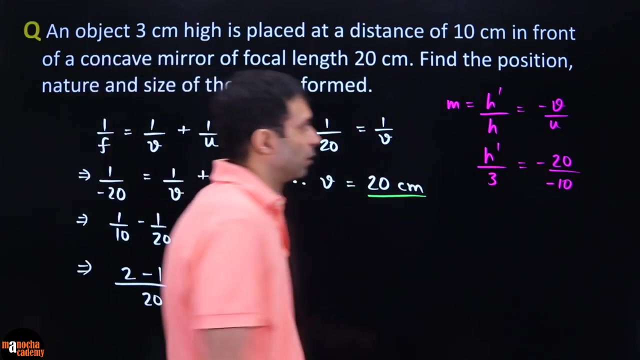 h dash object height: h is 3 centimeter minus v by u, so v is 20 and u is minus 10, again with the correct sign, see minus 10. so when you substitute that, what are you getting? the minus minus cancels. so this will cancel out here. 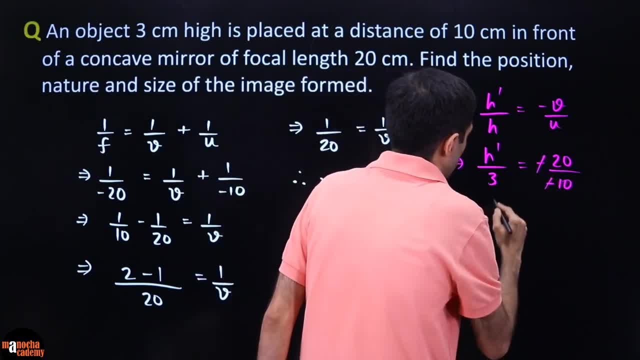 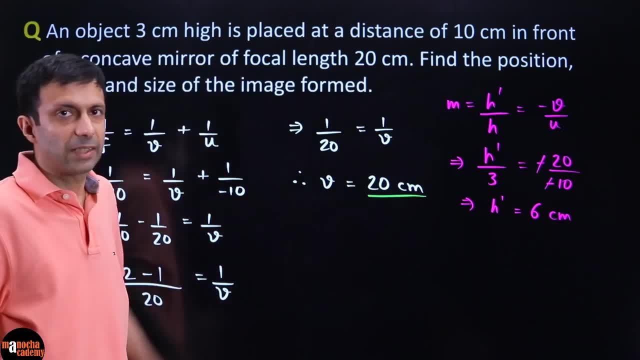 and so we are going to get h. dash is going to be 6 centimeters, not minus. 6 minus minus will cancel, because the magnification formula has a minus v by. u see, that's why each and every sign is very important. so this is our image height. 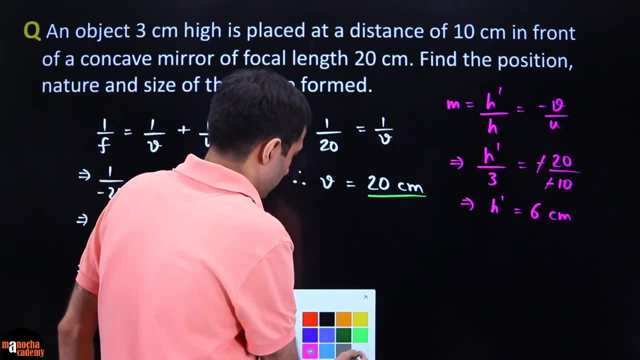 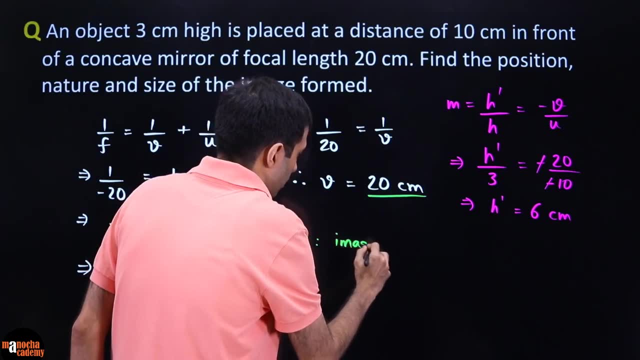 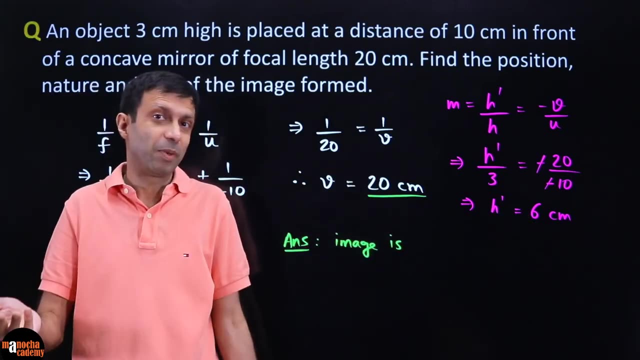 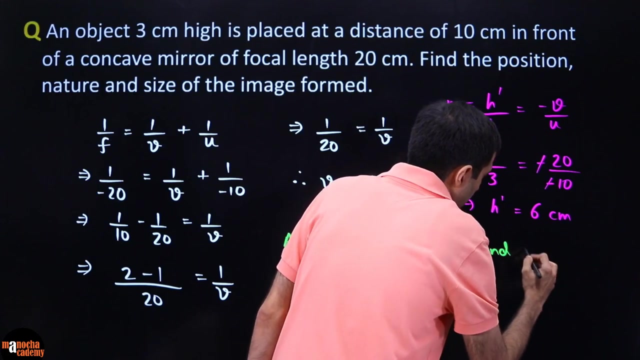 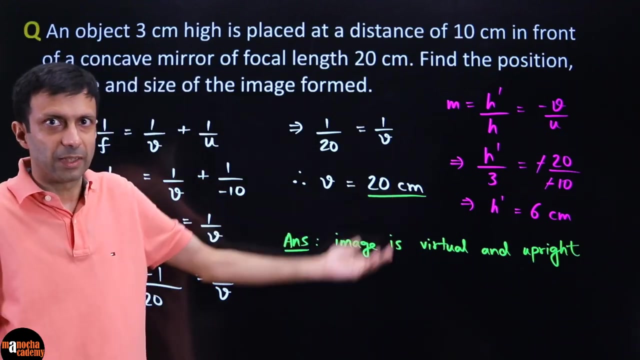 therefore, what is the conclusion about the image? so we can say: image is because it is a positive image. height means image is upright. that means it must be virtual, so image is virtual and upright. or you can write virtual and erect: upright means it is straight, so image is virtual and upright. 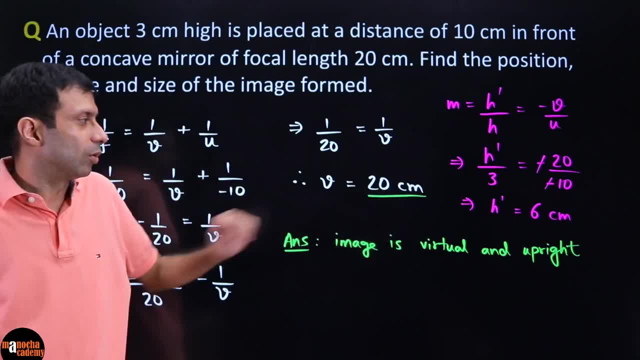 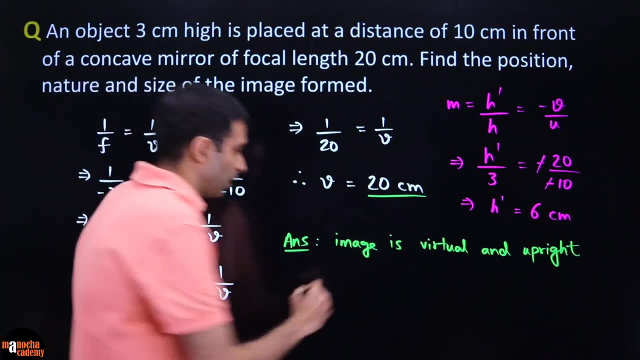 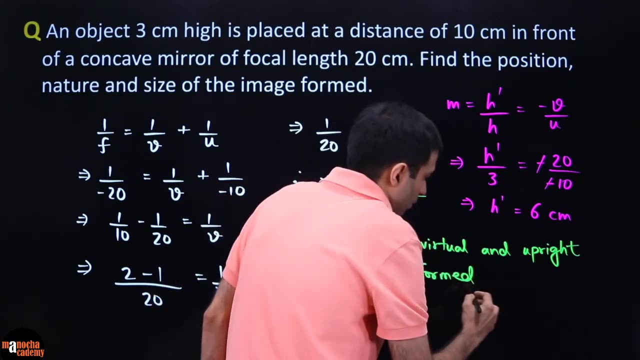 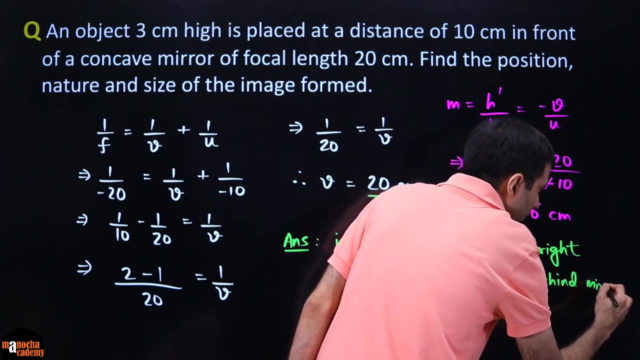 why? because positive height, otherwise you would have got negative height. so this is clear, then, what we can say: image is formed 20 centimeters behind the mirror. that is the placement of the image. image is formed 20 centimeters behind the mirror. and what else here? 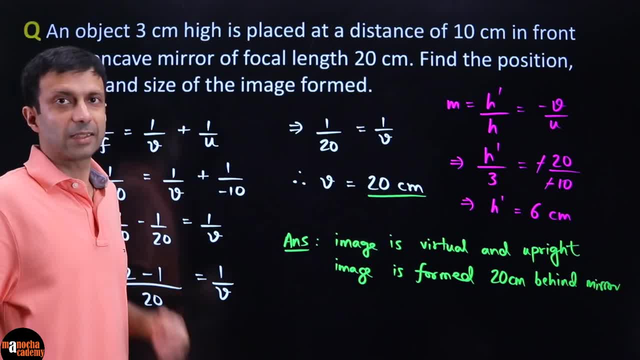 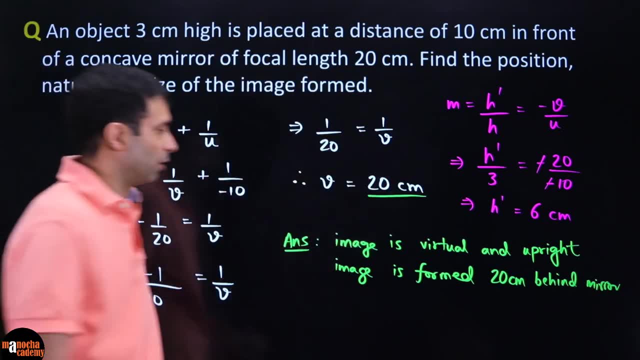 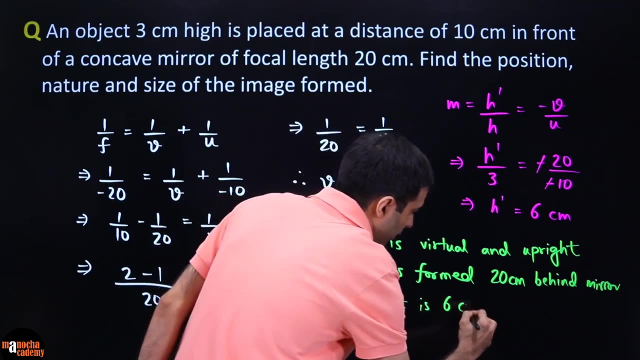 so these things we have got? and the last thing: size of the image. it is magnified, in fact double the size. right object was 3 images, it was 3 images, 6. so image is image, height is 6 centimeters, which means it is magnified. 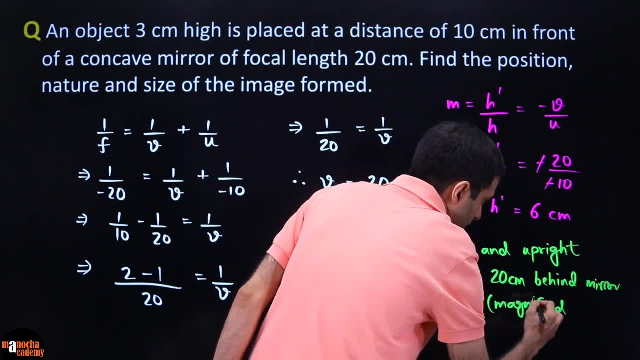 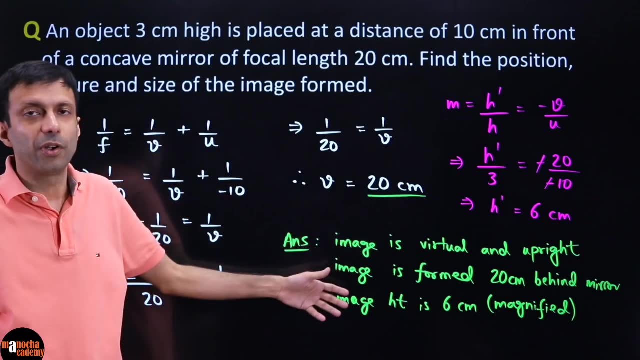 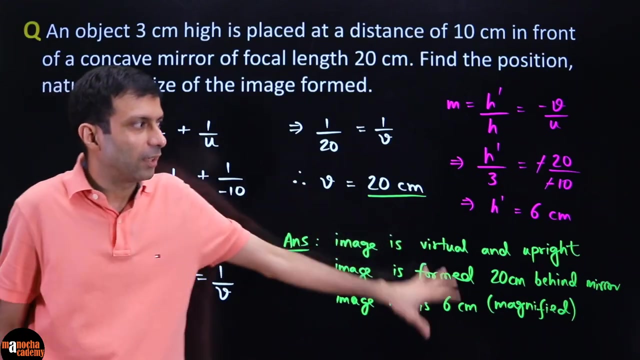 so of course you guys can write it in different way. also, you can say: image is virtual, erect, magnified. then give the details. whatever format you are following in school, but you must give all the details about the image that you have found or you have been asked to find. 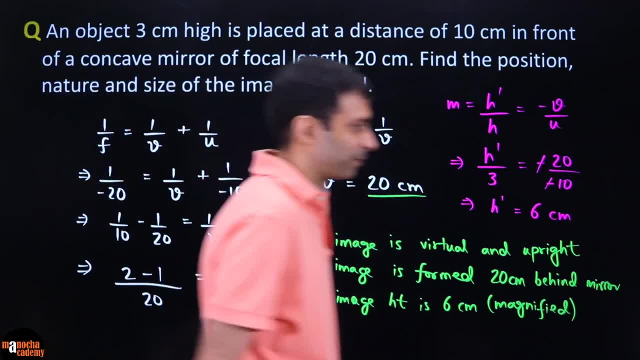 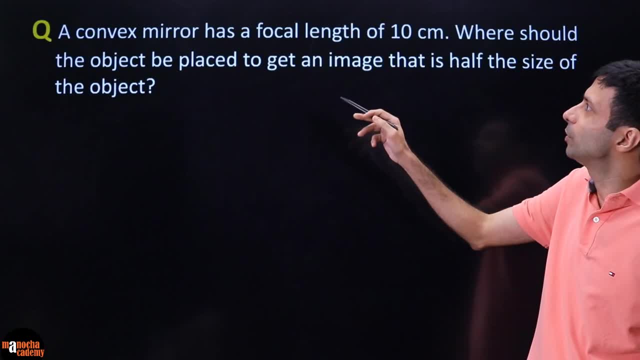 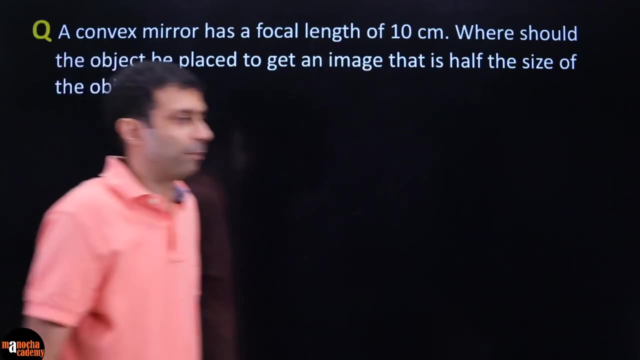 clear. so this is how we solve these questions. let's try another one, this time a convex mirror question. convex mirror has focal length of 10 centimeters. where should the object be placed to get an image that is half the size of the object? so again, what is the first step? 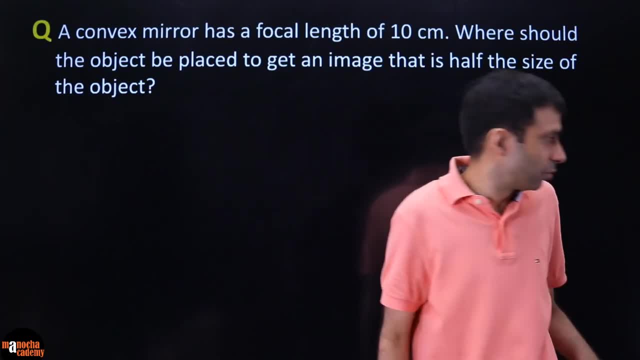 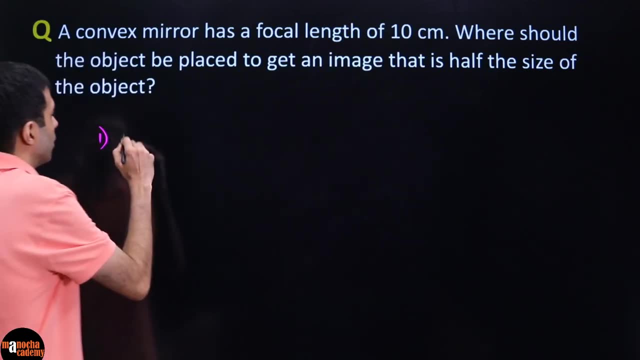 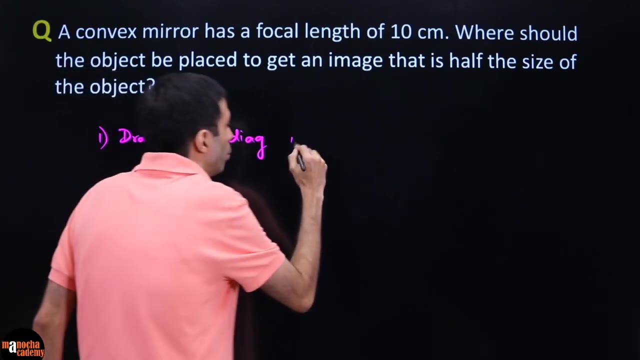 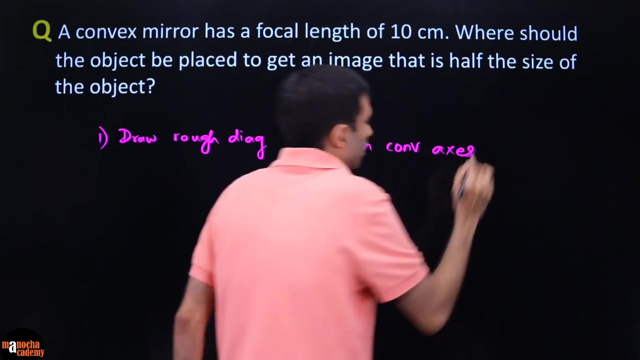 sketch a rough diagram. sketch a rough diagram like this. so always remember what is the first step. you guys promised me you will draw a rough diagram, so first thing, draw rough diagram with sign convention axis. this is super important, guys. if you don't do this, your question can go wrong. 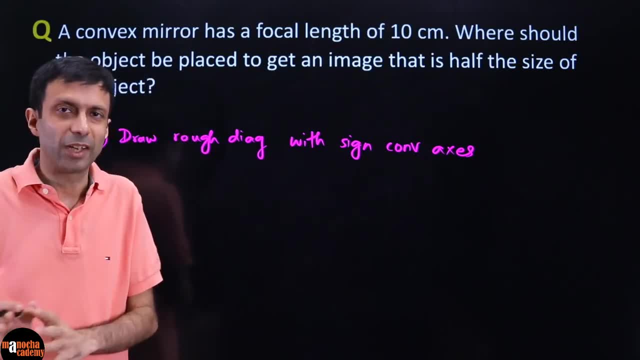 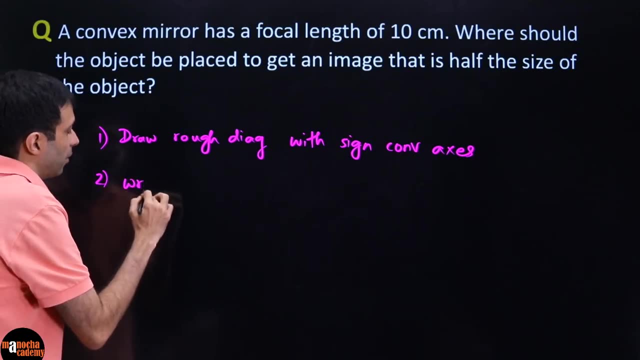 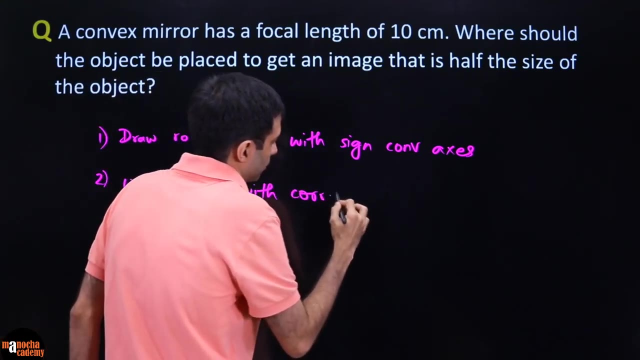 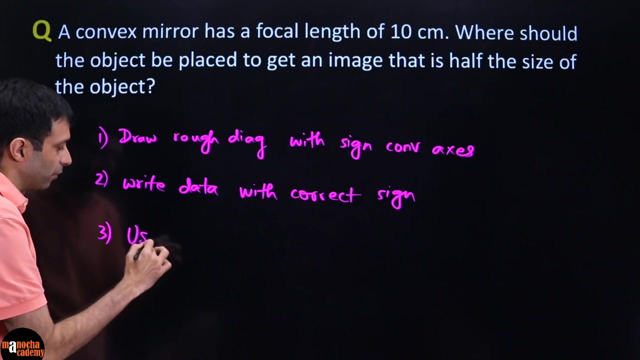 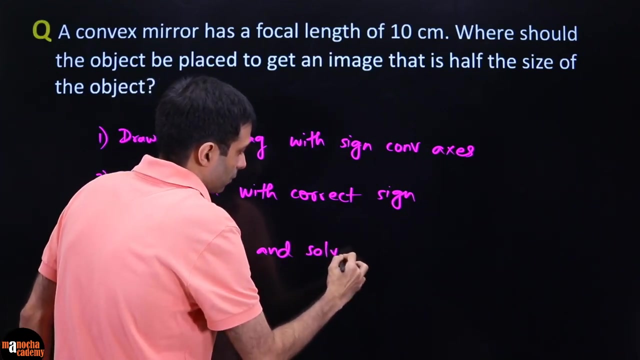 very important. that's why be careful: are you doing concave mirror, convex mirror? because things can go haywire if you do the wrong mirror. second thing: write the data with the correct sign and then use the formulas and solve. if you guys follow these three simple steps. 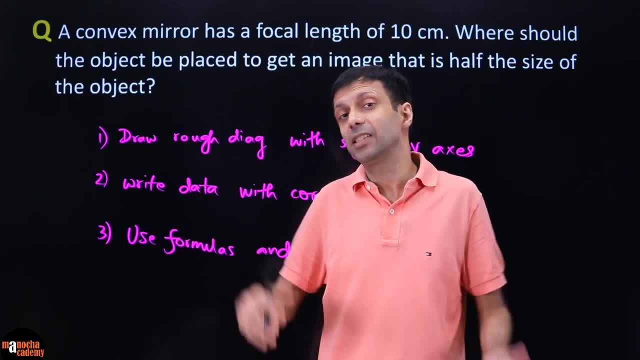 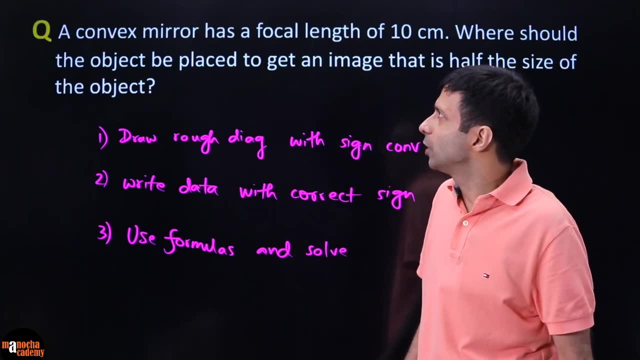 I am sure you can crack any of these mirror formula questions, and same things will apply when you come to lens formulas for concave and convex lenses. same tricks. so let's go ahead and quickly do this one. so first thing is you should draw a rough diagram. 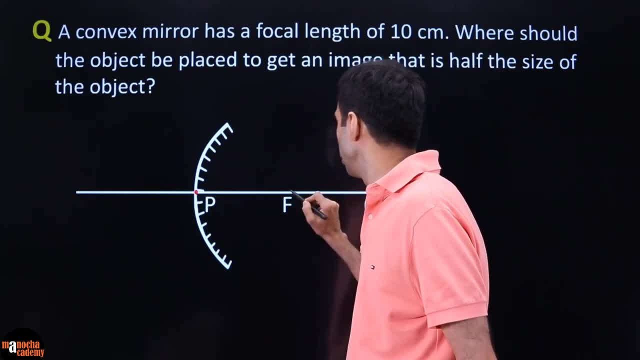 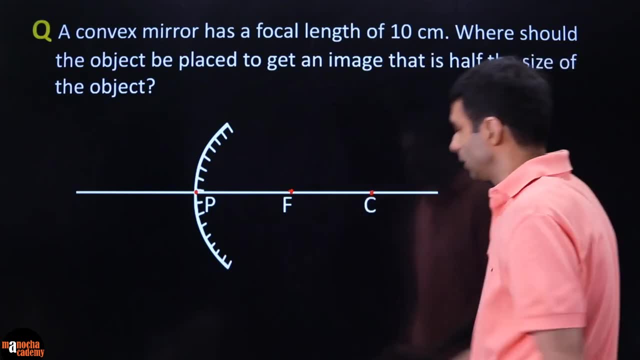 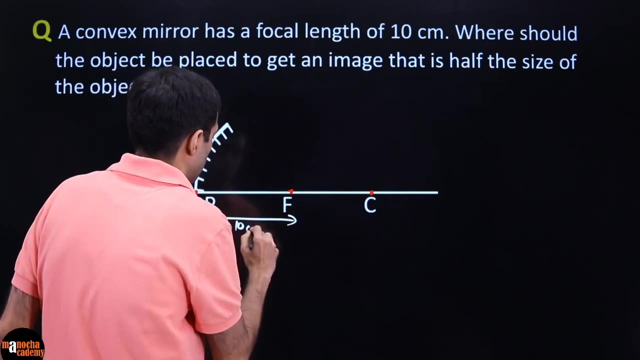 so just sketch something here out like this, so you have your pole focus and center of curvature. we can see that convex mirror has a focal length of 10 centimeters, so let's mark that here pole to focus is 10 centimeters. where should the object be placed to get an image? 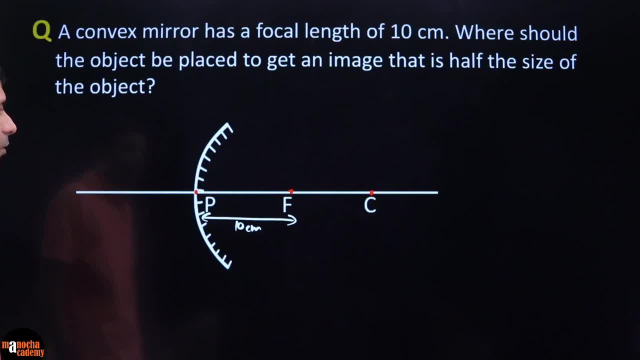 that is half the size of the object. so now we don't know where it should be placed, so let's randomly place it, because after all this is a rough diagram, we can just place it anywhere. so let's say object is placed here and it says it is half the size. 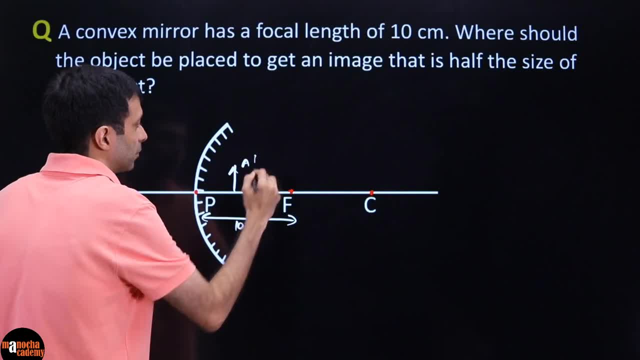 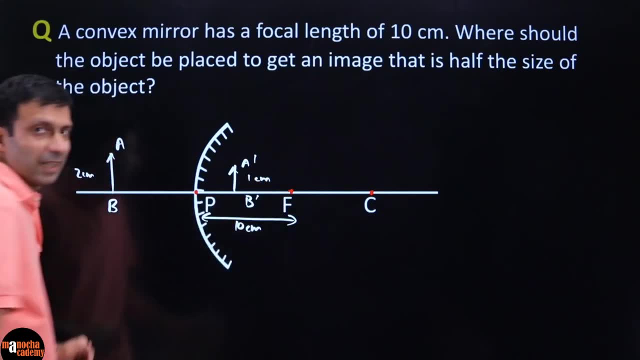 so that means, for example, if this is 2 centimeter object, this will be 1 centimeter, just as an example, but nothing, no real numbers are given. that is just to understand the scenario. so this is what we have here. clear again what is the important thing. 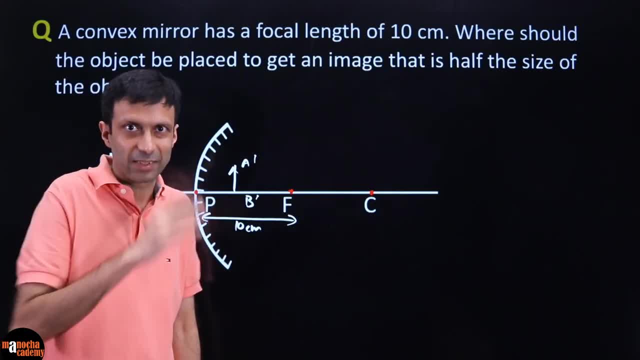 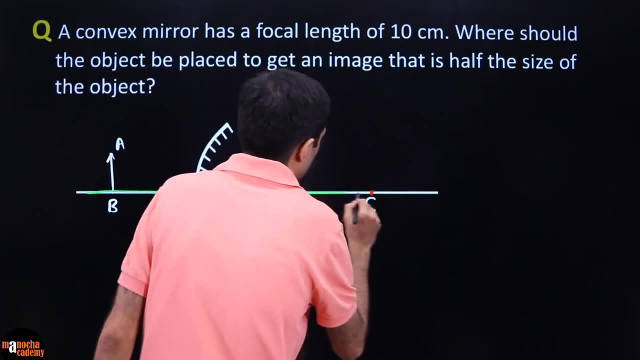 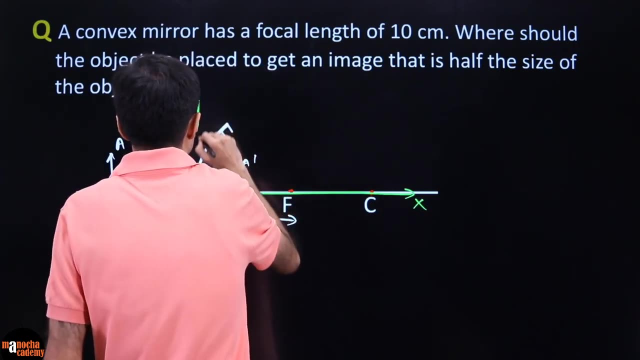 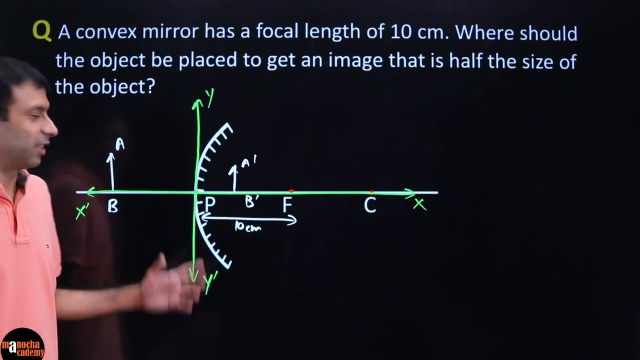 when you draw this rough diagram, please make sure you guys draw the coordinate axis, that sign convention axis. so let's draw that here. this is going to be my x axis and they are all drawn at the pole. okie dokie. so we have got our coordinate axis here, right? 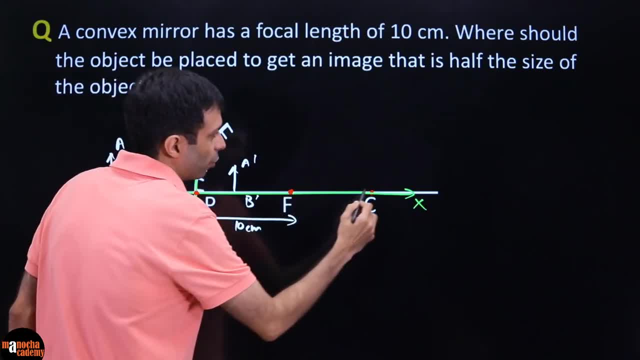 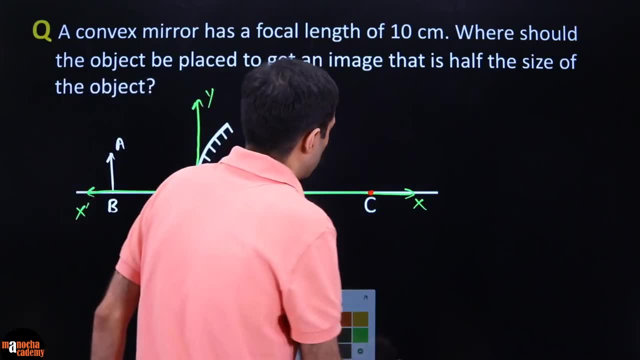 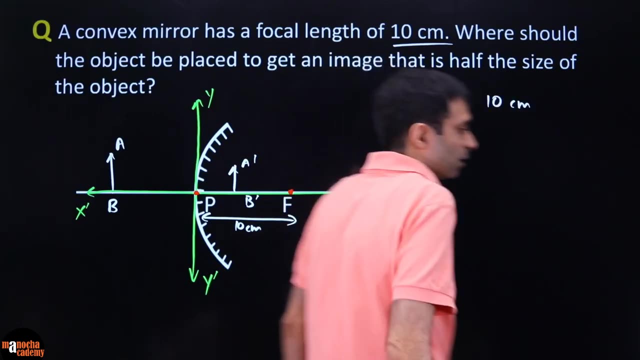 make sure you mark that pole which is like the origin, the focus, center of curvature. now quickly write down your data in terms of this rough diagram. so if you guys see here what is our focal length, 10 centimeters plus or minus, what sign should I put here, guys? 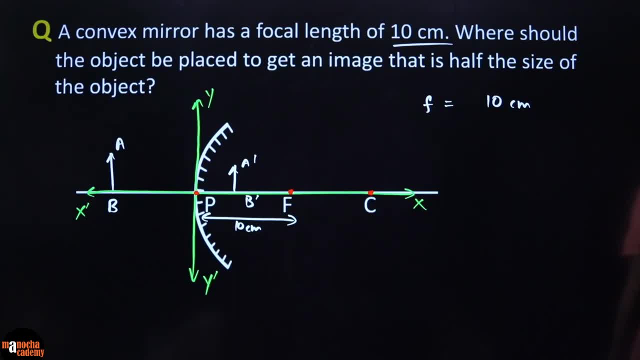 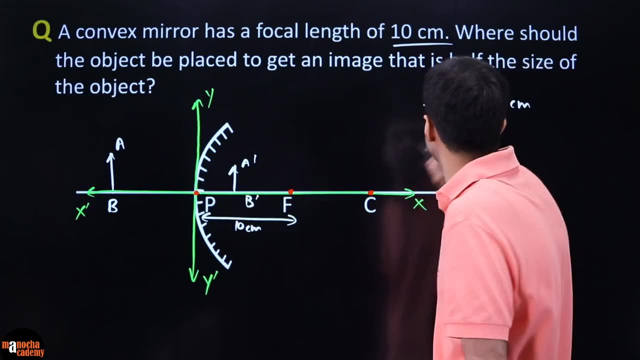 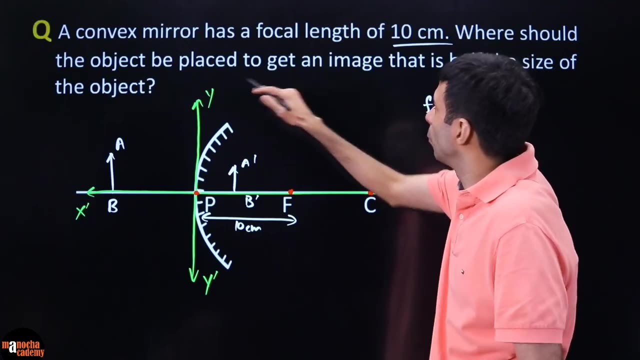 focal length. can you guys tell me positive or negative? clearly you can see. focal length is this thing from pole to focus along the positive x axis, so plus 10 centimeters, definitely. where should the object be placed? so, as you are reading the question, see what are they asking. 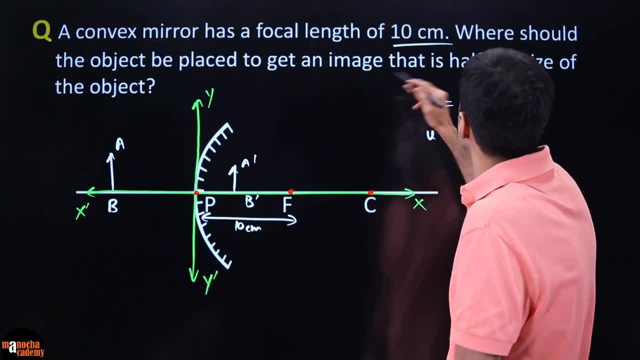 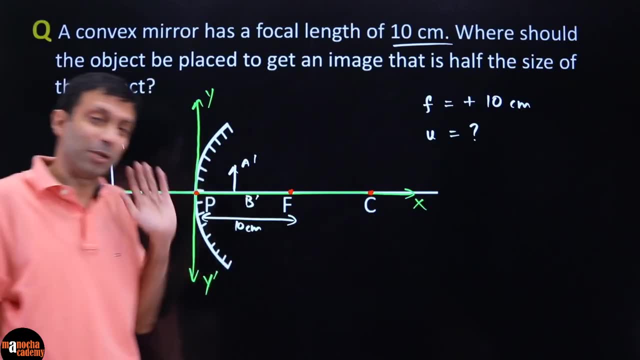 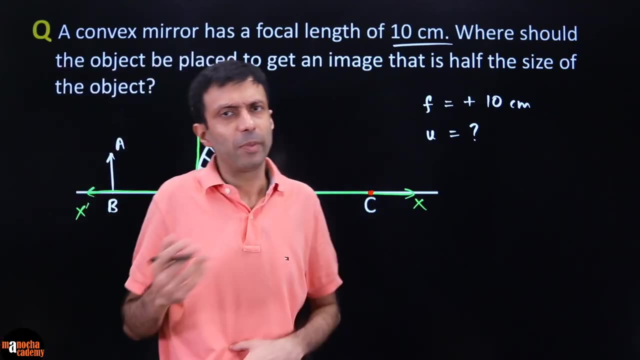 object distance, object distance, so that the image is half the size of the object. so in convex mirror, at least we know, image will be inverted. sorry, image will be upright. as I have drawn right, convex mirror always gives upright image. so if image is upright, what will be the magnification sign? 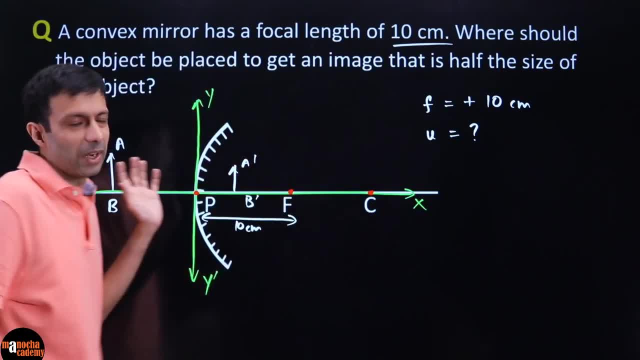 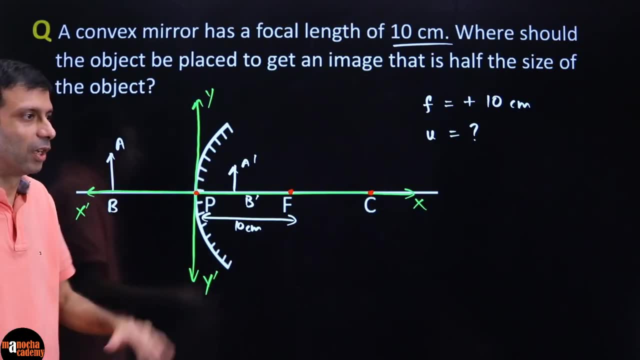 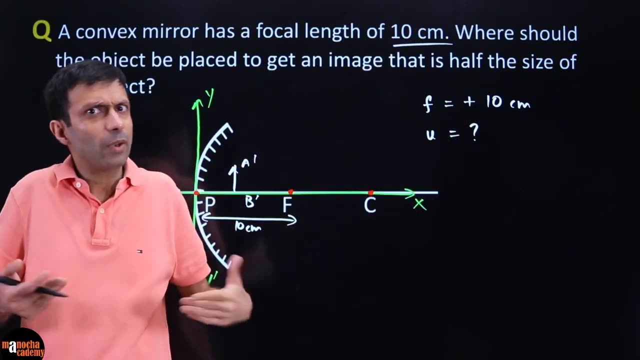 positive or negative. object is always usually upright, right. so upright, upright, clearly, magnification should be positive. negative magnification means inverted, doesn't mean small inverted image. so clearly magnification will be positive here, but the image is half the size of the object. so can you guys tell me what will be the magnification? 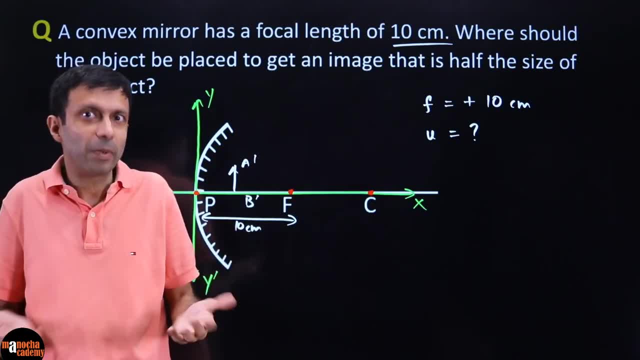 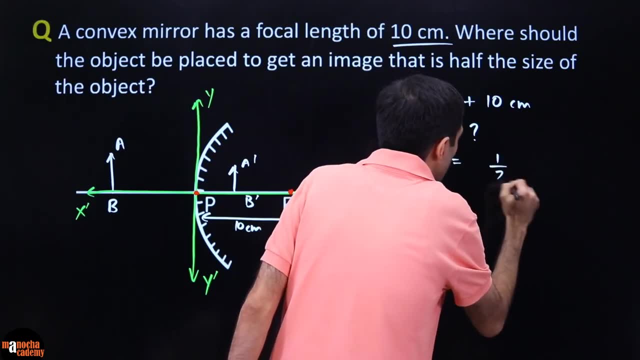 if image is half of the object, what is the ratio going to be half, 0.5, right? so we can simply say magnification is going to be half, again with that plus sign, that means I have taken the sign clear. so that's all the stuff and we have to find u. 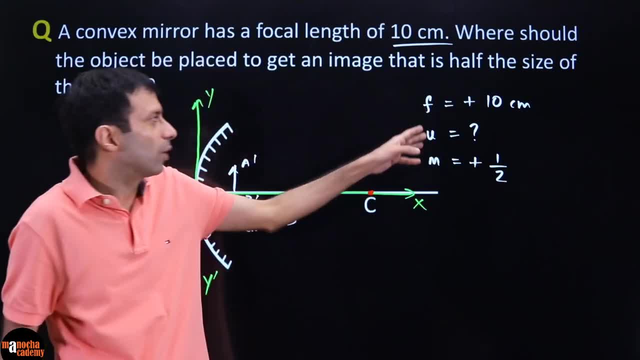 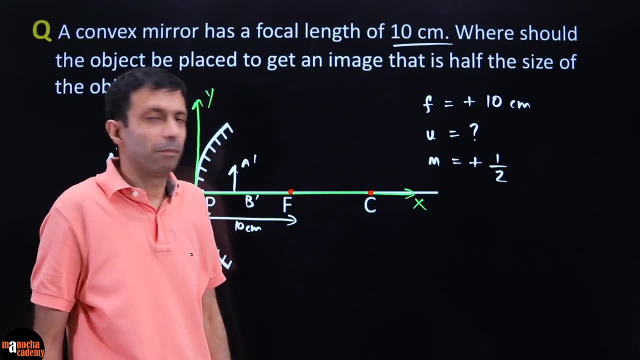 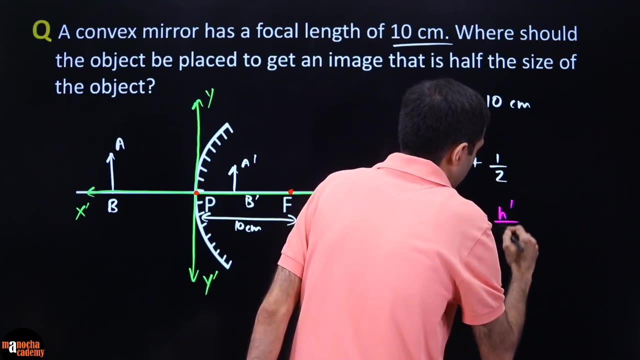 now there is no direct formula that connects focal length u and m. so what do we do? but we know that magnification, there is some formula right. magnification formula is h, dash by h, which is minus v by u. be careful, there is a negative sign, is there? 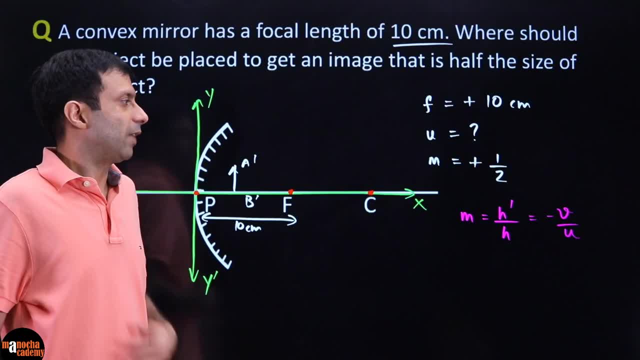 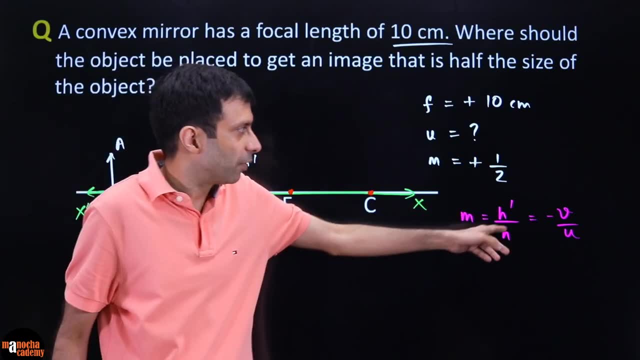 mirror formula is all positive here there is negative. so if you have h, dash by h is minus v by u, but we know that magnification ratio is half. so I can see that I am making some connection between v and u. yes, so therefore I can say that 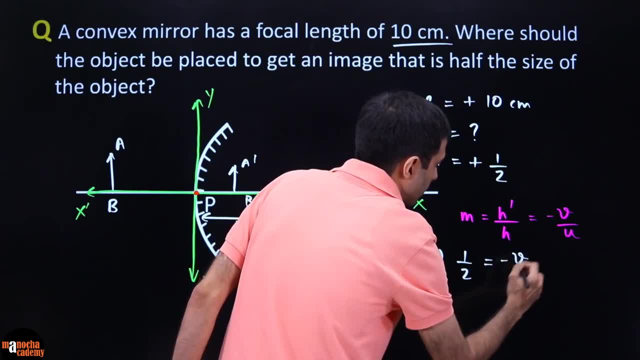 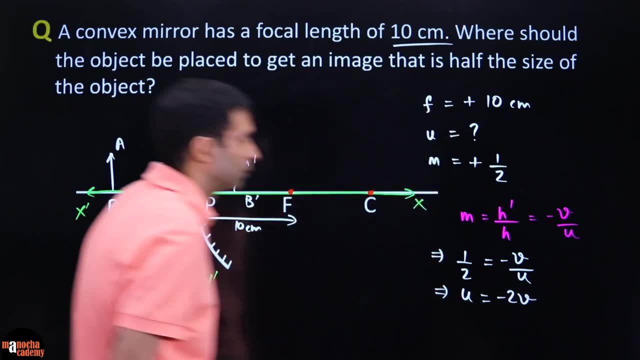 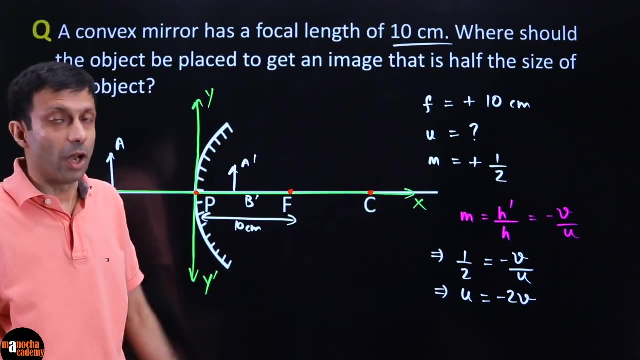 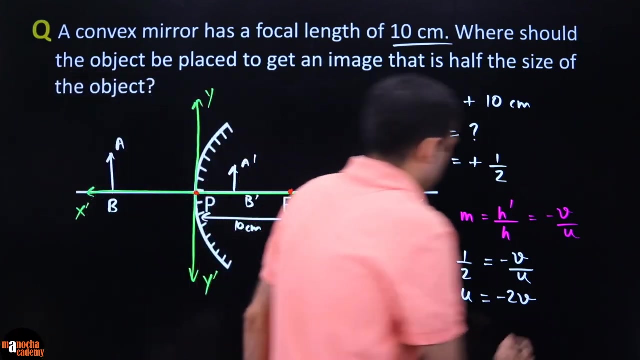 half equals minus v by u. or we can say that u is minus 2 times v. does this make sense? u equals minus 2 times of v. now we can use mirror formula, because maybe we can connect fu and we have one equation here: that u is minus 2 times v. 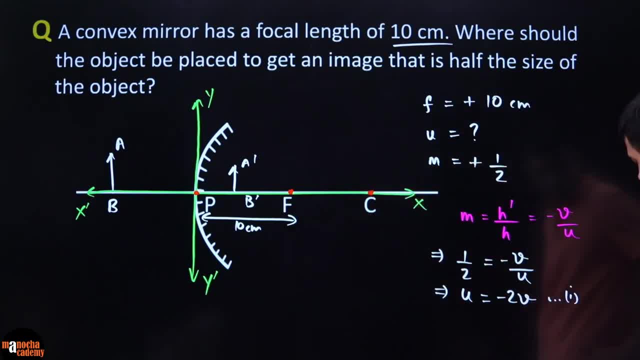 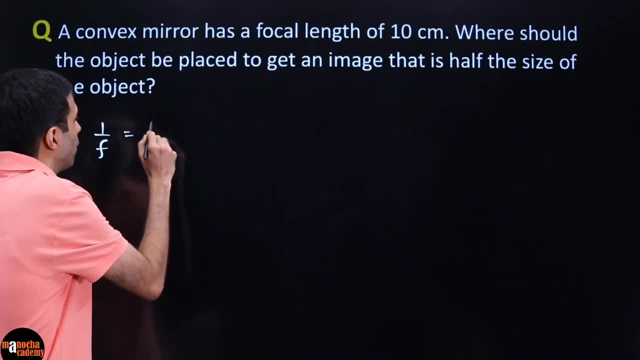 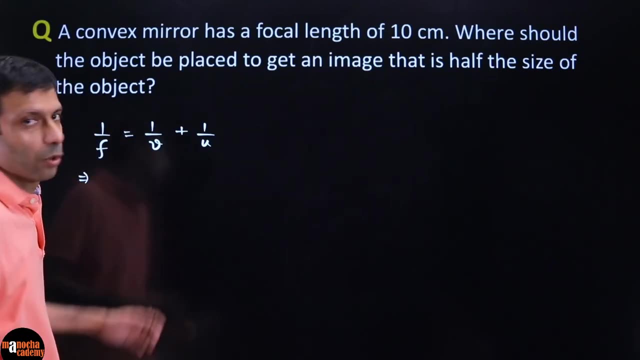 maybe we can use that. so let's go ahead and try it out. so I am going to write the mirror formula first. 1 by f is 1 by v plus 1 by u. focal length is always plus 10, so 1 by 10. 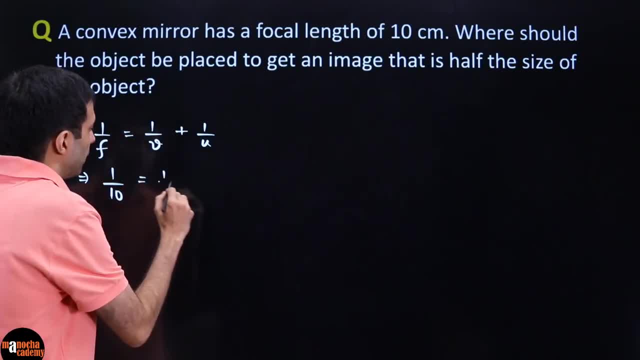 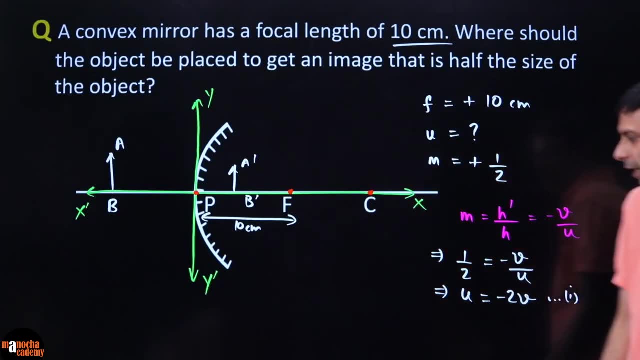 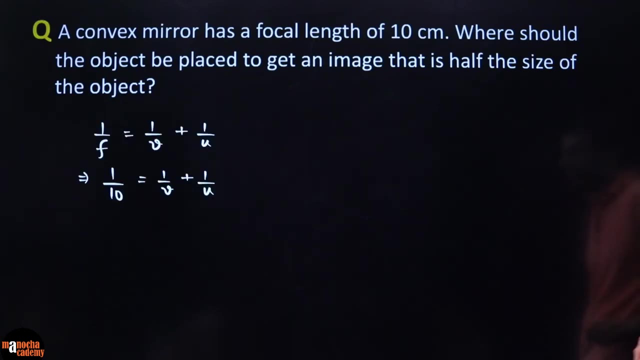 is 1 by v plus 1 by u, but what is the connection here? u is minus 2 times v, so maybe we can substitute u, we can replace it with minus 2 v, or you could replace the v with u by 2, based on that right. 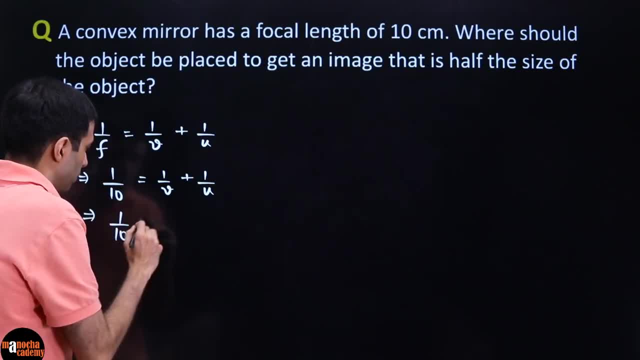 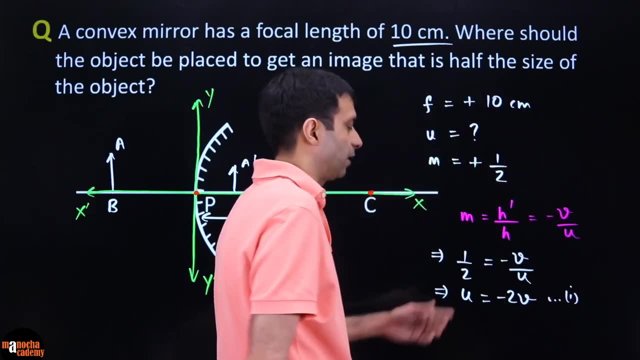 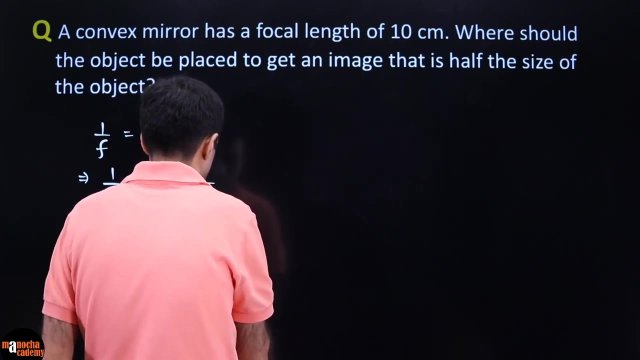 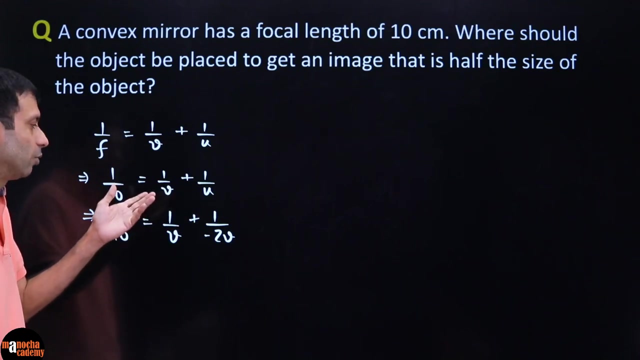 so I am just going to substitute. so we have: u is minus 2 v. so let's put that so. based on this, you calculate v and then you can calculate u. or you could have done directly. you know you could have changed the v into a u. 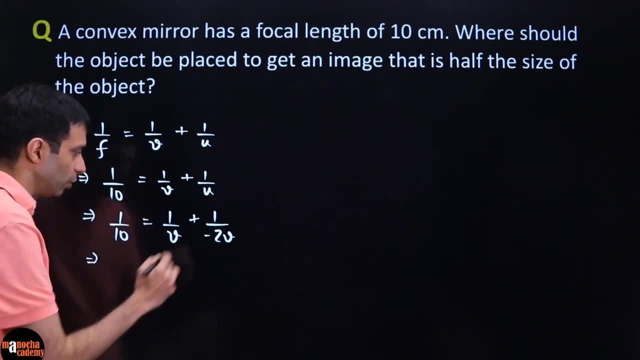 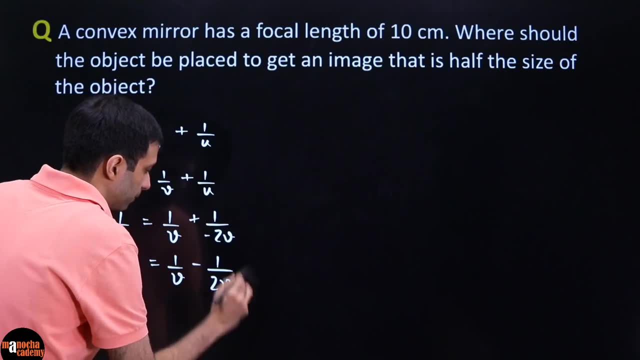 whichever way you want to go. so here, how will you guys do? please do this carefully. this is: 1 by 10 is nothing but 1 by v minus 1 by 2 v, so maybe you can take the 1 by v common. so smart way of solving this is. 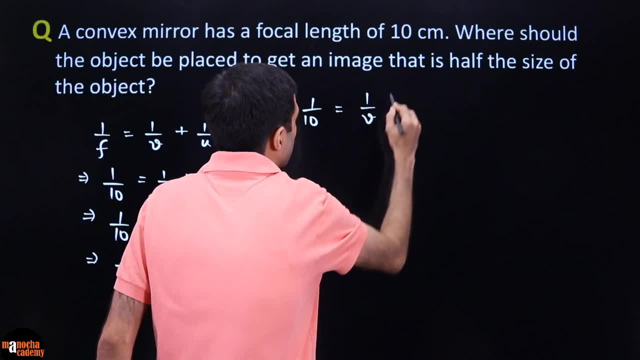 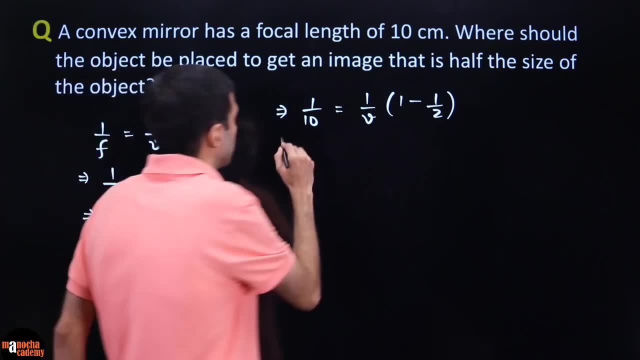 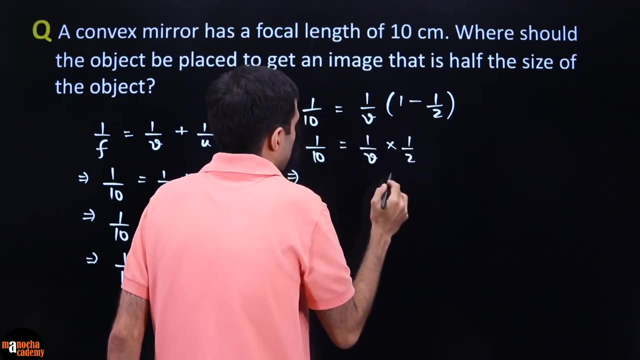 1 by 10 is 1 by v, and this becomes a 1 minus a half. yes, so 1 minus half is nothing but half. so 1 by 10 is nothing but 1 by v times half. so v is nothing but 5 centimeters. 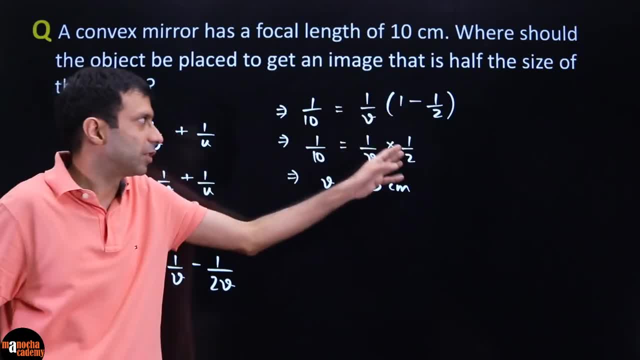 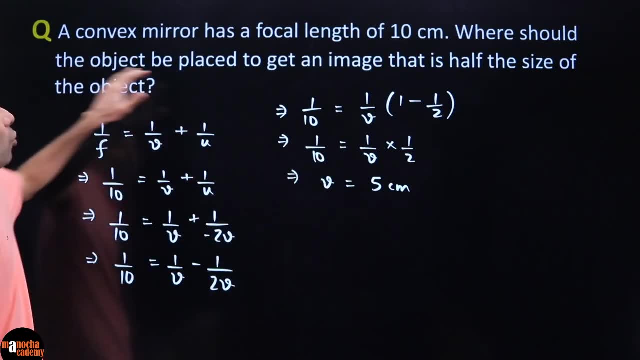 clear. so I just took the 1 by v in common. I was left with 1 minus half, which is half. so v is 5 centimeters because 2 v is 10. but I want my u because it is asking where should the object be placed. 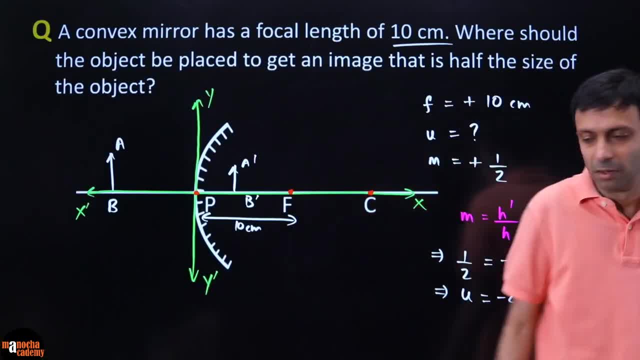 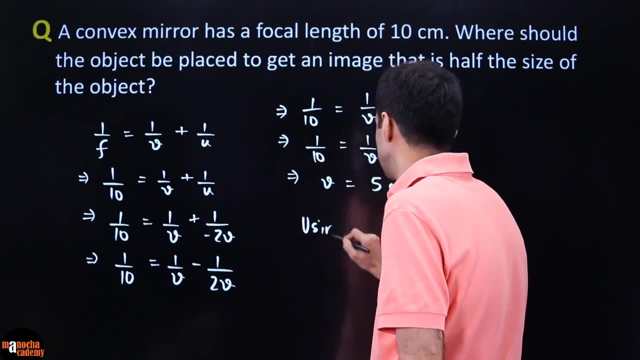 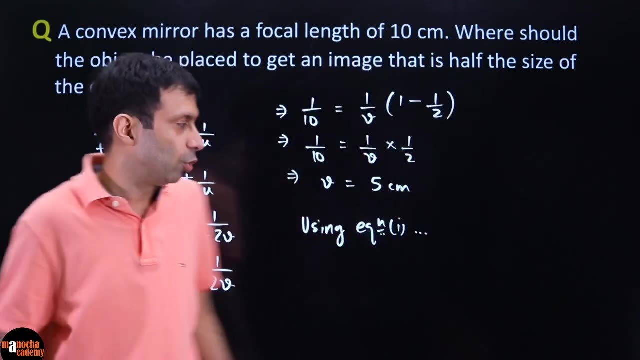 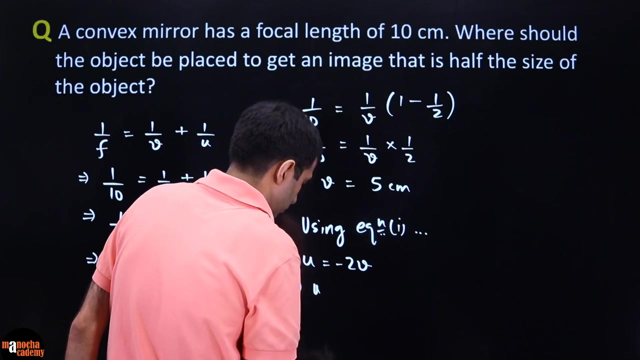 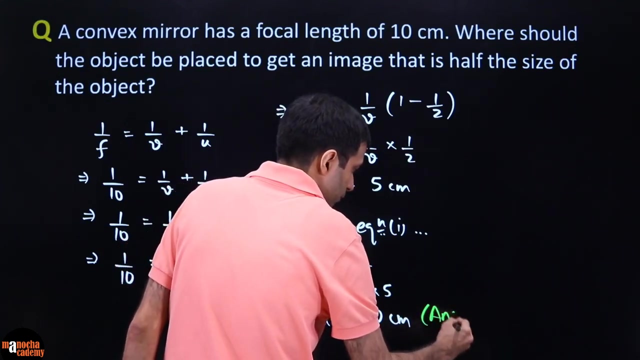 it is not saying where will the image be formed, but what is the connection? u and v are connected. so using 1 u equal to minus 2 v. so now we can say using one u equal to minus 2 v. there you go: minus 10 centimeters. 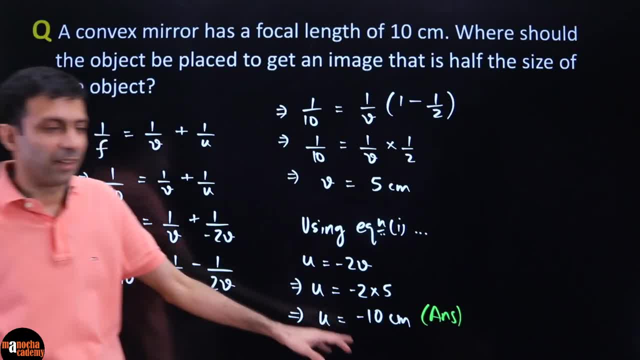 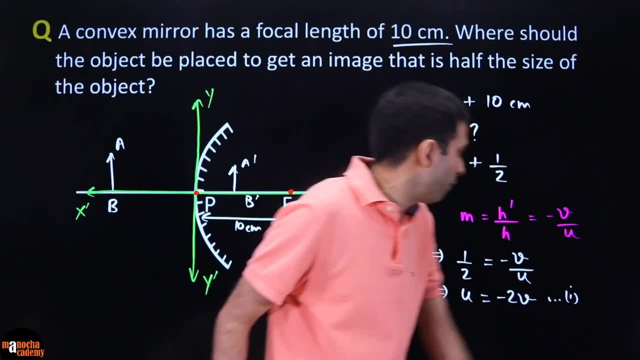 and we are done. so what is the meaning of minus 10? how will you write the answer? you better not to just leave it like that, better to write in sentence form. therefore, the object should be placed 10 centimeters. why is it negative? because it's on the negative x axis. 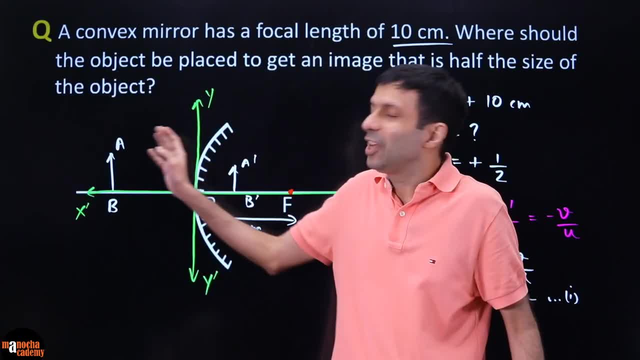 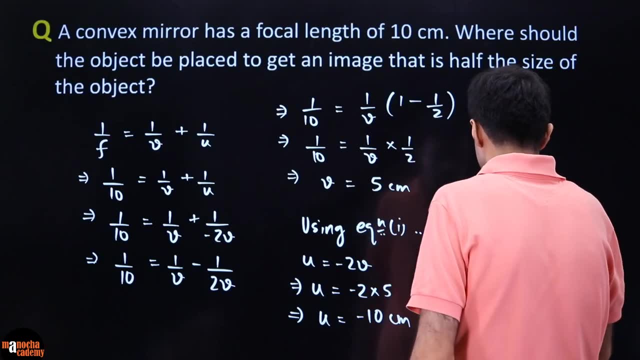 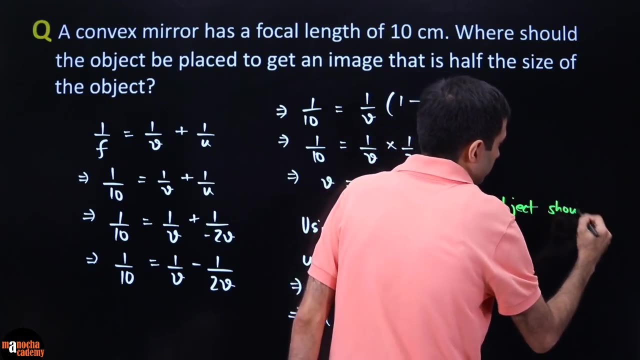 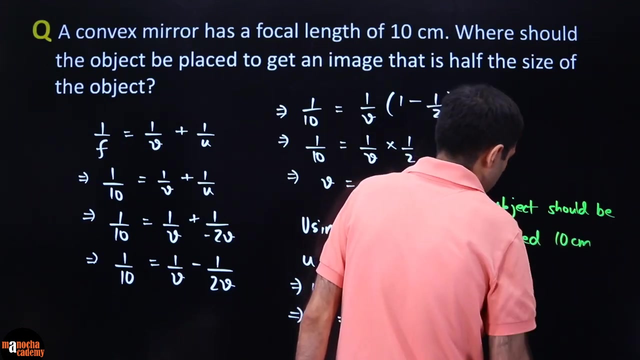 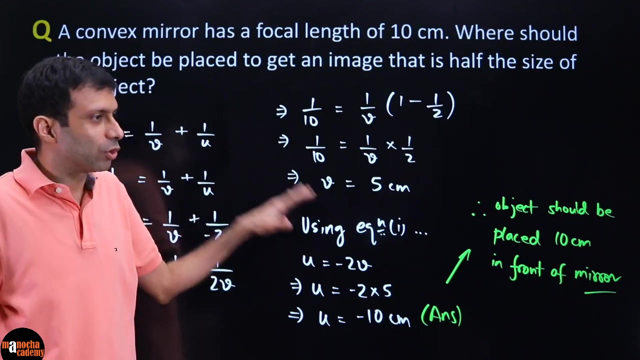 so object should be placed 10 centimeters in front of the mirror. that's how you write your answer, so we can write: therefore, object should be placed 10 centimeters in front of your mirror. that's it done. so see, when you draw a rough diagram, you just do the steps, write down your. 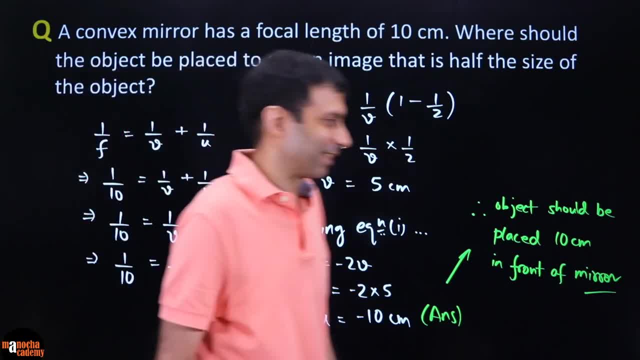 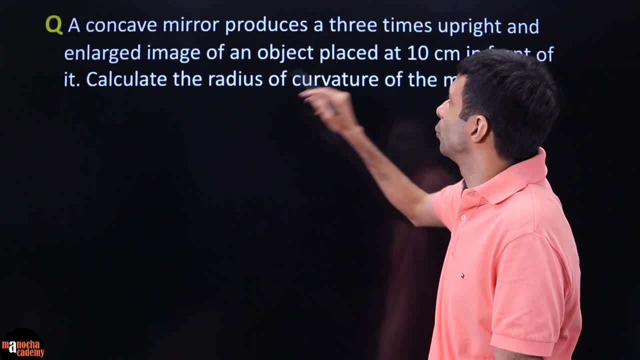 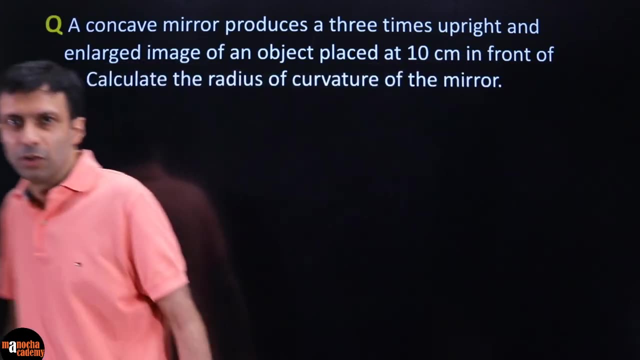 formulas. you can easily solve these questions, I think. one last question, let's try it out. a concave mirror produces a three times upright and enlarged image of an object placed at 10 centimeters in front of it. calculate the radius of curvature of the mirror. so, once again, draw a rough diagram. write down your data. 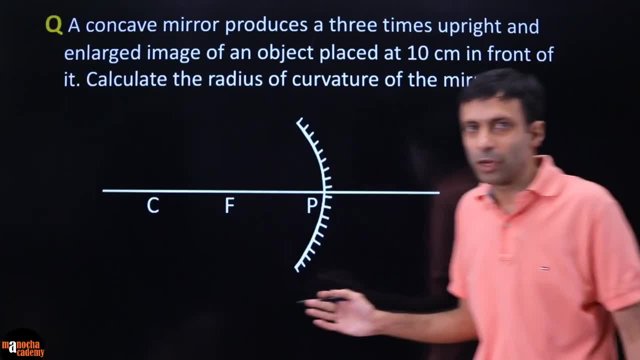 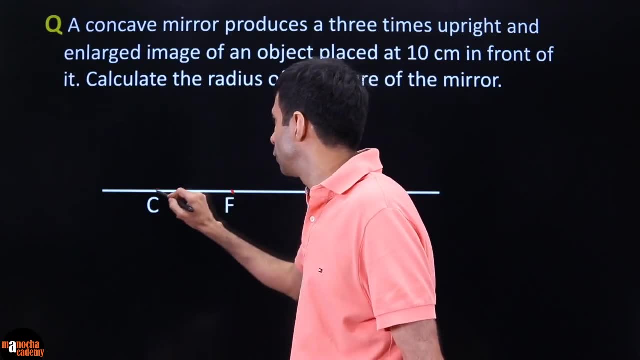 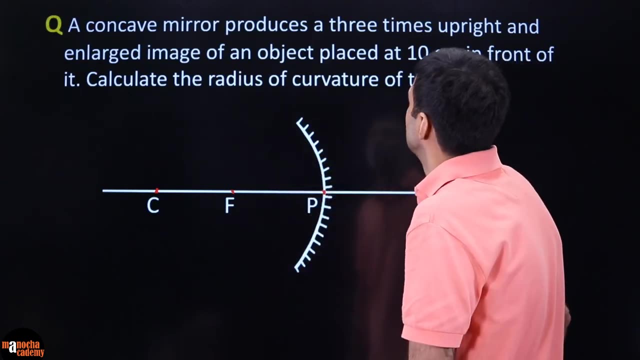 and try to solve this question. so see rough diagram. will involve a concave mirror. so we will mark the pole focus, centre of curvature of the mirror. what does it say? concave mirror produces a three times upright and enlarged image of an object placed at 10 centimeters in front of it. 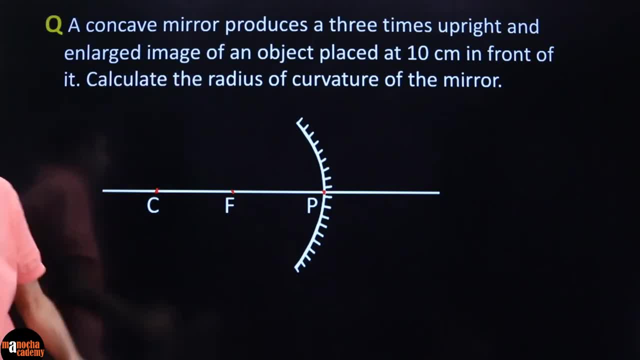 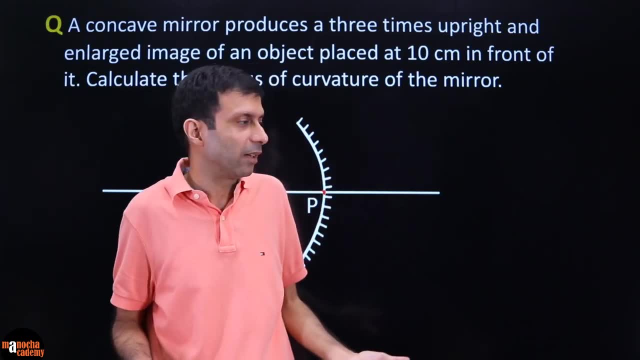 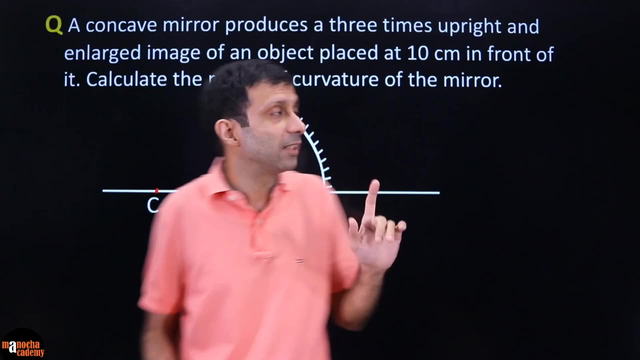 so when does the concave mirror produce enlarged and upright? can you guys tell me? so maybe we can use our case knowledge? of course you can draw a rough without thinking about that, but it helps to think so. when does a concave mirror produce an enlarged image which is upright, which means it is not inverted, it is upright? 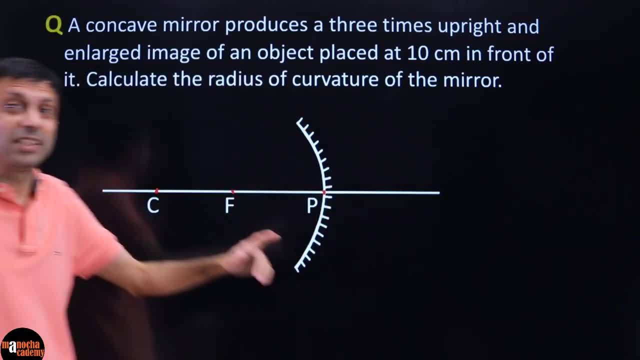 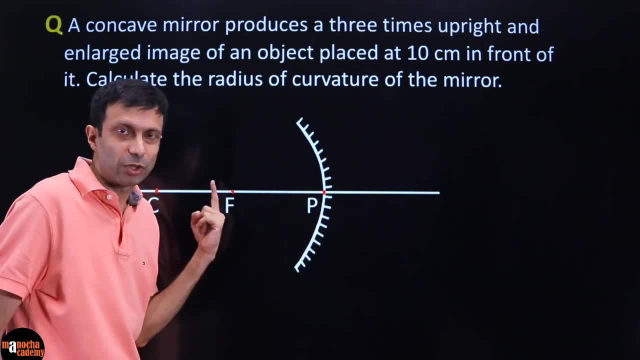 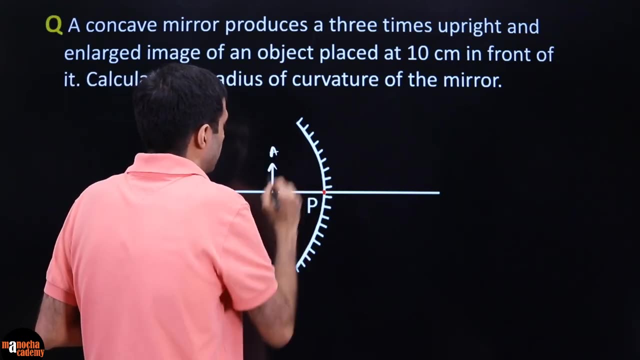 it is upright means it is virtual. so this is again that shaving mirror or make up mirror case. so we know that definitely, object will be between pole and focus of the mirror. see, there are clues in the question. so we know that our object will be somewhere here, because 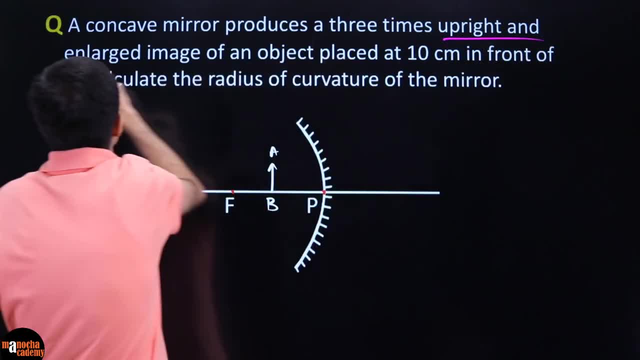 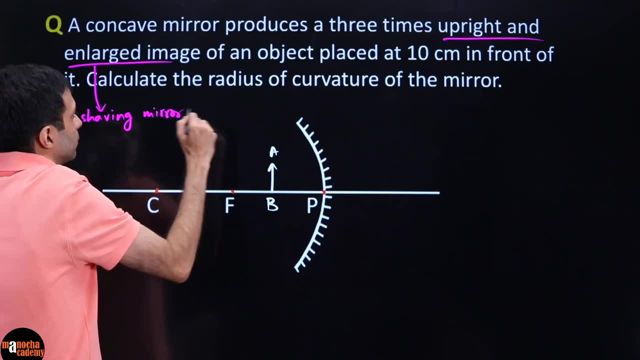 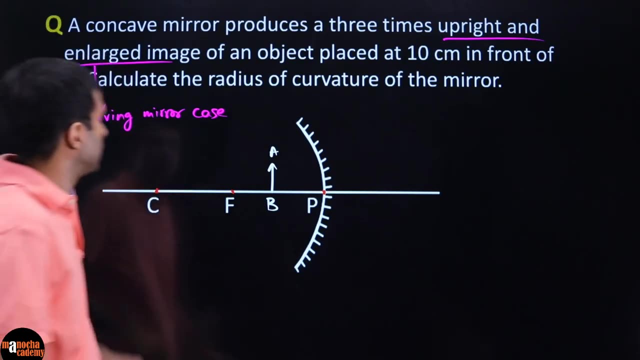 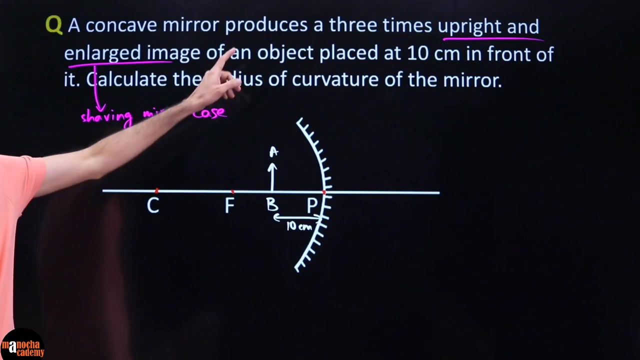 this is a clearly a shaving mirror case, right? so we are clear about that object: 10 centimeters in front of it, so let's mark the object distance given as 10 centimeters. and it says it produces 3 times upright and enlarged image. So if you look at this, 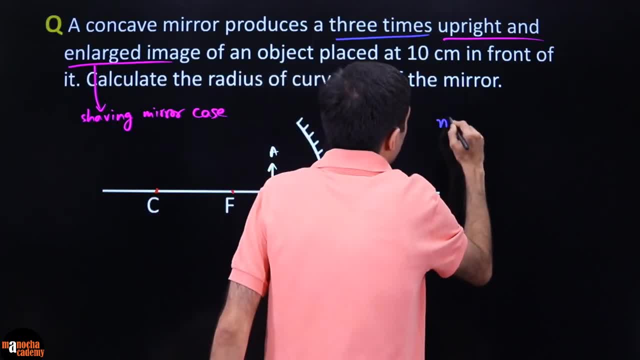 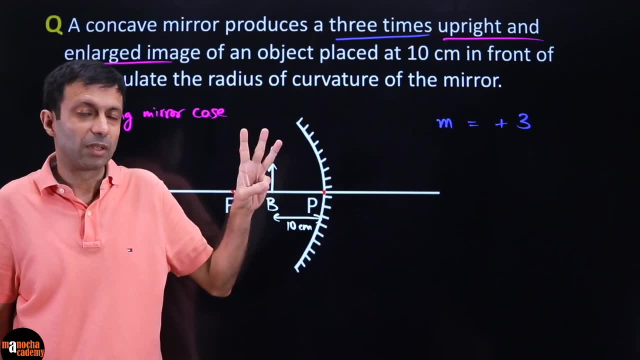 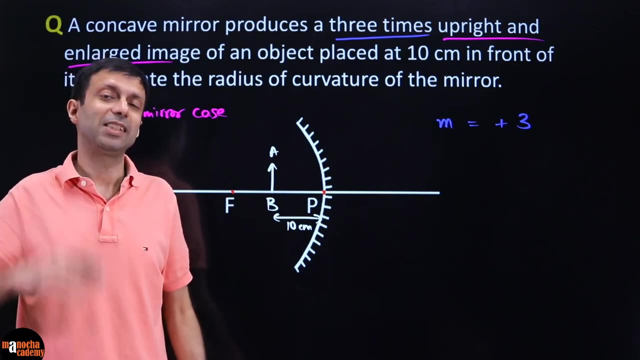 since it is 3 times, we know what will be the magnification plus 3. why did I write plus 3? because 3 times, and positive because upright image. negative means it is a inverted image. so positive magnification means image is upright clear. so we have written this and now we know. 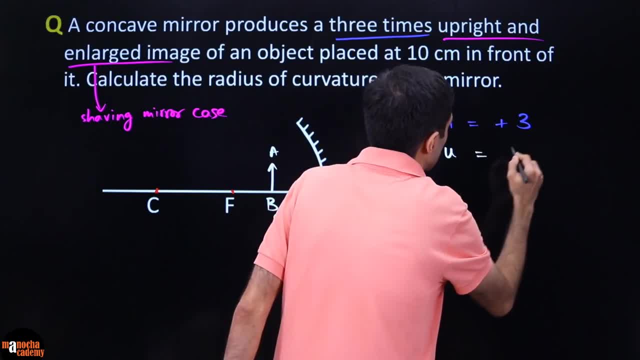 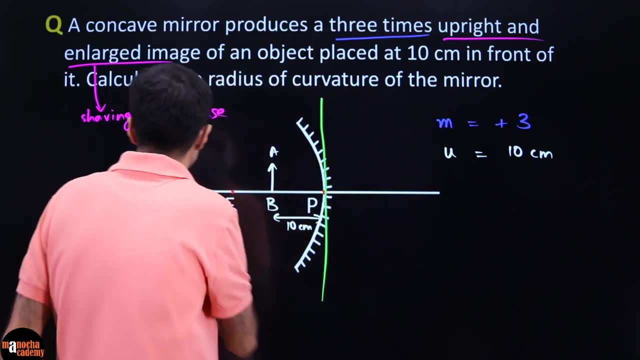 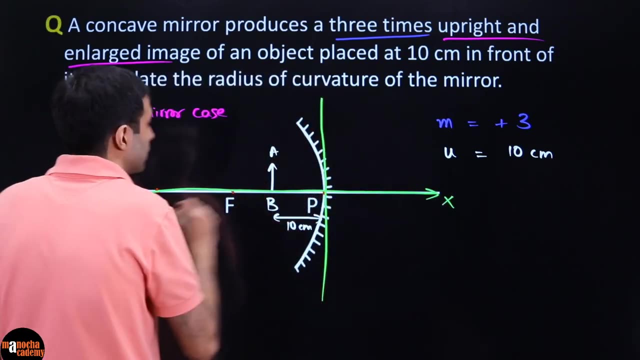 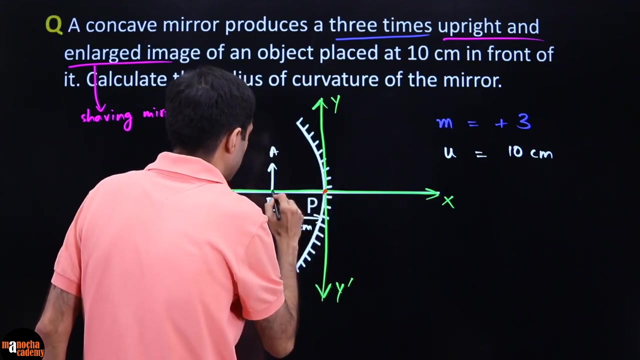 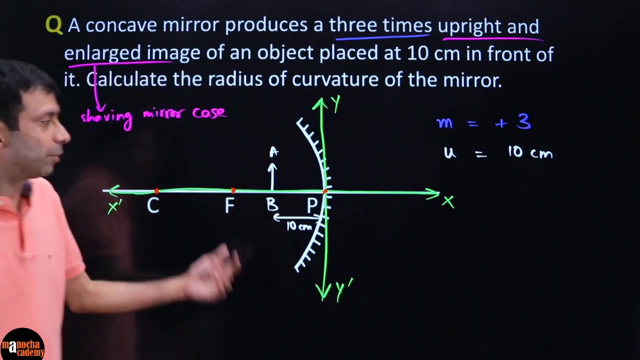 that object distance given to us is 10 centimeters, but again sign convention. so please do not forget to draw this sign convention axis. we have x, x' why, why so clearly object distance, positive or negative, object is in along the negative x axis, it's in. 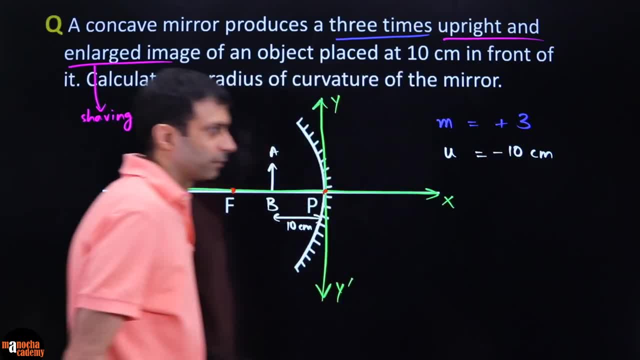 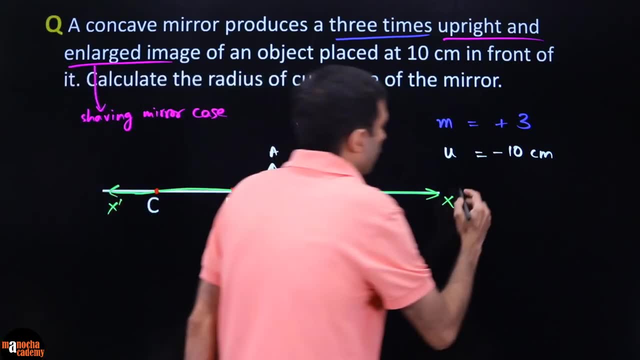 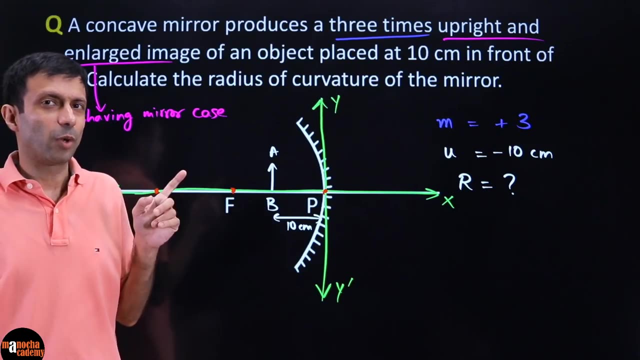 front here, right, so along the negative x axis minus 10 clear. and what do you need to find? radius of curvature of the mirror. so we don't need to find, we need to find the capital r radius of curvature. remember there is a formula connecting radius of curvature and what focal length. because we 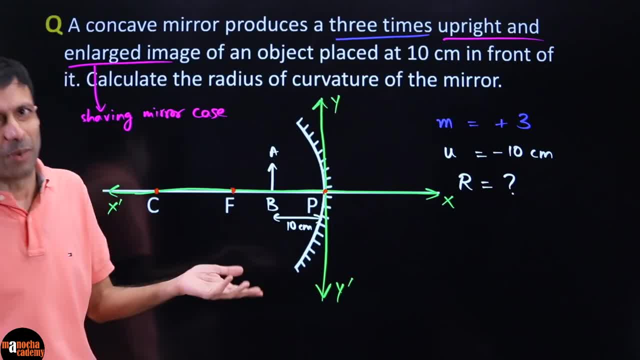 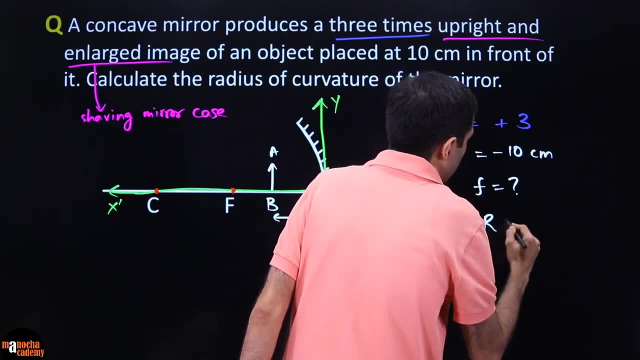 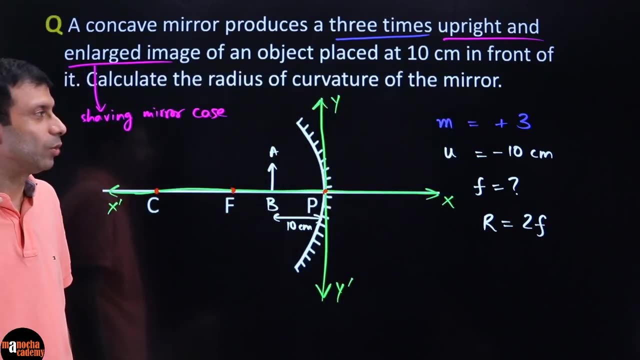 know it's twice the focal length. so basically we need to find f and double it right. so actually we need to find focal length and that will lead us to the radius of curvature 2m. that's it. so how will you guys do this? come on, so you can see. some magnification is given. that means we 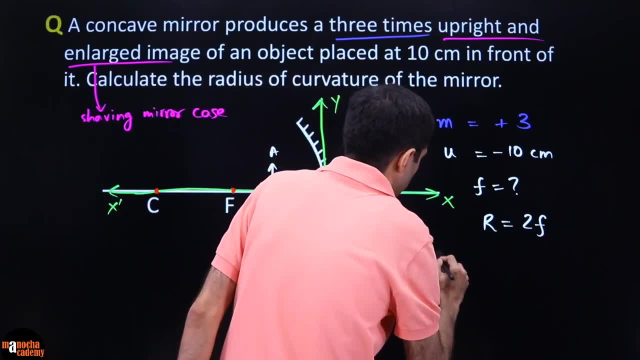 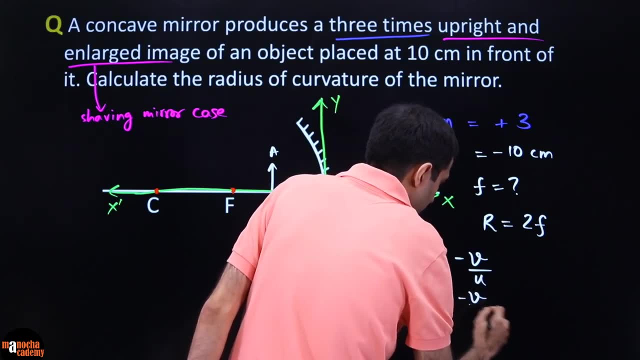 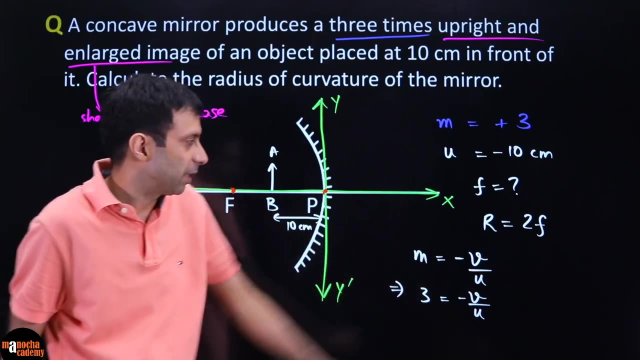 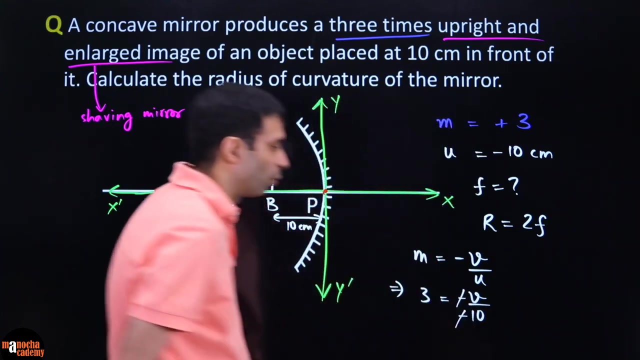 can use magnification formula. so we know: magnification m is minus v by u. 3 is yes, minus v by u, but u is given to you minus 10, so please substitute it here. the minus minus gets cancelled. so what is the image? distance: 30 centimeter. 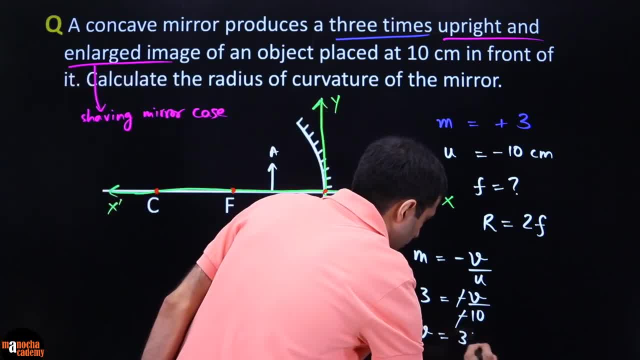 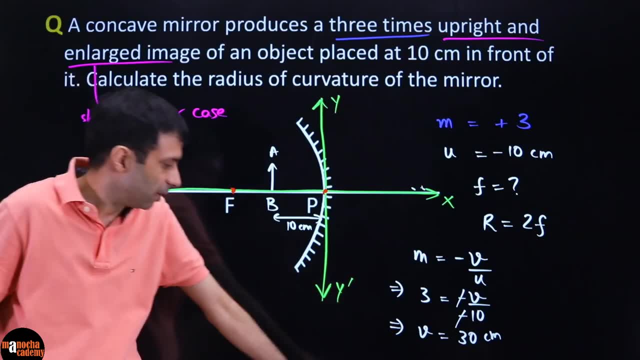 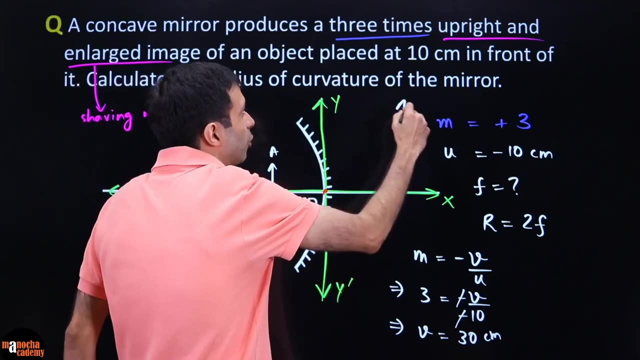 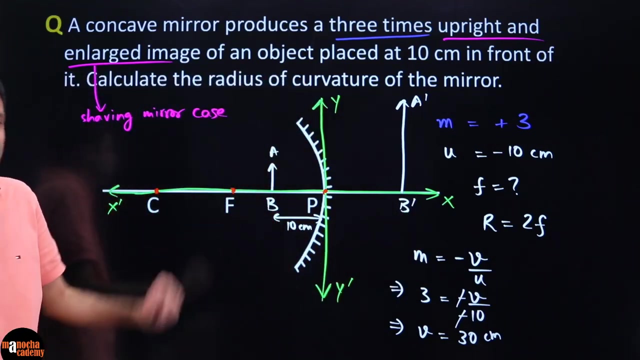 30 means plus, so it's along the positive x axis. that is exactly what we expect, because in a shaving mirror case we expect the image to be formed behind the mirror. we expect this three times magnified to be here, so that definitely makes sense: 30 centimeters image distance: 10 centimeters. 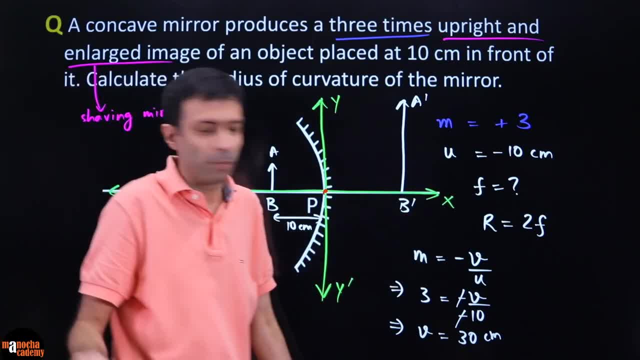 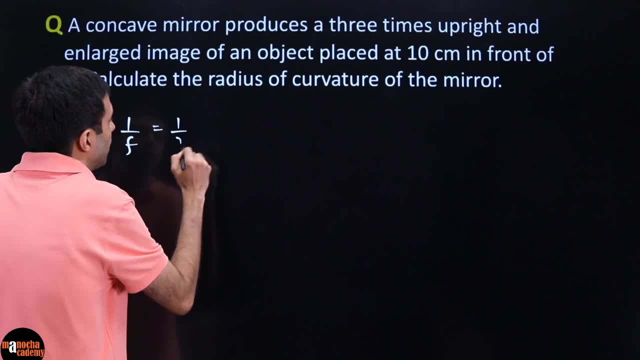 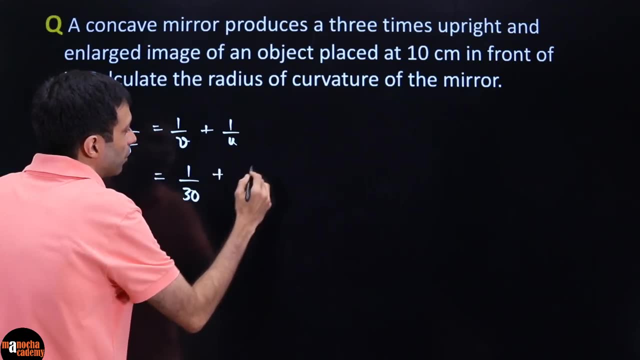 object distance. all we need to find is focal length. let's use mirror formula for that. so, using mirror formula, 1 by f is 1 by v plus 1 by u. the image distance we found was 1 by 30 and the object distance is minus 10, right. 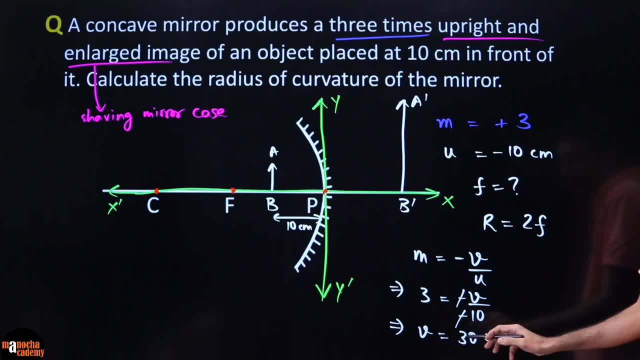 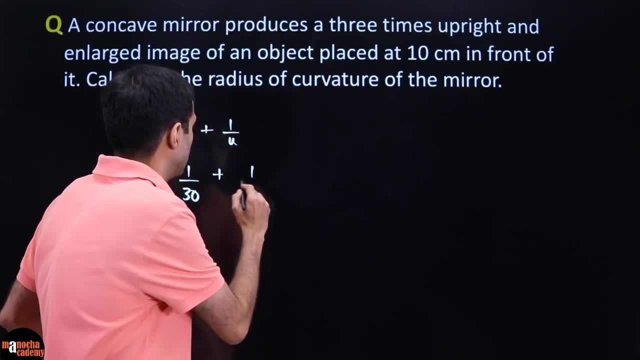 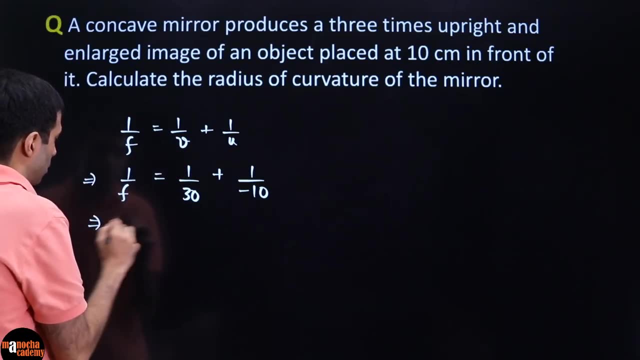 see very important to use the correct sign: minus 10. this one is positive, so just go ahead and solve this equation. just solve for f or 1 by f is basically going to be 1 by 30. you can bring this minus up here, so minus 1 by 10. 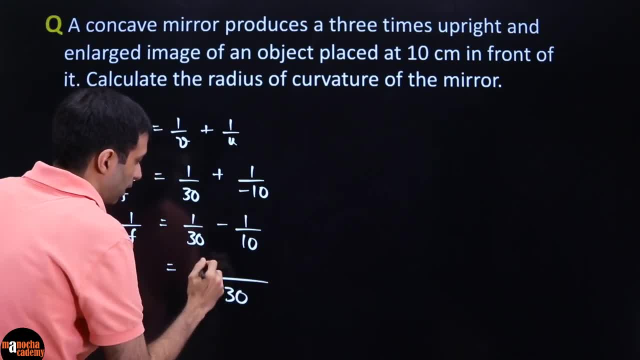 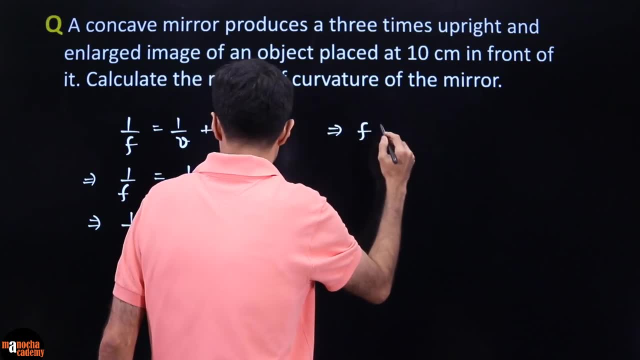 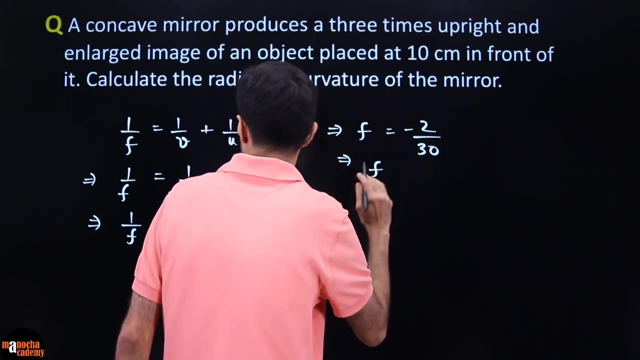 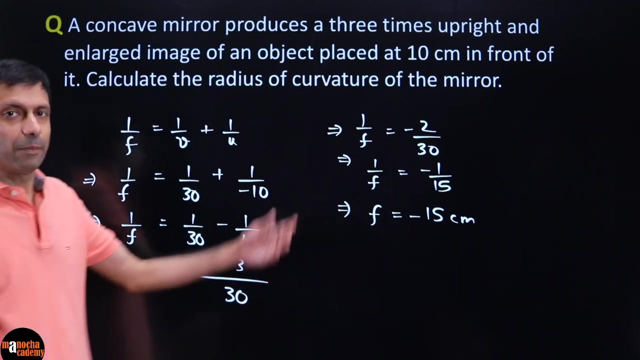 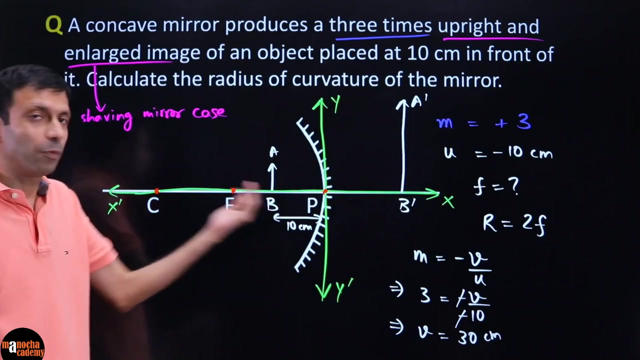 please take the lcm. lcm is 30, so 1 minus 3. so what are we getting? focal length: we are getting minus 15 centimeters. does that make sense? because for a concave mirror, focal length should be negative. it should be along the negative x axis. so see, you can check. 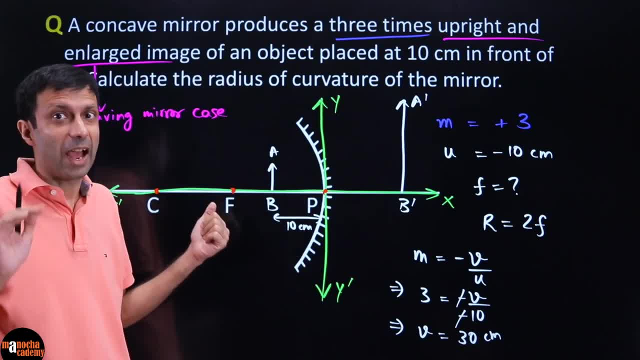 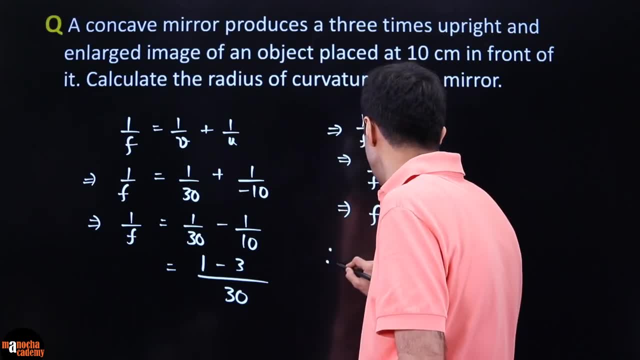 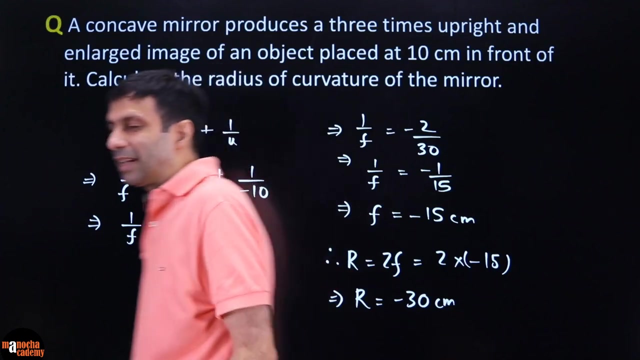 is your answer making sense according to sign convention? absolutely. so what is going to be the radius of curvature? very simple, therefore, we can say: r is 2f, 2 times minus 15. so therefore r is going to be minus 30 centimeters. so you can end your answer with: the radius of curvature, therefore, is 30, because you can 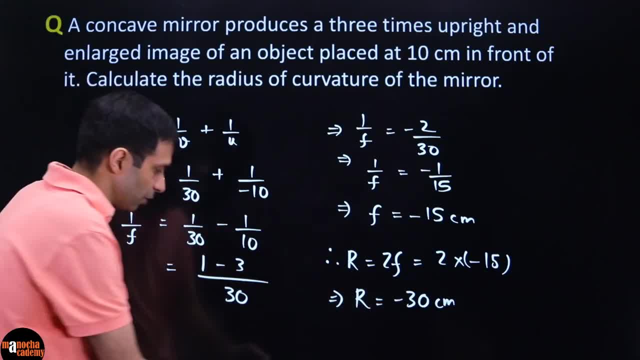 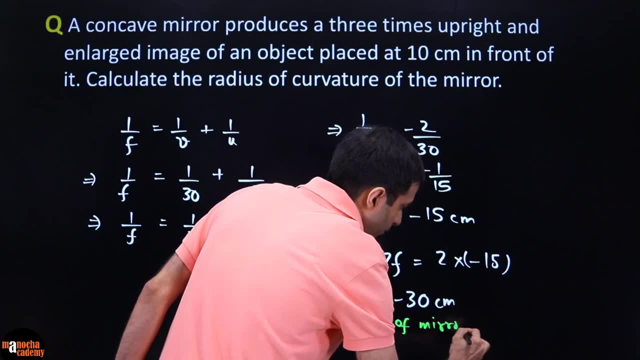 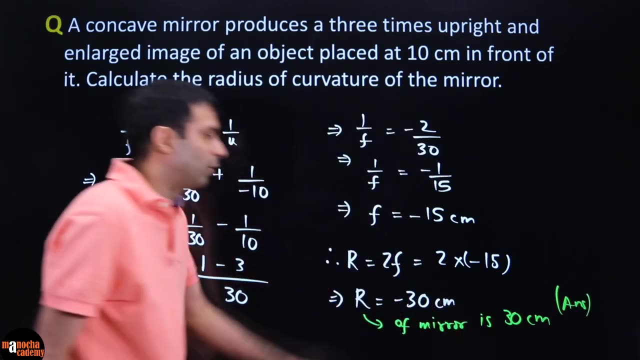 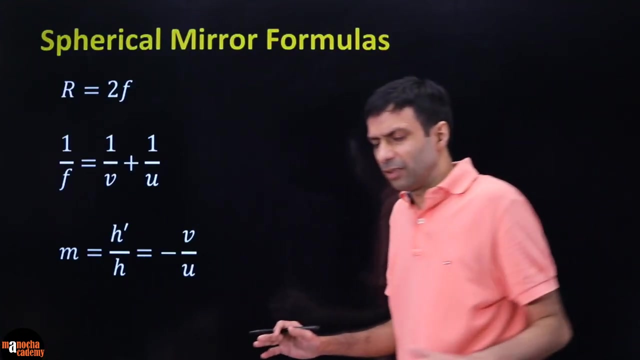 give both the numerical answer with the sign and then the written answer. so therefore we can say: radius of curvature of mirror is 30 centimeters. so i would say to give both the answers, the numerical answer with the sign and then the written answer as well. so that's it, the 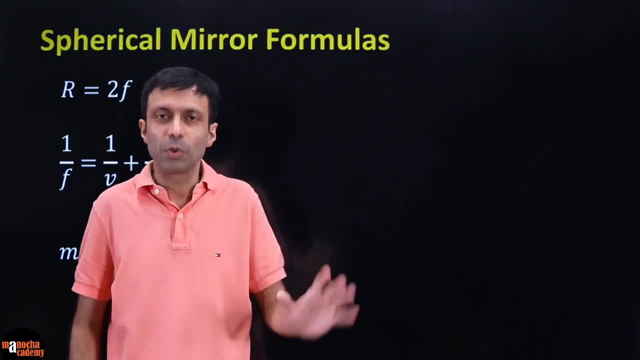 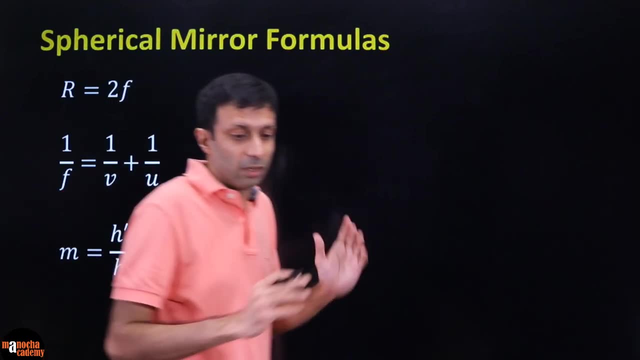 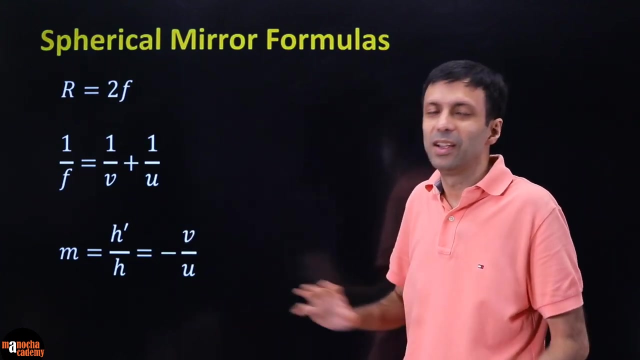 the trick was: draw a rough diagram. visualize the question. please draw that sign: convention axis, positive, negative axis. write down the formulas clearly, sorry. write down the data with the correct sign and then just use your formulas and please learn these formulas. write them down and it's super easy. after that it's just solving it. 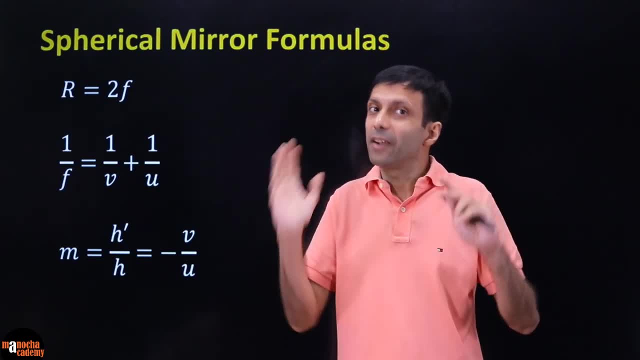 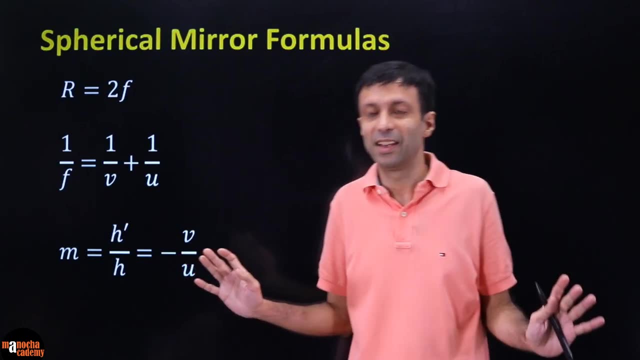 so, once again, draw a rough diagram with sign convention, write down the data with the sign convention, keep asking yourself: positive or negative? if its unknown, you just leave it as is, don't need to think about the sign. and then you saw that we were doing some common sense there. we were checking: okay, does this? should the focal length turn? 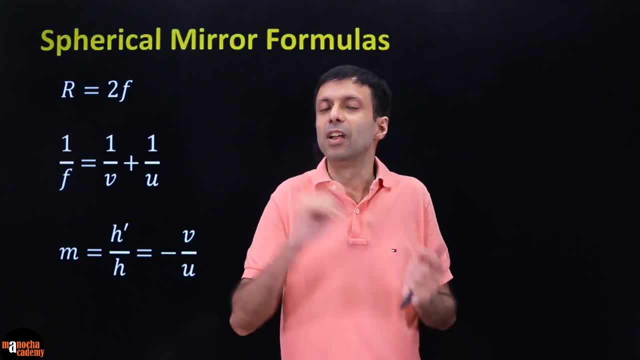 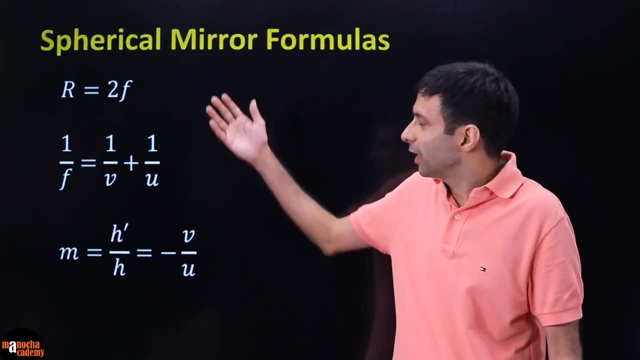 out to be positive or should the- you know image distance be positive or negative? you should definitely check that while solving so, even without you know, checking the numerical, just the sign. so sign convention is super important and all these formulas have to be used with sign convention. so hope you. 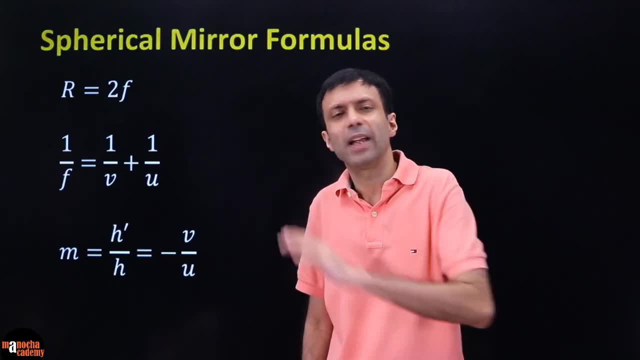 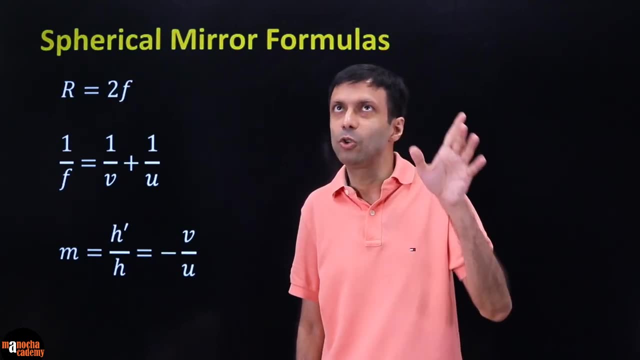 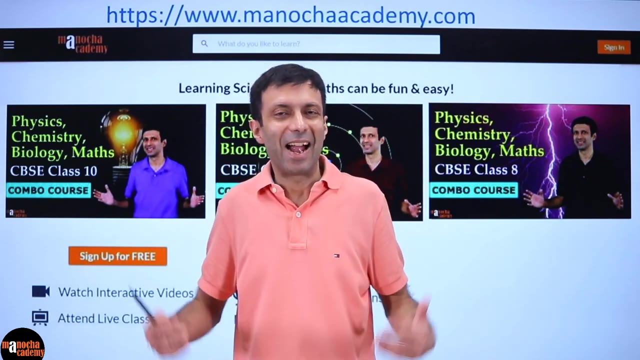 guys enjoyed this class and if you follow this technique I'm sure you'll get all these sums right. so please practice and use this technique okay. do not do shortcuts, do not do mental sums or directly jump to formulas. then you are inviting trouble. so hope you guys enjoyed it and please practice more. 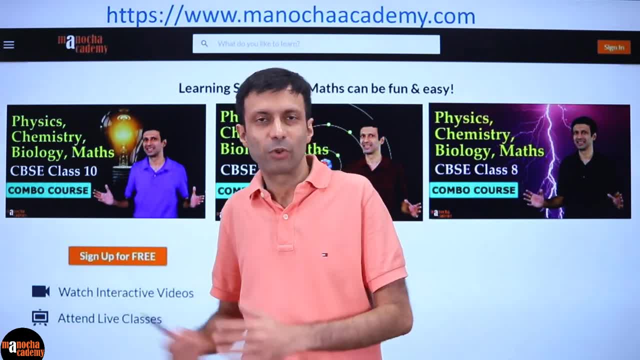 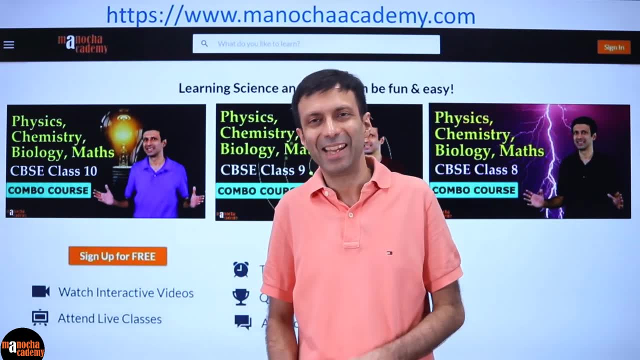 questions? we will. we have questions on our website. you have questions in the book as well, and do check out the other courses on our website. we are physics, chemistry, biology and maths for CVS e, class eight, nine and ten for the ICC students also, we have these courses.